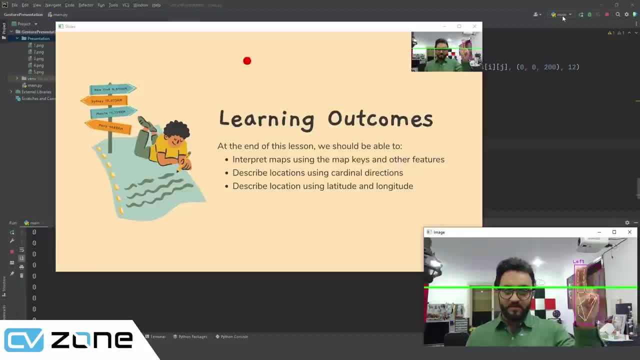 are the learning outcomes. I can delete, And then I can show the points And then I can draw a line, for example. And all of these things. they do not affect if you are using your hands normally. So you can see, here I'm using my hands normally. 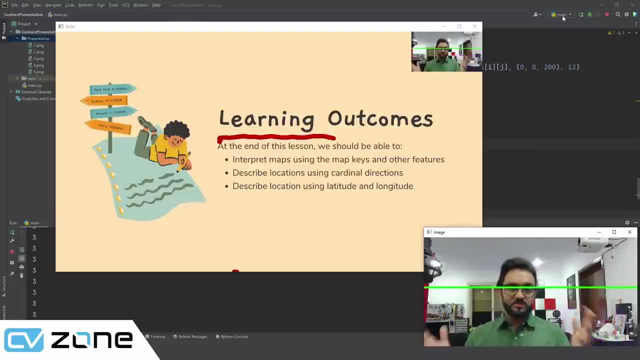 I'm moving around and nothing happens on the screen. So this is perfect for actually giving real presentations, So you can use this out of the box and give your own presentation like this. And not only that, I will also show you how to create a good presentation. 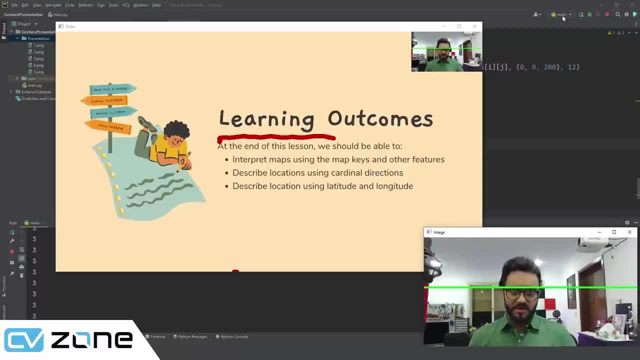 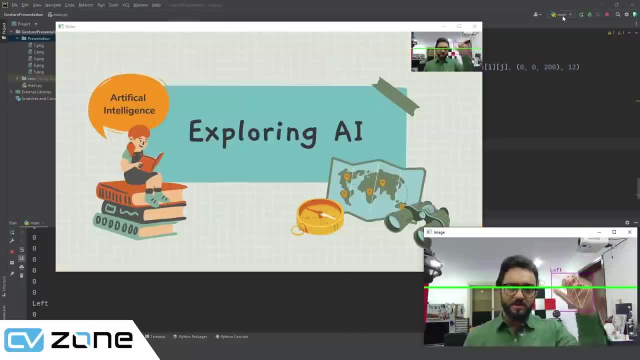 using an online tool which is free, And that's how I created this. I can go back and forth- And all these files- they are also available on our website to download, But you can create your own files as well, So this is a very exciting project. 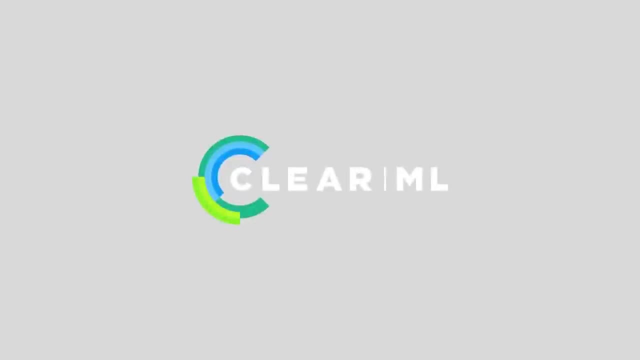 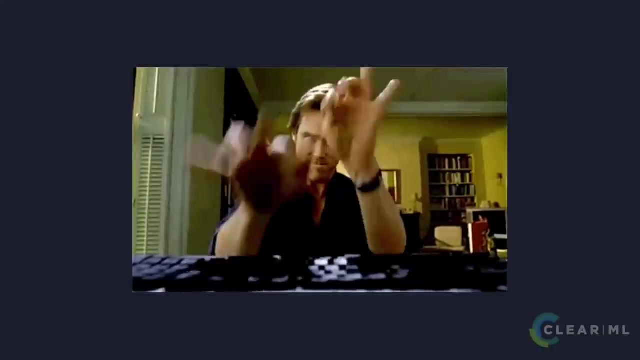 So stay tuned. This video is sponsored by ClearML. Do you want to know how machine learning and computer vision are done in the industry? Well, we all love running experiments and notebooks to learn really fast, But when solving problems in the real world, things tend to. 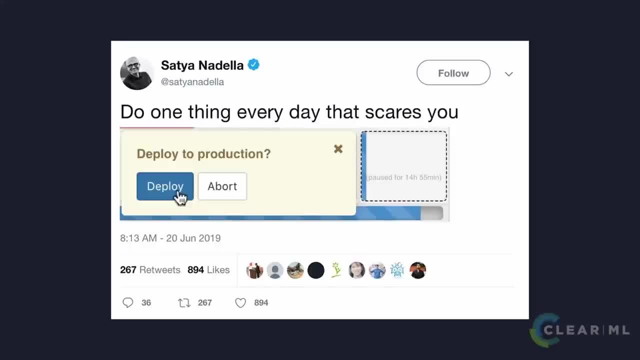 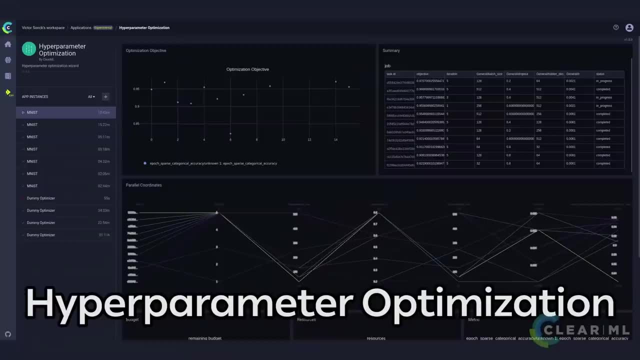 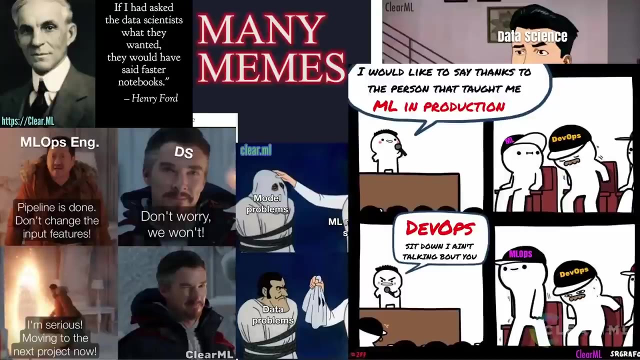 get really complicated, But that just means there's more to learn. ClearML, an open source toolbox, will help you bridge the gap between learning and actually deploying your projects in a way that's scalable to thousands of users, If you love machine learning and are looking to make real impact with your skills. 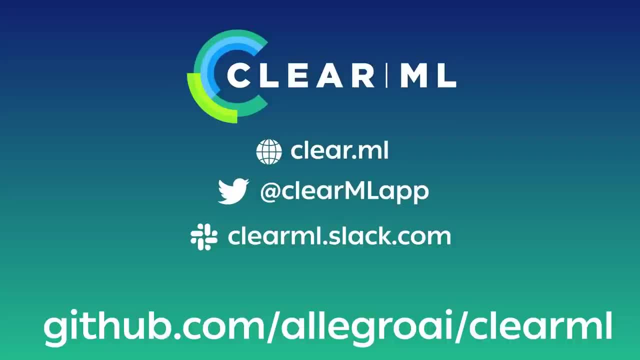 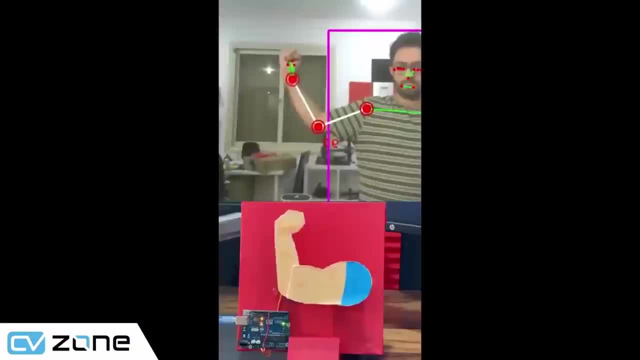 you can get started for free in 10 minutes. Check out ClearML and let them help you take your projects to the next level. If you would like to level up your computer vision skills, do check out our premium courses that are available on our CVZone platform. Links are in the description. 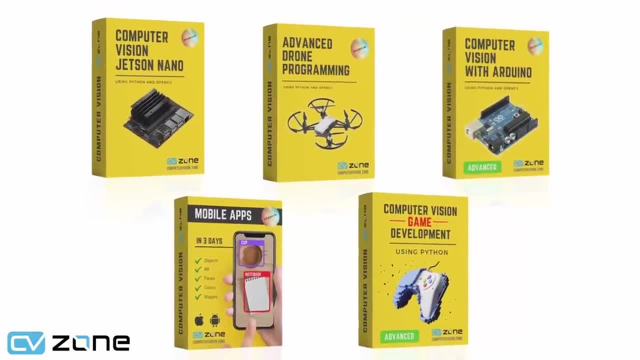 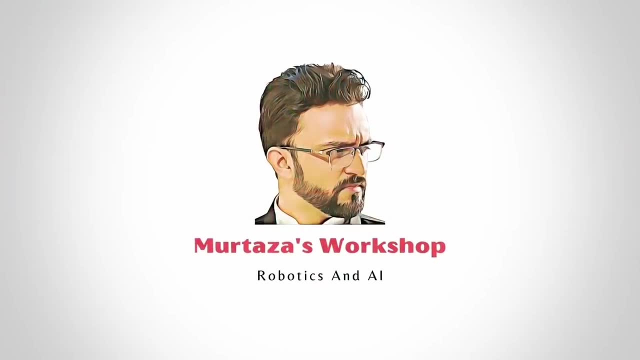 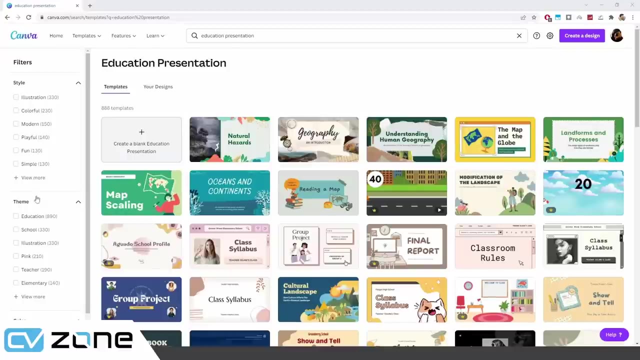 So, without further ado, let's get started. So the first thing we'll do is to start off by creating our presentation, So it's very easy to do that. You can head on to canvacom, and this is a free tool that you can use. 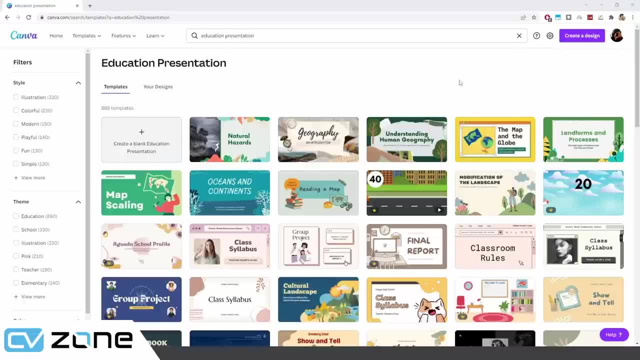 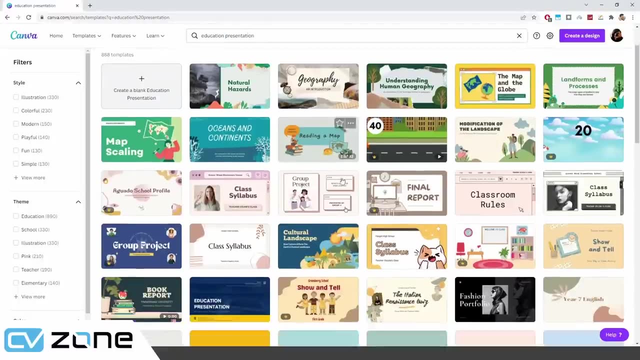 Of course, there is a paid version as well, But here you will find lots of free templates that you can use and you can add your text and animations and all that, And that will be quite useful. So what you can do is you can write here: education, presentation, And then these are the. 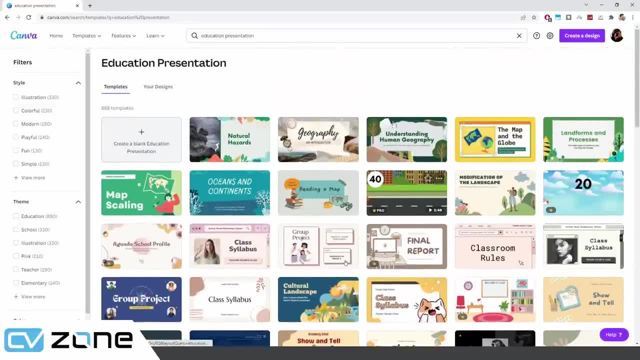 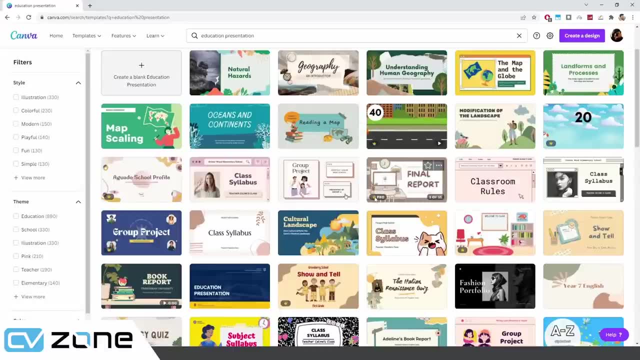 templates that you can see. So here you can see final reports, natural hazards, geography, whatever you want you can select. So again, there are pro versions and they are free. So let's pick a free version so that everyone can use. 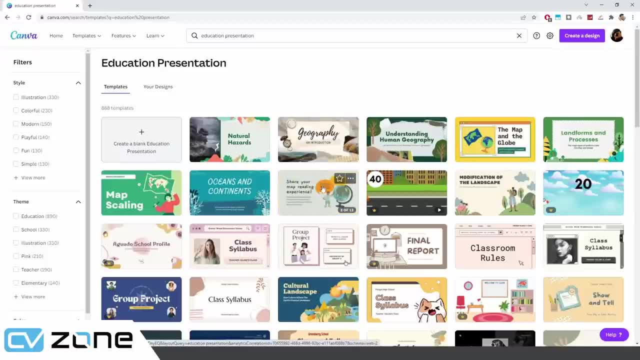 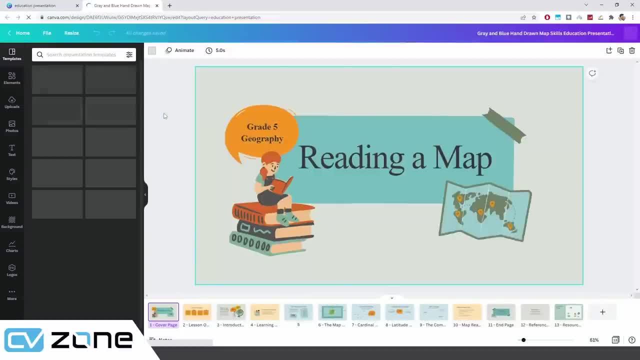 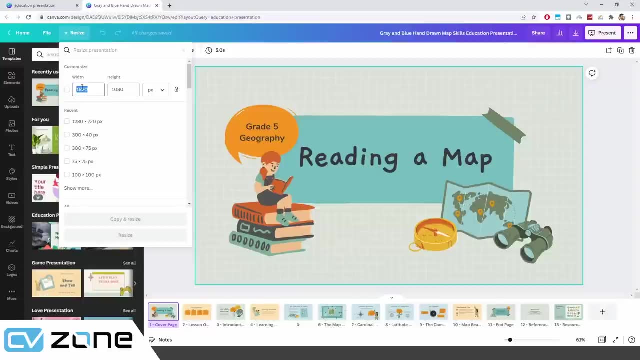 So, for example, here we have reading a map. This one seems free and it seems good, So let's click on that and it will open it up in a new window. We will resize this to: this is right now. it's full HD, so it's 920 by 1080.. What we will do is we will 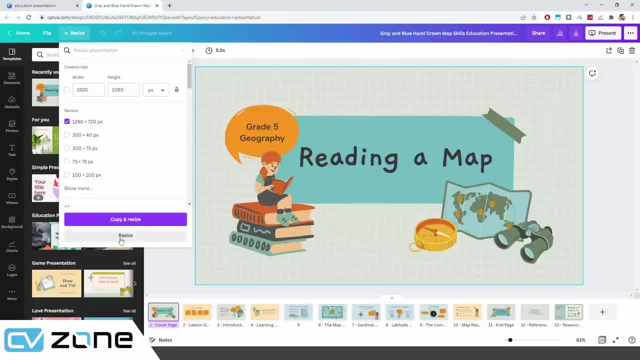 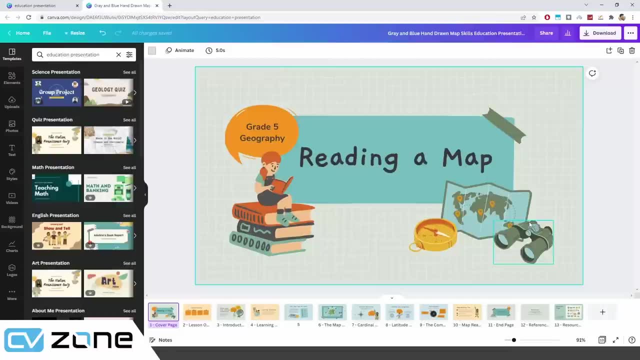 change it to 1280 by 720 pixels, So we will resize this so that we can export it in this format. Now, Normally, if you're presenting, you probably would want full screen, So you can go ahead with 1080p as well. 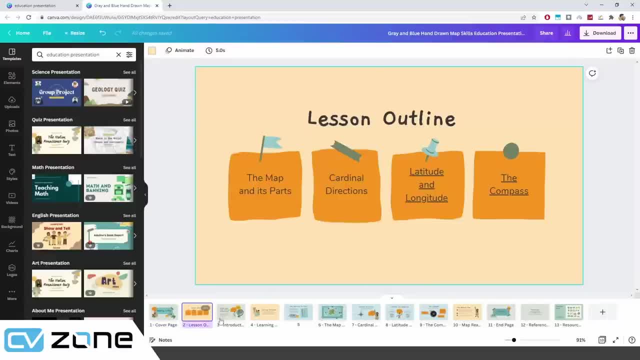 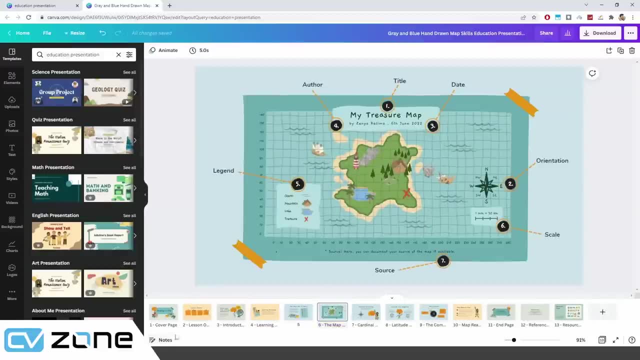 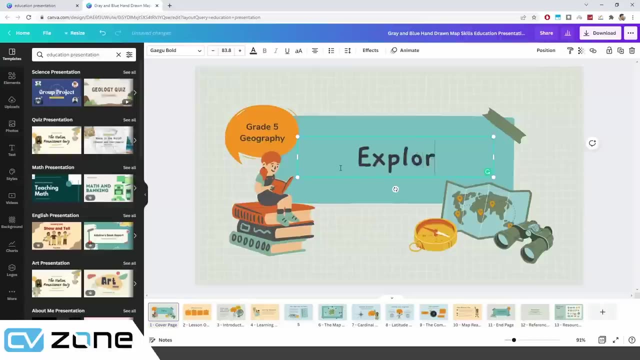 So full HD resolution. So here you can see, we have all these different designs and it looks quite good. So what we can do is, if we wanted to change, we can change things over here. For example, we can say exploring AI. let's say: 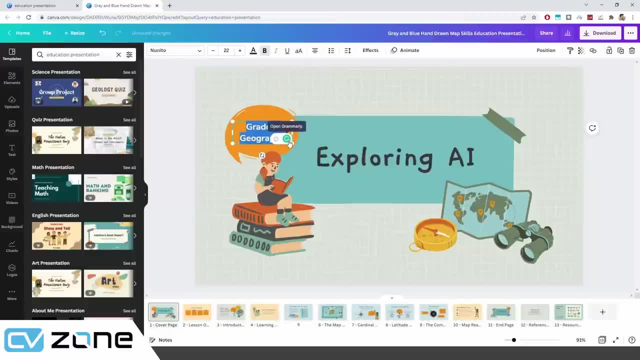 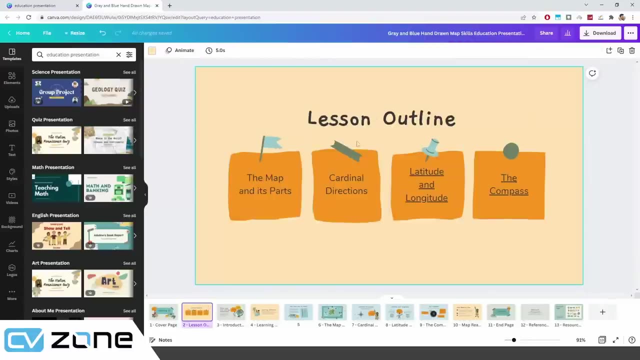 Okay, and let's just remove a grade five. Let's just say artificial intelligence, So exploring AI, and then we will go on to the next slide. These are the lesson outlined, So the map and its parts. let's say we will first start with the basics. 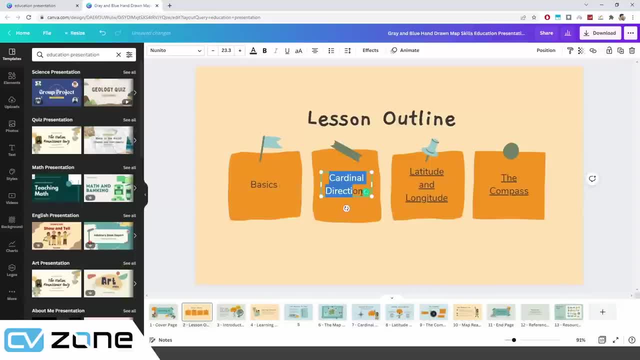 And then we will move on To, let's say, machine learning, and then we will move on to deep learning, and then we will go ahead and implement. So we will write here implementation, so we can resize this so that it fits maybe a little bit smaller. 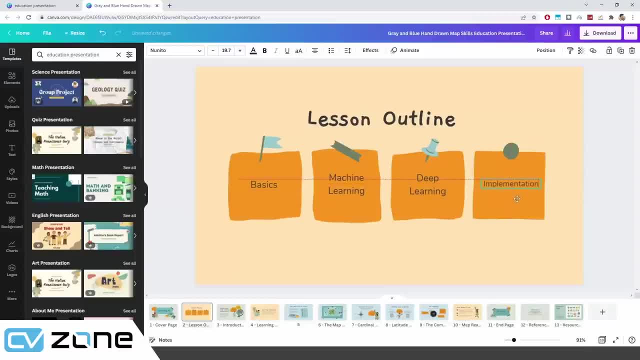 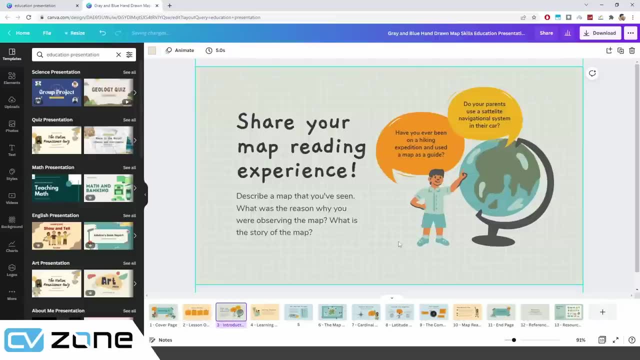 There you go, Okay, so I believe you get the idea. You can play around with this and you can create your own presentation- Most of the things that are already available- and all you have to do is you have to change these images and text based on your requirement. 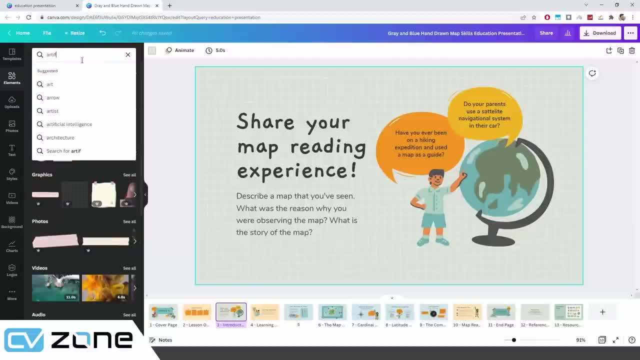 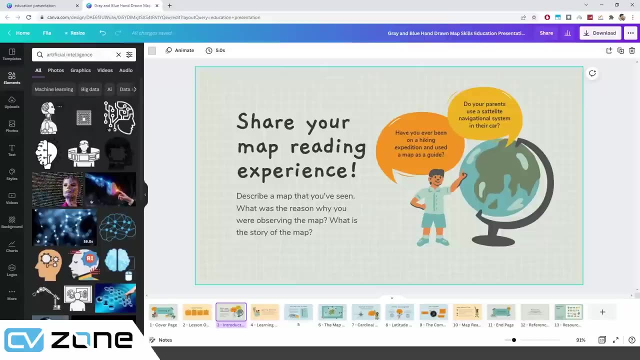 You can go to elements and, for example, here I can write: artificial intelligence. What is the problem? Artificial intelligence? And here you go, You have these images. So again, you can use the free ones if you are not using the paid version. 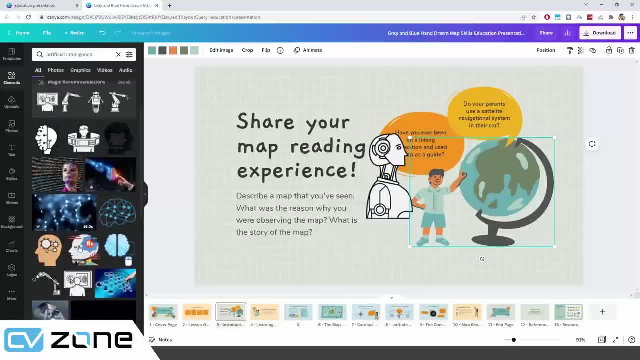 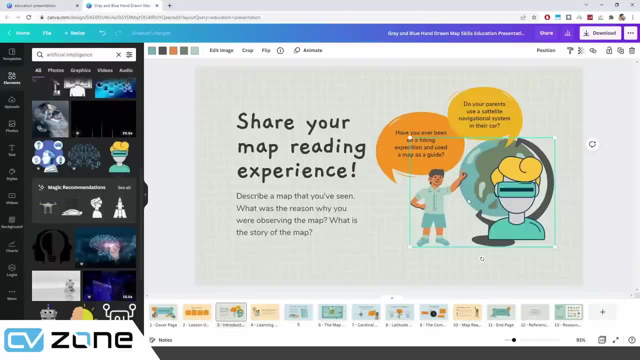 So, for example, or let's pick something that is similar to this, Maybe this: Yeah, I think this is a good replacement. So if we remove this image and we just paste this one here and send this to the back, Yeah, maybe not that back position. 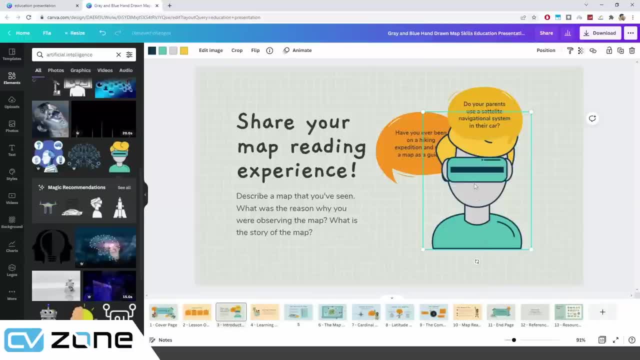 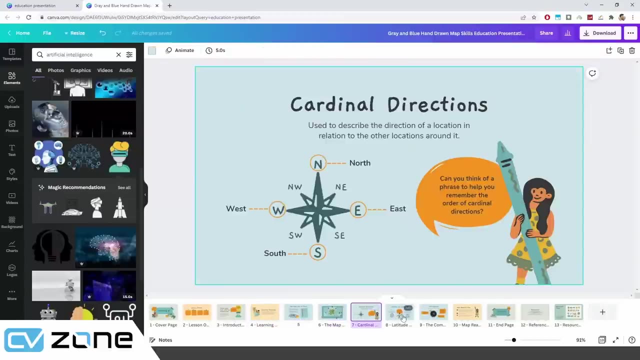 No, This is the position for this. send backward, send backward. There you go. So maybe we can do something like that And then we can change the text over here and all that. Then again you can play around with all these what do you call files, and you can create your presentation. 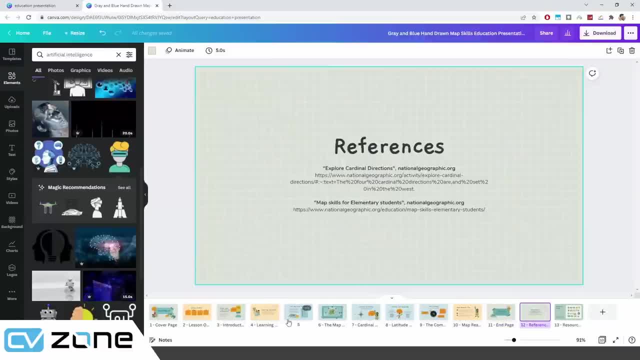 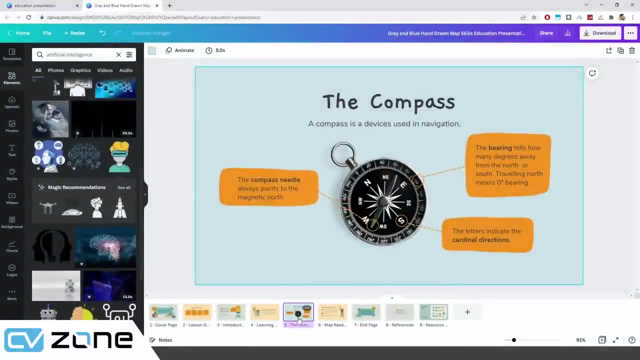 I think there's a lot of them over here. What we can do is we can remove a few of them, So we will try to keep it simple. Yeah, we will keep. let's say how many pages are there. Let's say we'll keep five pages. 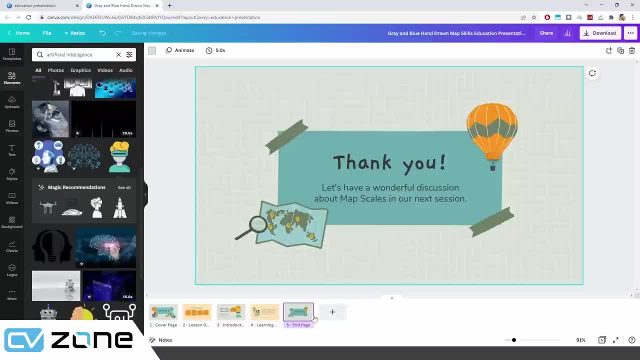 So this is thank you And we don't need the resources pages. So here we have these five pages and we are going to use this Now. one important thing here is that these pages should have numbers. So this is one, two, three, four, five. 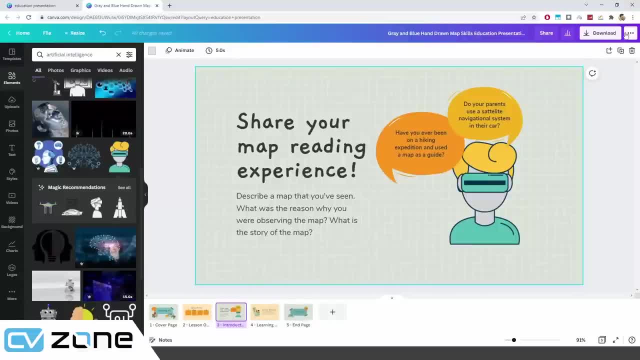 So we need to make sure they have these numbers so that when you download them, they are going to be Are already sorted, so we don't have to sort them, Okay. So let's download this and we will download it in PNG formats. 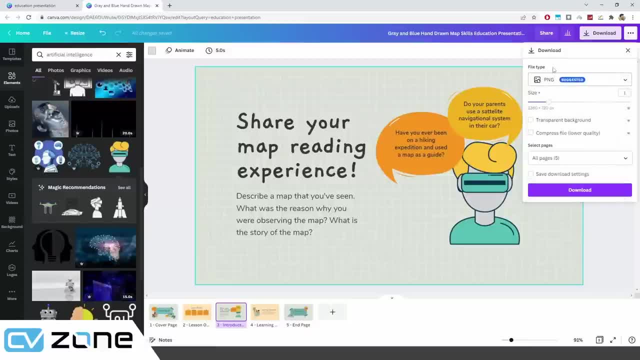 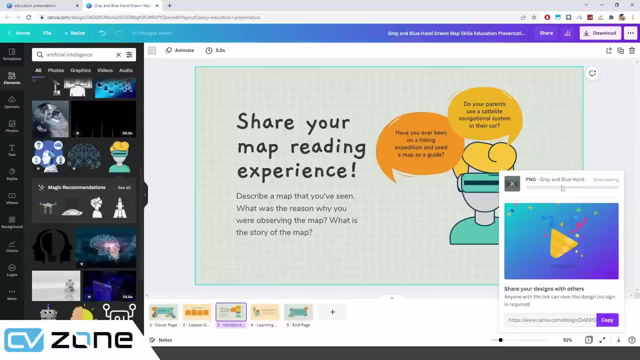 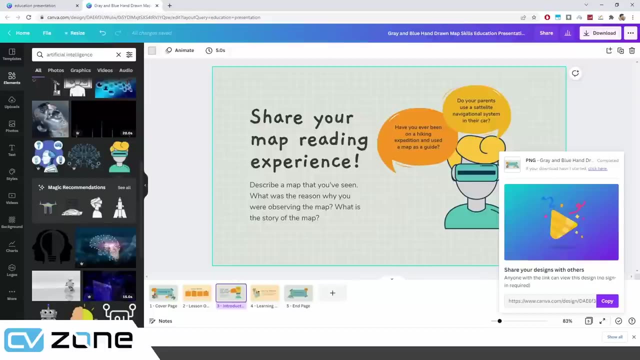 PNG will be a little bit clearer than JPG, so it's better to download it PNG. And yeah, so we can simply hit download and it will download a zip file, And from this zip file we will have all these five images. So let's open that up. 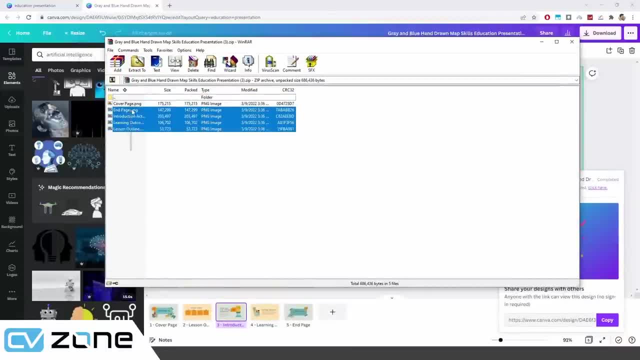 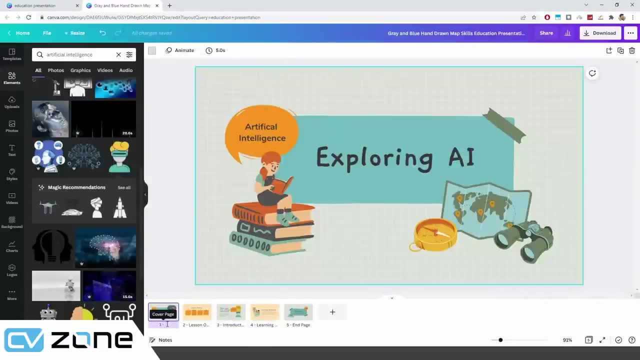 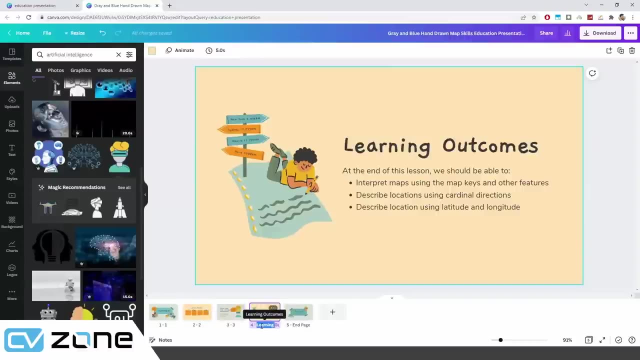 There you go. So we have these five images, but here you can see the numbering is not there. So that's not good. So let's just go back here and we will change the name to one, two, three, four and five. 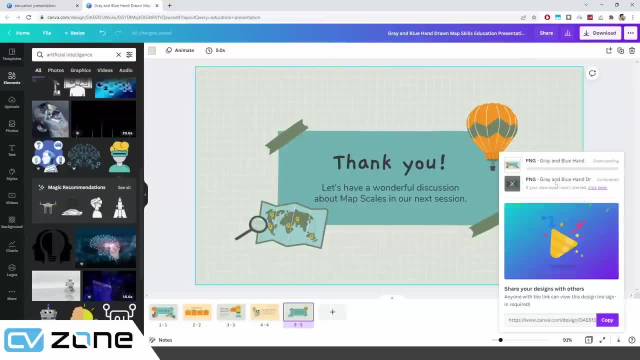 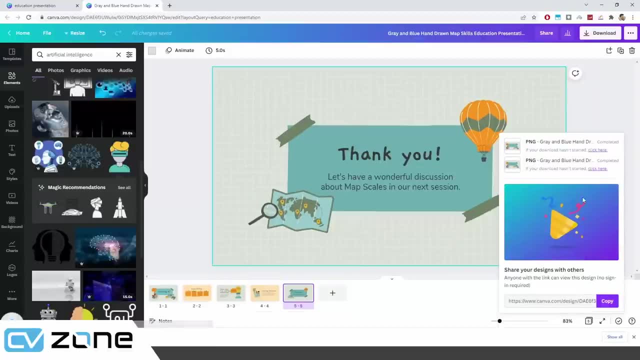 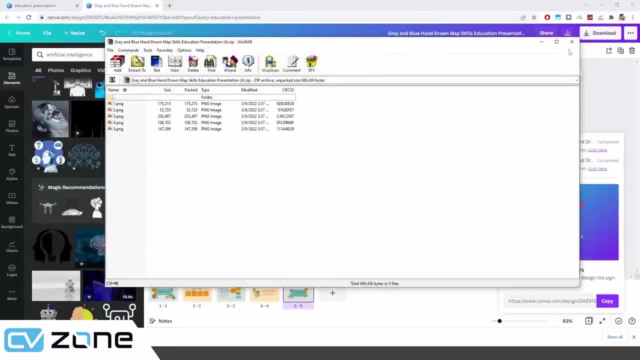 So let's download that again. There you go. So now we have all the images in the correct order so we can take this to our PyCharm project. So let's go ahead and do that, Okay, So Okay, Okay. 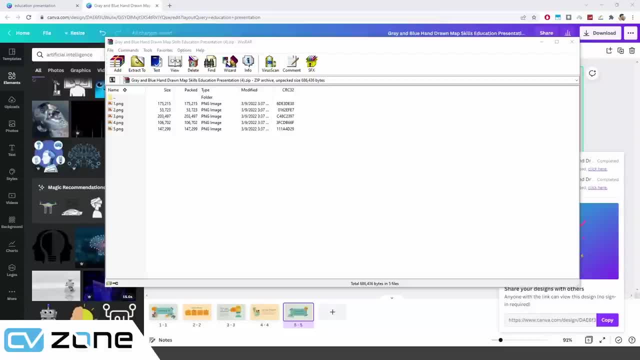 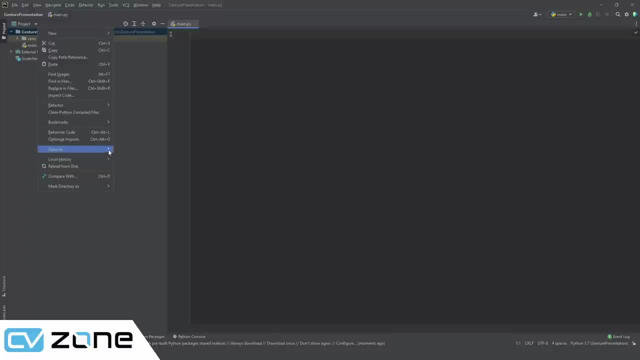 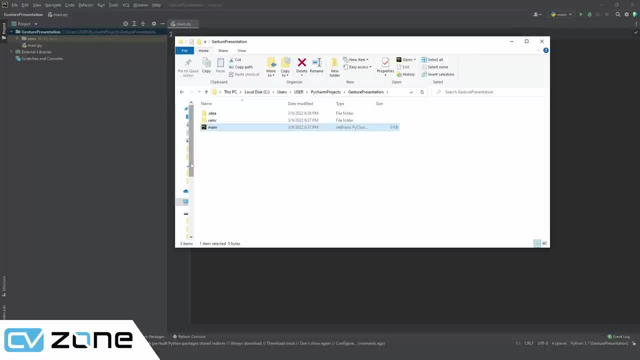 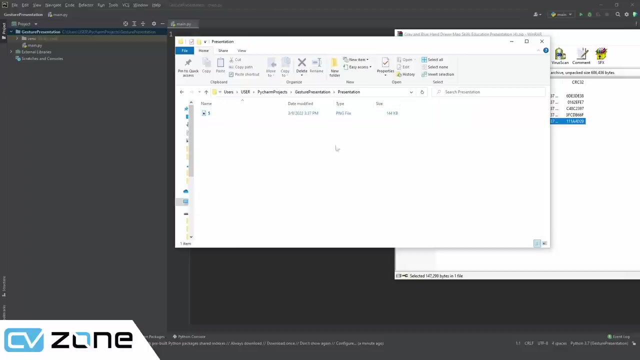 to add all these images, the ones that we downloaded, but before that we will create a new folder. We will call it presentation. no spelling, wrong presentation. Okay, Okay, Okay, Okay, drag. so simply dragging and dropping. so we will drag and drop. something is wrong. 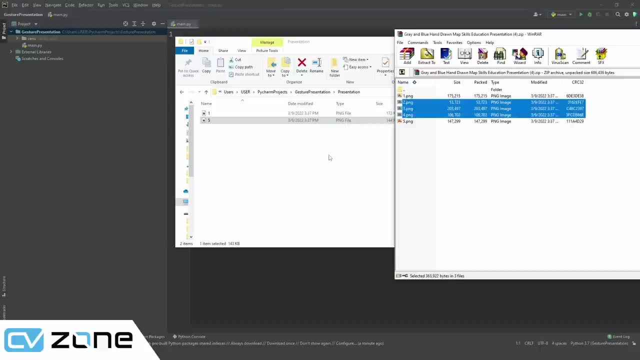 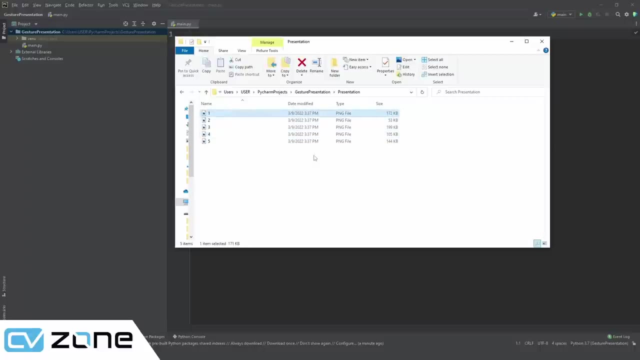 it's not selecting all of them. I don't know something is wrong here, but let's just drag one by one or we can extract. but these are just five images, so not a big deal. so we have these images now let's just zoom in and see if they are. 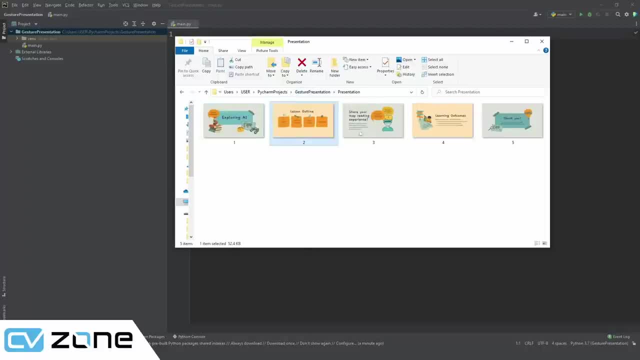 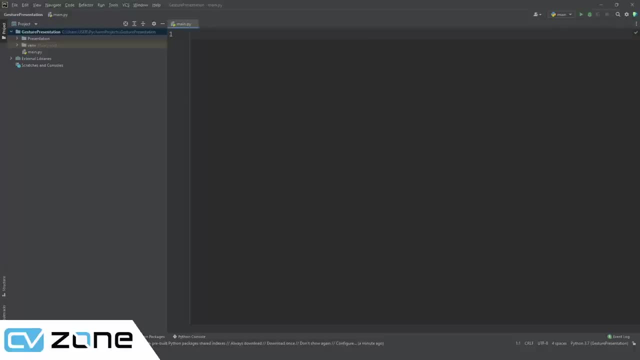 there. there you go, and they are in sequence. so that's good. so now we will close this and we will go to our main file. now, the first thing we have to do after we add our presentation files, we are going to go to settings and then we 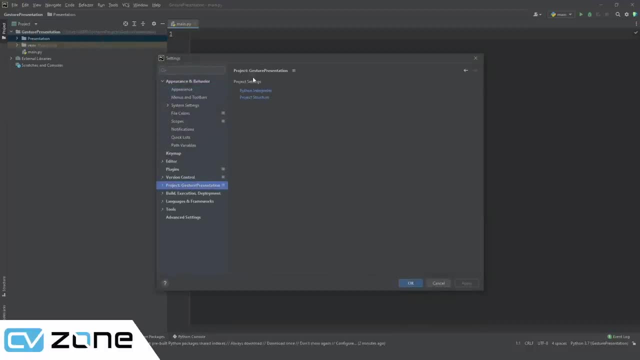 are going to install the packages that we require. so we'll go to project Python interpreter and we are going to add the interpreter. actually, it's already there. if it's not there, you can see that it's already there. so you can see that it's already there. so 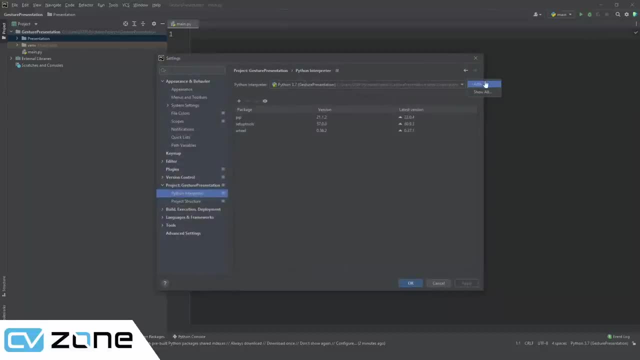 we can see that it's already there, so we can click on this and then you can add it from here. so here we will click on add and then we will write CV zone. we are going to install that, and what else do we need? we need media pipe because we 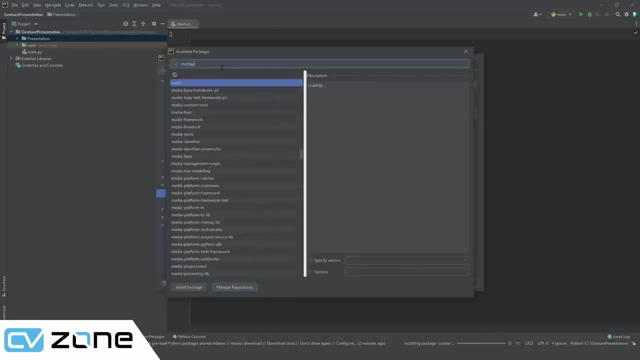 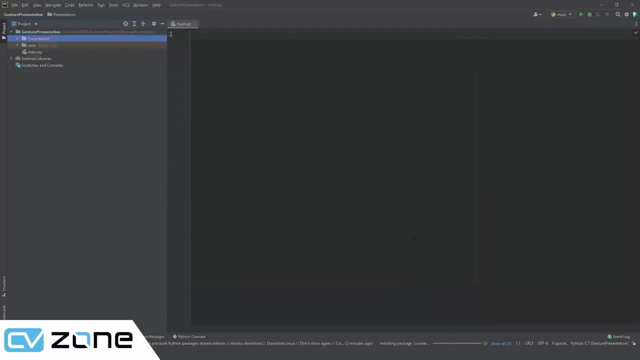 are using the hand detection media pipe and when you install CVs own, it will also install OpenCV and it will also install NumPy. so we will be using those, but we don't have to install them separately, because they come uh with defaults, uh with cb zone, okay, so now it is installing, so we are going to wait. 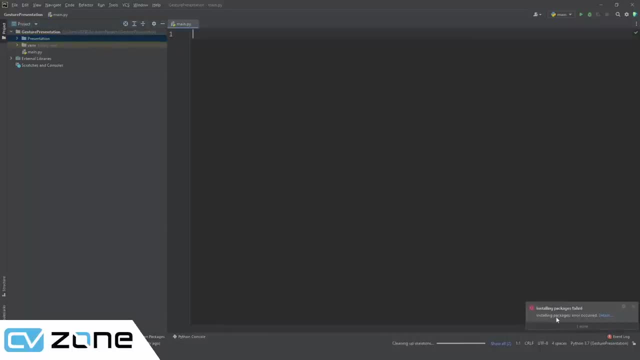 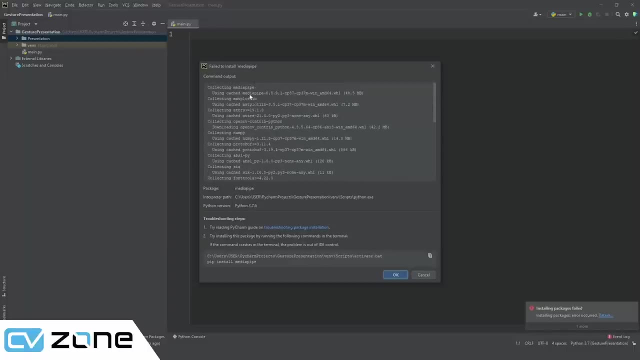 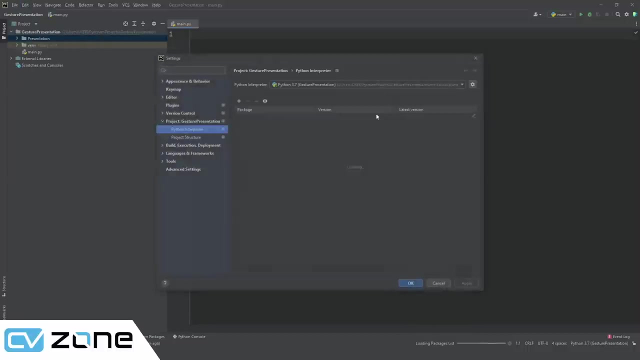 for it to complete installing. so one of the packages was installed. the other one gave an error. let's see what that is. uh, it is of media pipe. not sure why that is. let's just close that. go to file settings, add media pipe and we will install it again. 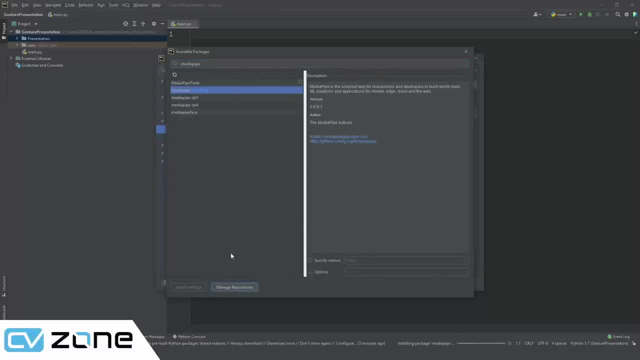 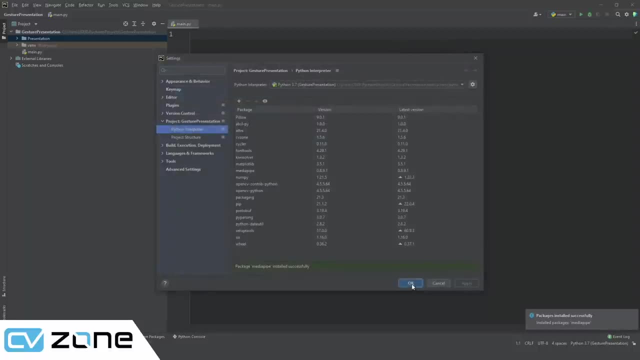 okay, there you go. so now it is installed. so let's just close that. and now what we will do is we will first of all import our packages. so we will start off by opening our webcam so that we know everything is running smoothly, and from there onwards we 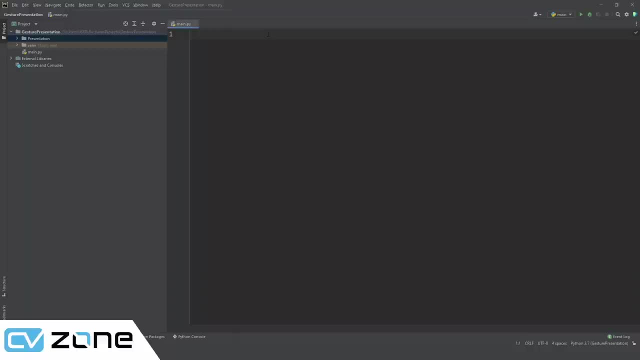 are going to add our presentation files, then we will look into the hand detection, then we will look into the drawing and the gestures and all that. so let's start with the webcam. so we will import cb2 and then what do we need? yeah, that's pretty much it, and then we are going to create. 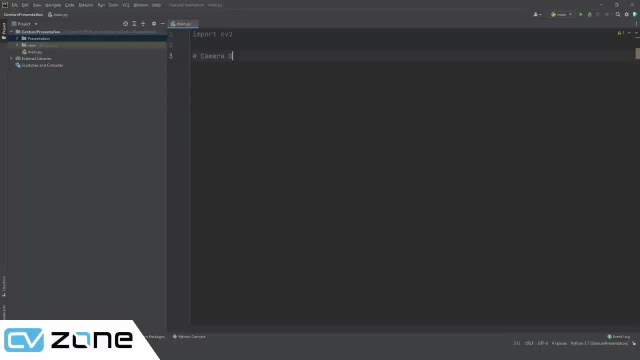 our camera object. so let's just write here: camera setup. and here we are going to write: cap equals cb2, cb2, cb2, dot video capture and we will give in the id number, which is zero. then we need to give in the width and the height. so let's write here: cap, dot set and number id. 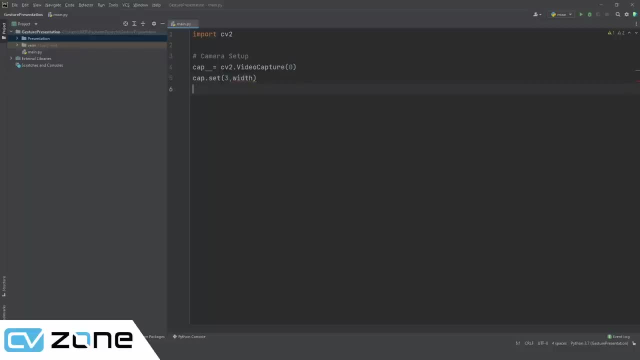 number three is the width, so let's write here width and the gap dot set id. number four is the height. so we didn't define width and height, so let's define them here variable variables, and we will call them width and the height equals one, two, eight zero by 720, so we are: 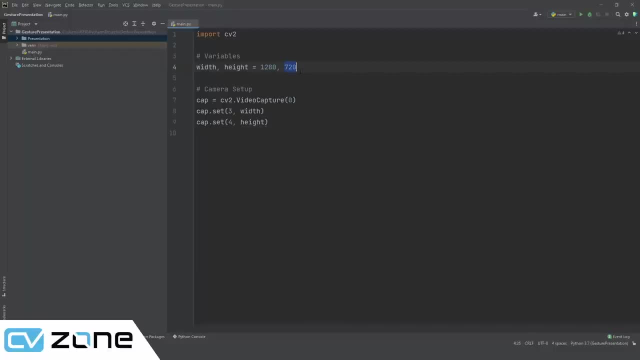 going to use these later on as well. that's why we are putting in putting them in variables, so we can use them later on as well. so, once that is done- uh, what happened there? once that is done, we are going to write the while loop. so, while true, we are going to check the success and the 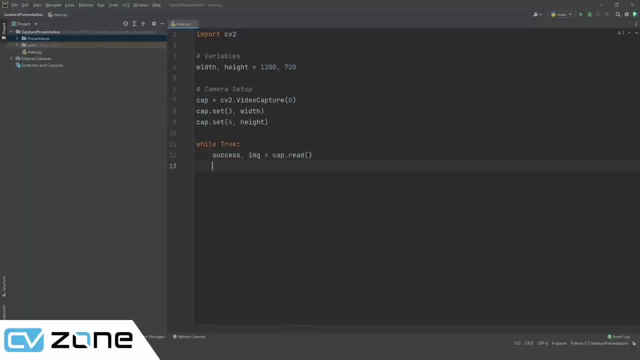 change value and we're going to say that it's skulle is right as close to zero. even though maybe it is true previous time, we do have a new one. this time i had to make it smaller one and the selected to be the active object. soacula controlling function of evident the. 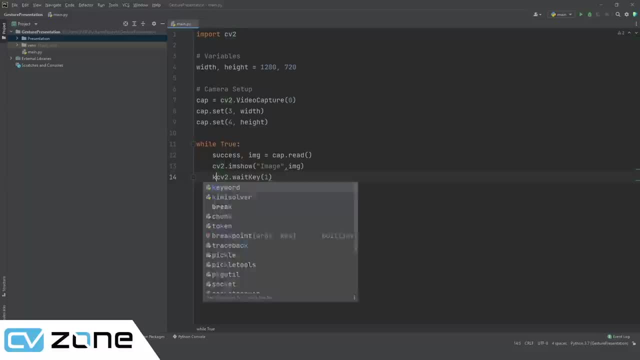 system will be set to the this in key and we will check if the key, if the key equals- or the Q, then we are going to write break. so it will break from the while loop if we press the Q button. so this will allow us to close it without pressing the cross button. 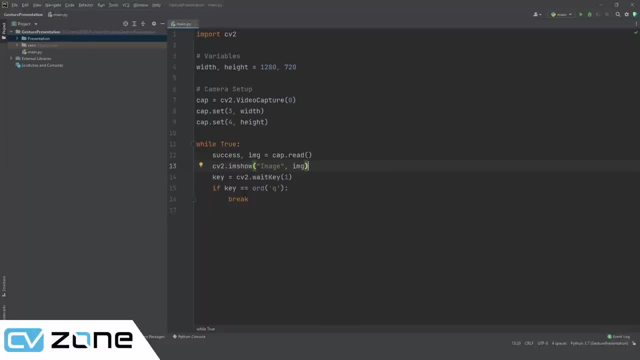 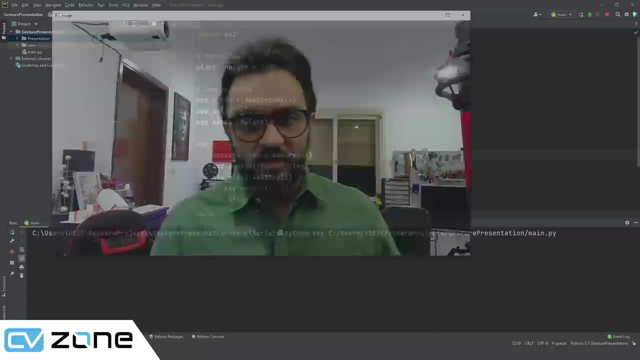 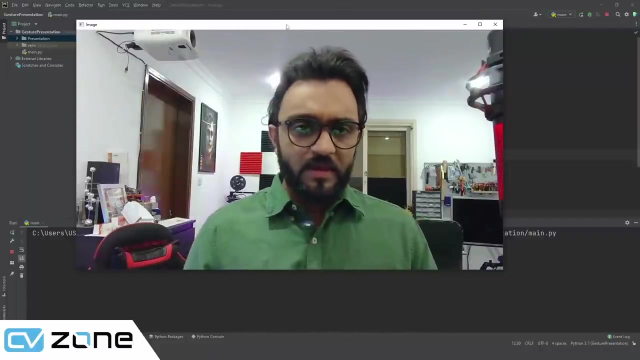 actually, if you press the cross button, it's not going to, it's not going to close because every frame it will keep every iteration, it will keep changing the frame. so right now I'm turning on the webcam and, as you can see, the webcam is turned on and you can see me around. there you go and we have everything. 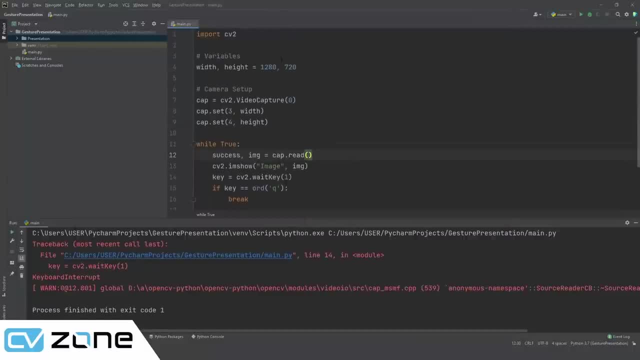 ready. so again, it's up to you. if you want bigger size, you can have it here. so this size, it doesn't have to be exactly the same as the presentation. so your, your webcam can be of different dimensions and your presentation can be of different dimensions. it doesn't matter what if they are saying: okay, so this is for. 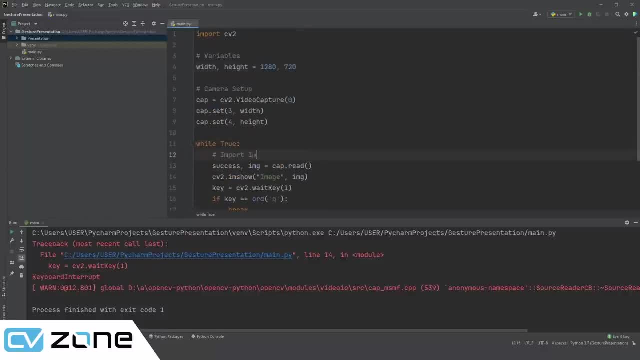 importing the images. so imports images. so what do we mean by images? we are going to import the presentation images as well over here. that's why we are writing importing images. so here what we will do is, first of all, we need to know all the names of these files. so whatever we have, we have to import. so 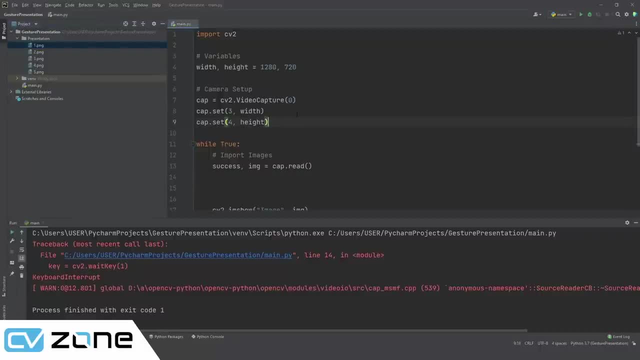 normally what you would do is you would, you would put all of these in a list and then you can just change their numbers when a gesture is being made. but the problem there is that if you draw something, it will remain on it. so we don't want that. we want to keep what do you call iterating these images. we won't. 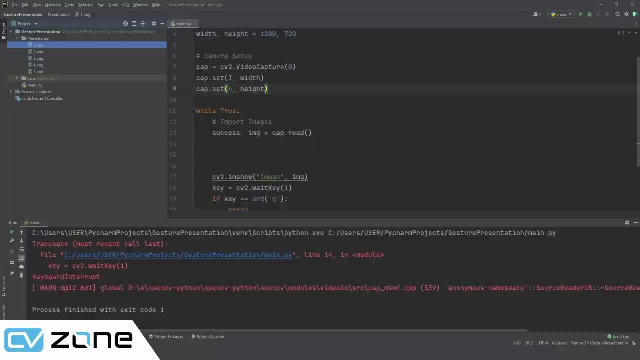 import on every iteration so that every time it's a new image and if we want we can draw on it. so it might be a little confusing at this point, but I will explain this further on as well. so the first thing we will do, we will get the. 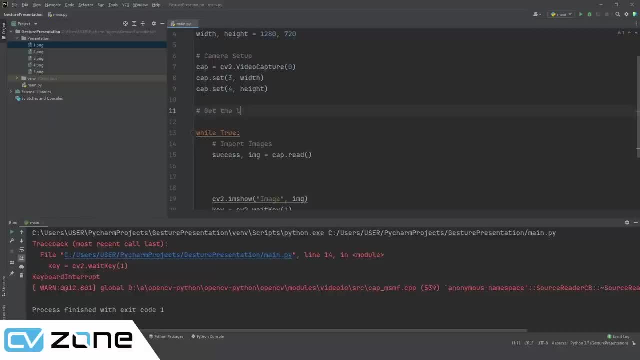 list of presentation images. so get the list of present presentation images. so let's call it path. images equals OS dot list directory and we will give in the folder path. so what is the folder path? let's just declare it here. folder path equals present presentation, so this is the name of the folder. so here we will. 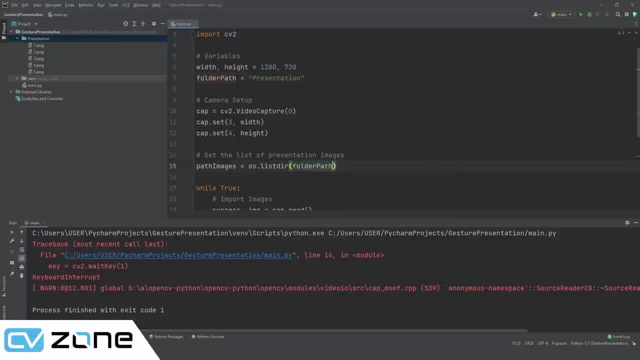 write folder paths, folder path and yeah, that's pretty much it. so actually is it? yeah, so for for the list: yeah, that is pretty much it, so let's run that. oh, actually we didn't print anything, so let's print the print the path images to see if we are getting it right. let's run. 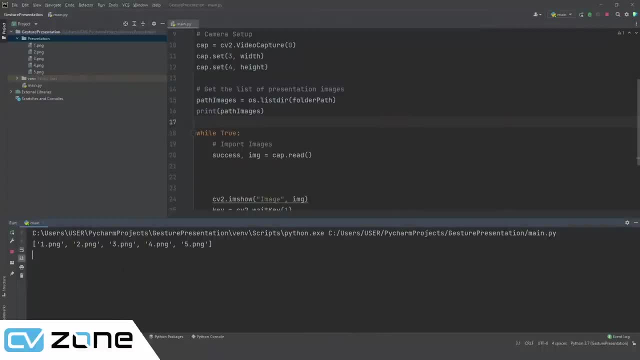 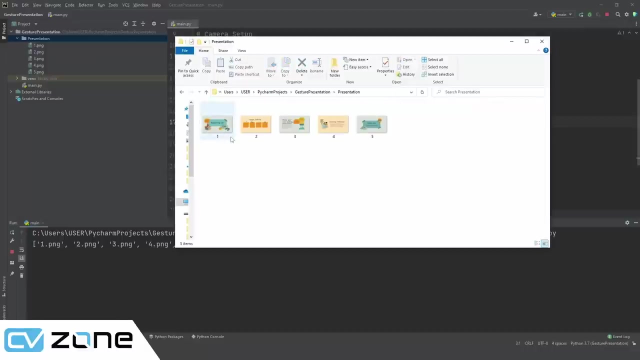 that. there you go. so now you can see. we have all the names. now. there is a very important thing to remember about this is that if you want to use the very specific problem that you can encounter- and let me explain how, how that works- so if you have more than nine presentations, so if you have ten files, 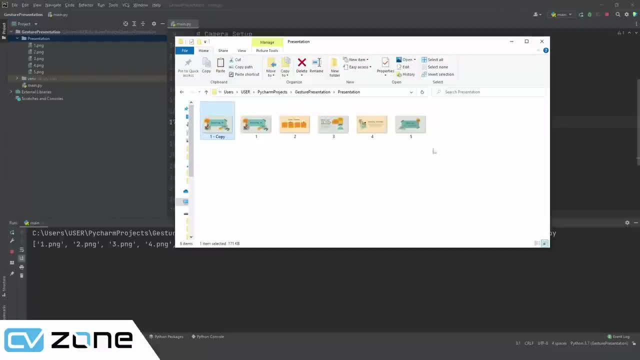 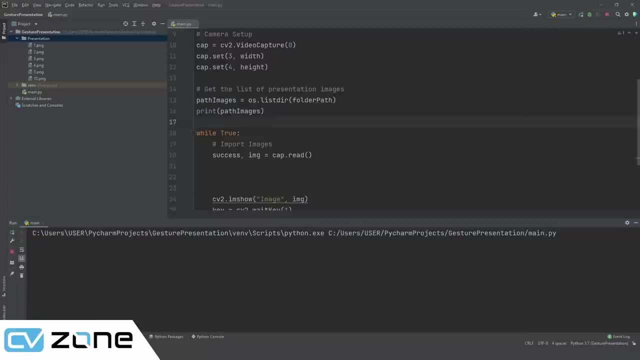 then the sorting will be wrong. so if I write here ten, so let's say after five, it should give you ten, right, but in this case it will give you ten after one. so let's just run that again. so there you go. so now you can see it is one, then it's 10, then 2, then 3, then 4 & 5, which does. 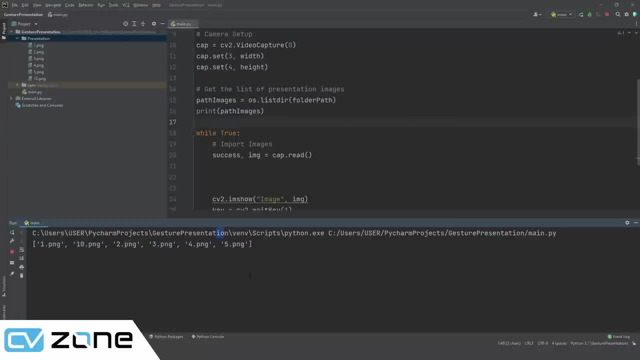 not make sense, right, so that if your tenth presentation is Thank You, it will just appear right after the first one. sorry, the slide. so what exactly can we do to sort this out? so what you can do is you can write here: sorted, sorted, and then you can sort based on length. so of course it will sort based on the 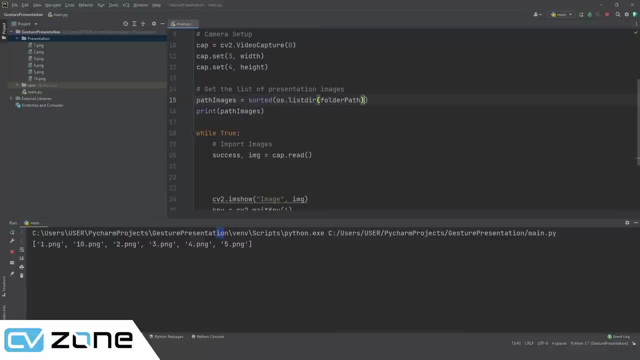 what I call numbers, but it will also sort based on the length. so key is length. so this time around 10 will now be at the end. there you go. so it's 1, 2, 3, 4, 5 and then 10. so I will keep it here like this, in case you have more than 10. 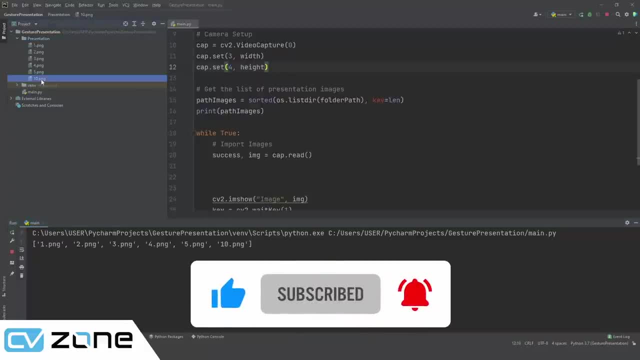 files. so, but I will remove the 10th one, okay, okay. so now that this is clear, now we need to import. so these are just names. we didn't really import any image, so what we need to do is we need to import. so here, first of all, we will. 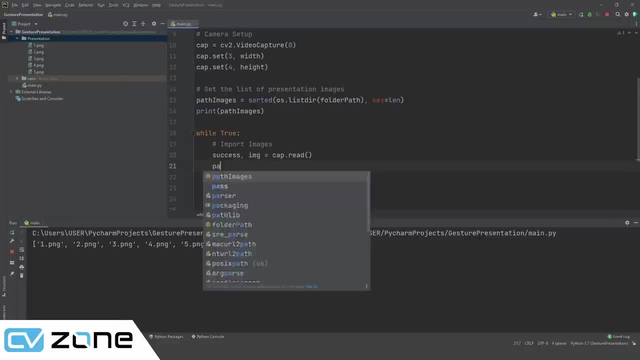 create the path name. so here we will write: let's call it path. full image equals OS, dot, path, dot. join. now you could literally create a string and join them. but if you use this function it will work in different platforms so it will be easier to work with. so here you can write: folder, folder, path you want to. 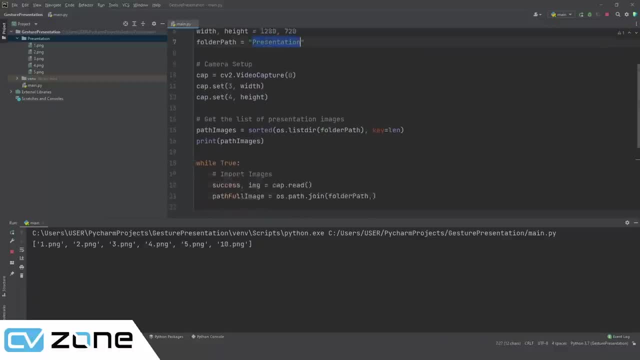 join this. it will save presentation slash the name of the image. so what is the name of the image? we will get it from here, from path images, so we will get the first one. so here we will write path images, number 0. so number 0 will give us this one, 1 dot png. so it will import the first one. 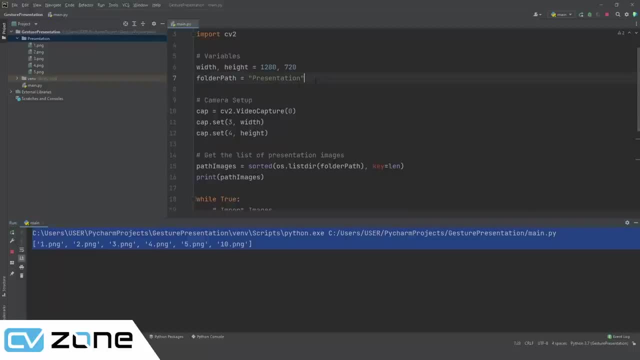 but in this case what we will do is we will make it a variable. so let's just write here variables and here- where is the spelling wrong? show context: very, oh, there's no a, my bad, okay, so then, uh, what were we doing? okay, yeah, we will write the image number. so here we will say that image number. 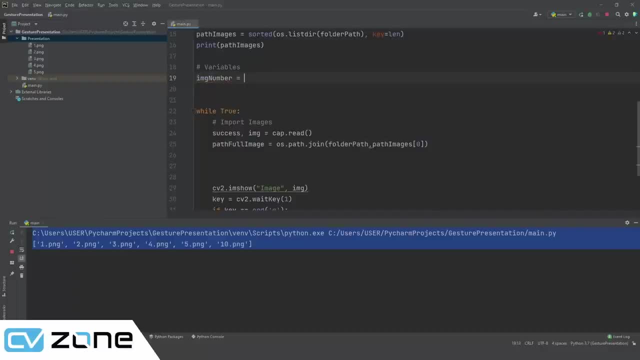 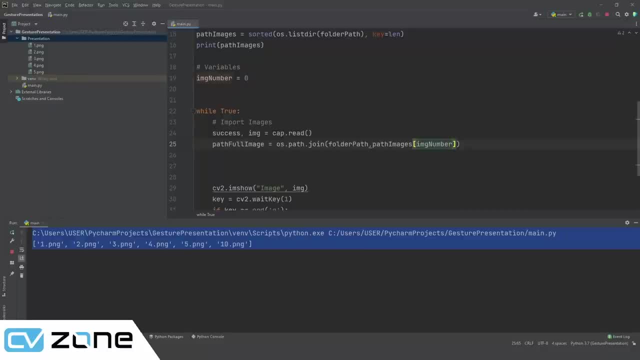 forth in our slide. so that's how simple it is. if I want to go to the next slide, I will change the image number to 2 and it will automatically change it to, let's say, the second slide. we will test it now. so here, once we have that, we will. 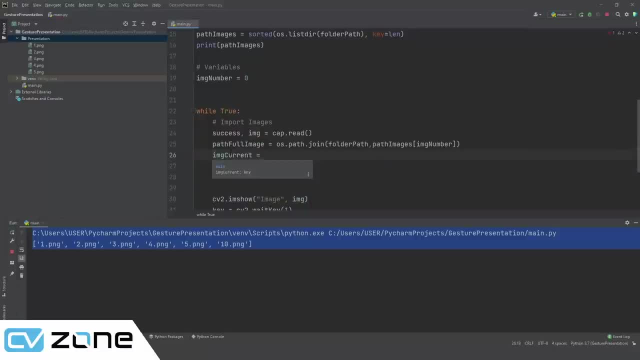 write image current equals or should we write slide? let's just write image current, so we will write cv2 dot. I am read and we want to read the path of the full image. so that's how simple it is and we need to display it. so here we will copy this and we will write here slides, slides or. 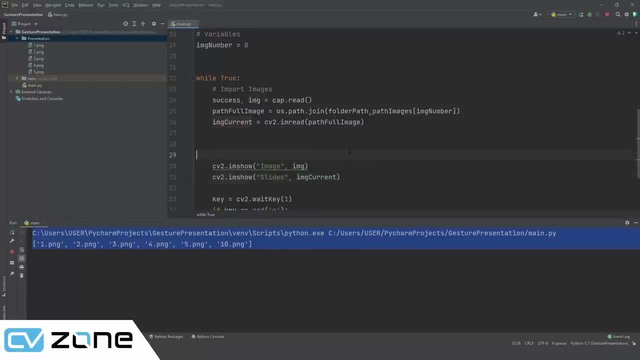 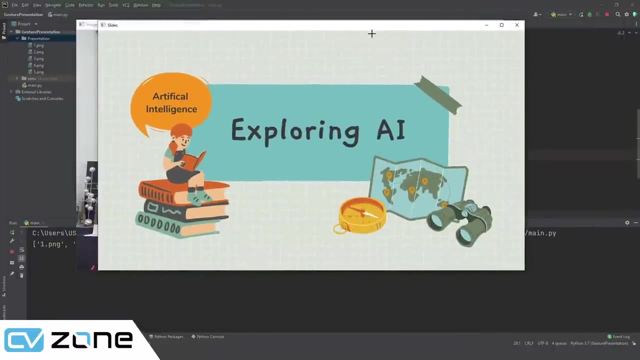 presentation, whatever you want to call it, and image current. so yeah, so let's run that and see how it works. so now we should have two images. there you go. so this is our presentation. it says exploring AI and yeah, it works. so this is the first image. now, if we wanted to, 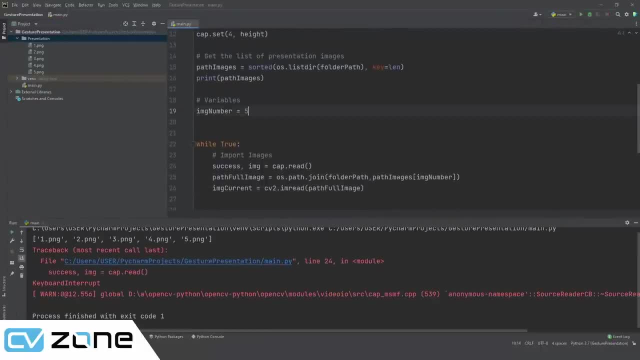 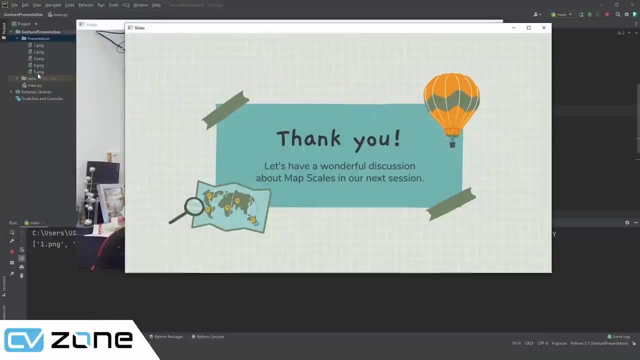 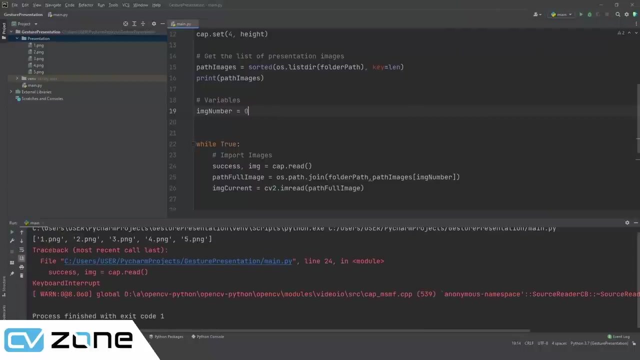 we can change the number here. let's say image number 4. okay, so this will be the last one, because we are using 0 as well. so it will be the fifth one which says thank you. there you go. so you can see how it easy it is for us to change the. 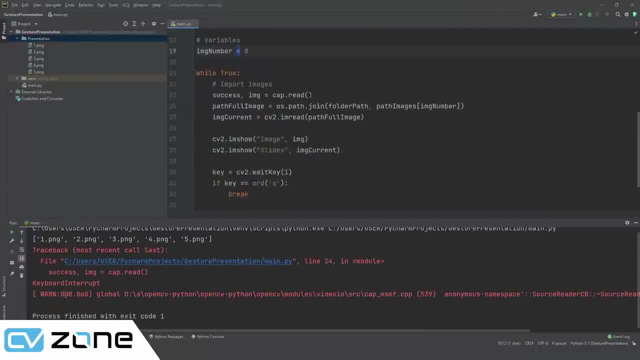 slide number. we just change the number here and it will change the slide. but how do we tell it? we will tell it based on some gestures, now, before we go there. we will tell it based on some gestures, now, before we go there. what we will do is we will add this, what you call display, or you can say the. 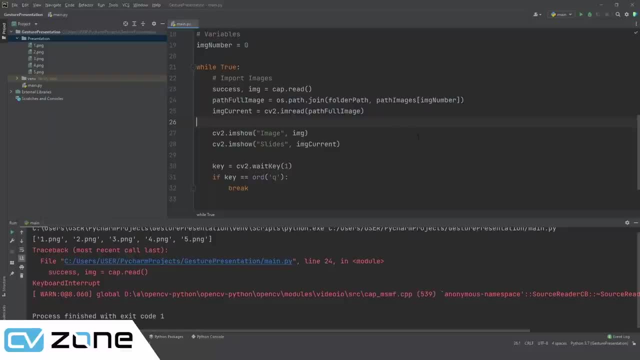 webcam image on our slide as well, because when you want to present, you don't want two different images. you just want to see what is happening a little bit on the side, just to make sure you are in the correct position and everything, but you don't want two different images. so what we can do is we 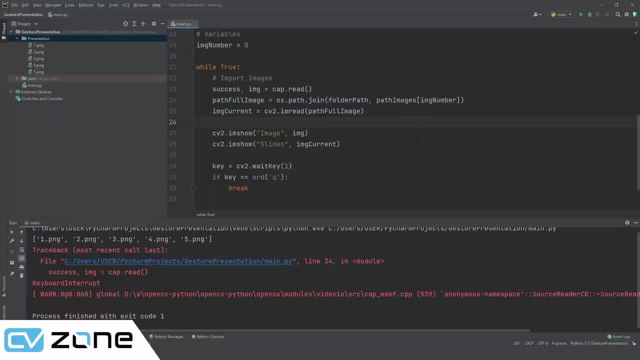 can make this image smaller and then we can put it on a corner. so it's very simple. how we can do this is, first of all, we have to define the size of it. so we can say: the height of the small image and the width of the small image equals 120 and 213. so these are numbers based on. 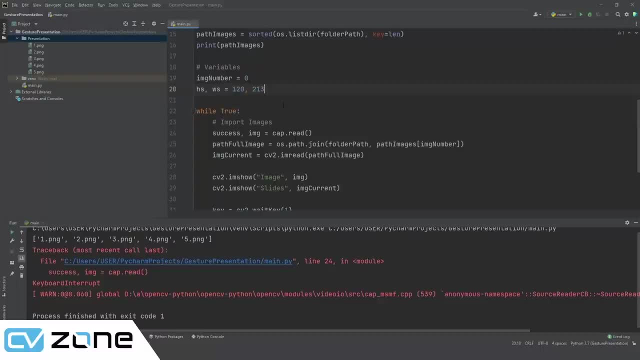 the actual size. you just divide it by, I think, 8 or 6, something like that, and you will get this. so and then, if you want to make it bigger or smaller, what you can do is you can multiply it by, let's say, 1.5 or something like that. I will keep it. 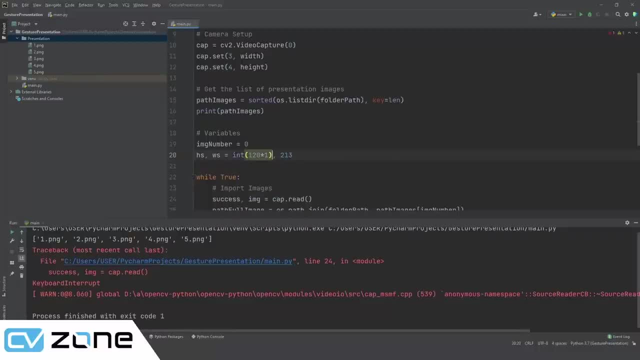 multiplied by 1. and if you multiply it by points, 1 point something 1.2, then you have to convert it into integer. so here I will write: integer multiplied by 1.2, let's say. so you can increase the size of this. that's why I'm keeping this here. 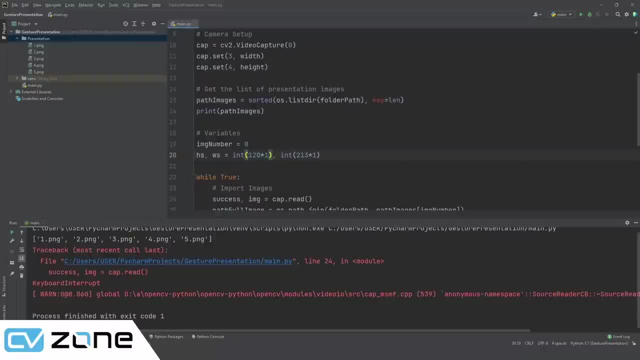 otherwise it's not really required. so if you want it a little bit bigger, a little bit smaller, you can change it from here. so now that we decided on the width and the height of this image, what we need to do is we need to place it on our actual image. so, first of all, we are 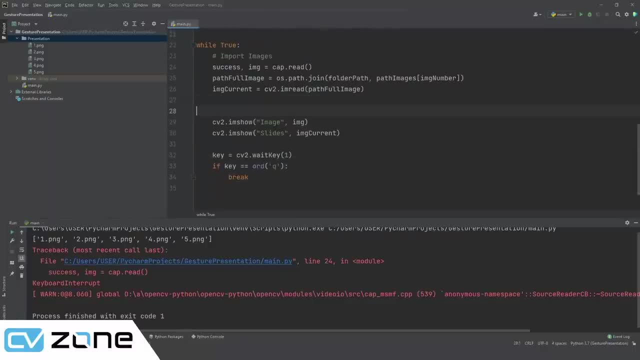 going to resize it. so here we are going to: let's just write here: adding: adding. okay, the caps lock is on adding, let's say, webcam image on the slides. so first thing we will do, we will create an image small. then we are going to resize it: cv2 dot resize and we will resize it based. 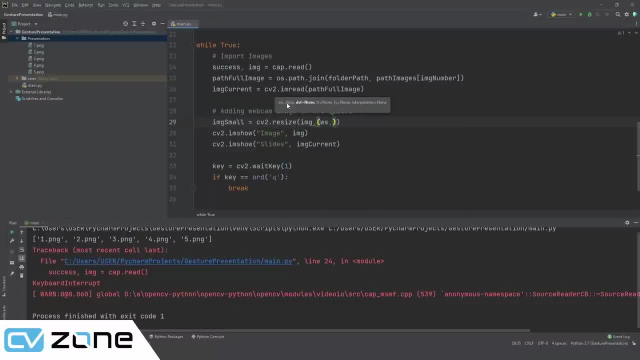 on the width and height. we decided so: WS and HS, width, height, width small and height small. so it will resize it this way and now we need to place it on our slides. so for the slides, we don't really know the width and height of those. so what? 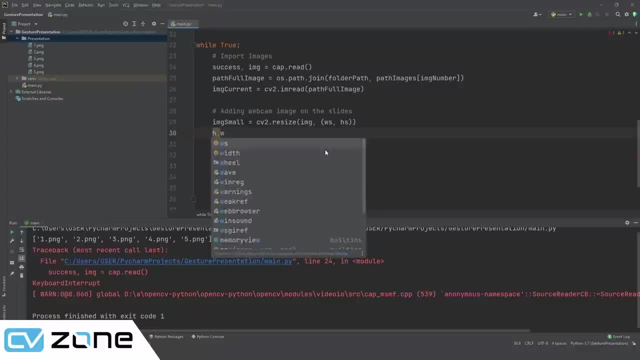 we can do is we can get the height and the width, and the channel equals image current dot shape, and that will give us the width and height of the slides. so now all we have to do is we have to place it on our image, so we will say that the image current. 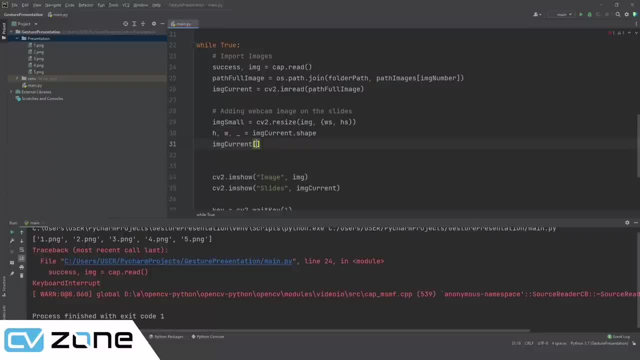 so it is a matrix. so what we need to do is we need to define the starting and the ending point of the matrix. so the starting point, what we are doing is we are putting it in the top right corner, so the starting points of the of the height will be zero. so we want 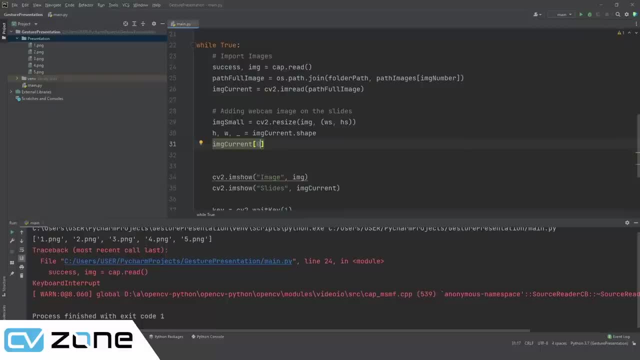 to start from zero. and the height. the ending point of the height will be the height of the small image right and the width will be a little bit tricky for the width. the starting width will be the total width minus the width of the small image and the ending point will be the total width. so that will give us the top right corner. 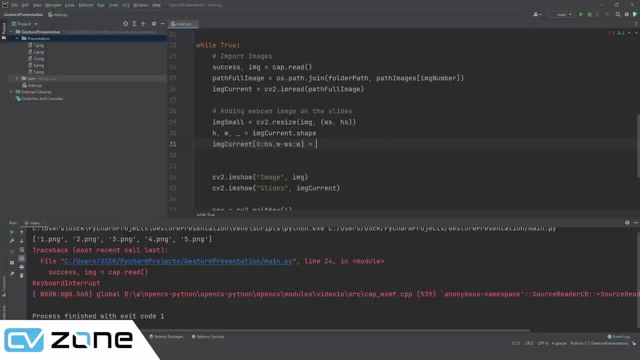 if you want to change, you can put it the bottom right or the top left or the bottom left, whatever you want, and so this is a matrix. now we want to change this matrix to image small, so we want to overlay that. this is what we are writing here. it's very simple. so if we run this now, 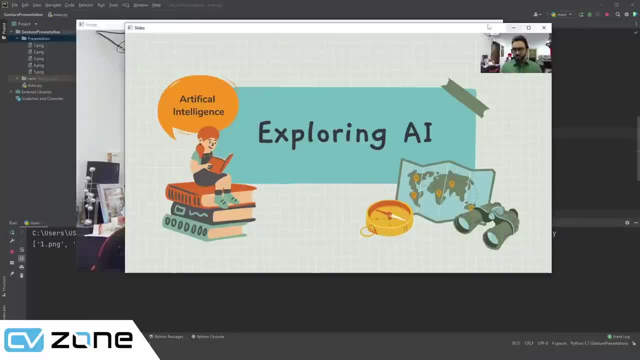 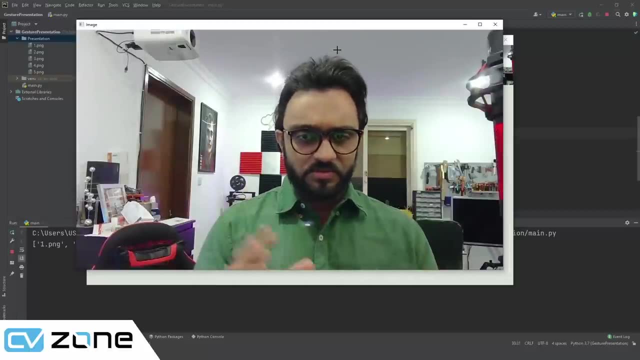 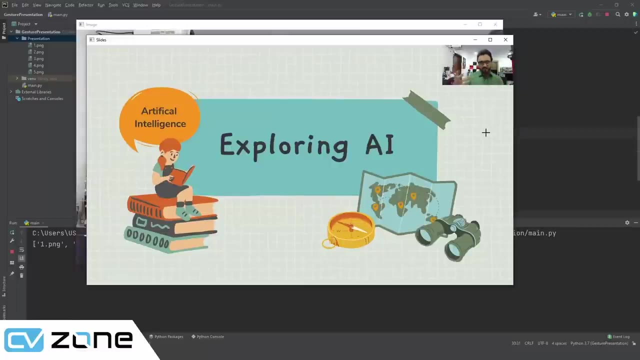 it will give us the image on the side always. so there you go. so you can see me now on the right hand corner. so if we wanted to, we could simply neglect this image. we don't have to display this at all, but for now, because we want it to display a little bit bigger, it's. 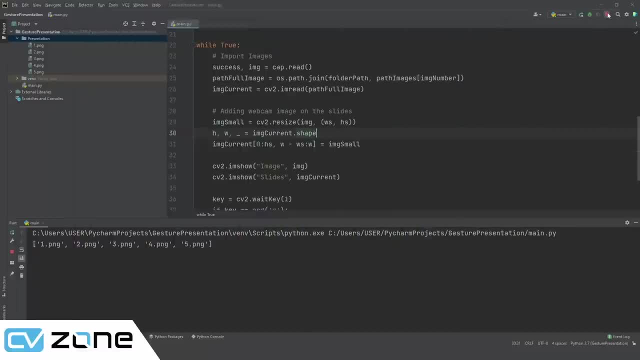 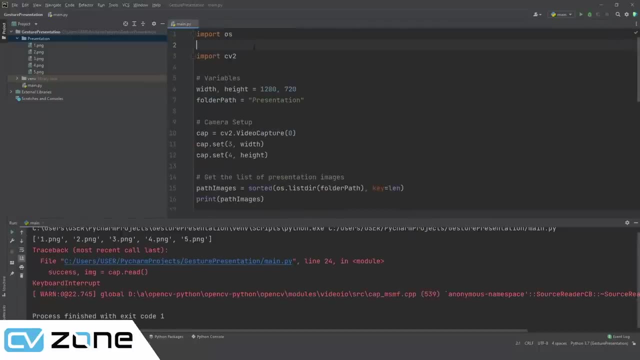 it's good to have that too. so that is good, and now we can move on to the hand tracking part. so now we are going to add the hand detector module. so what we will do is we will write here from cvzone dot hand tracking module, import hand detector and we are going to use this hand detector to find the hand and based. 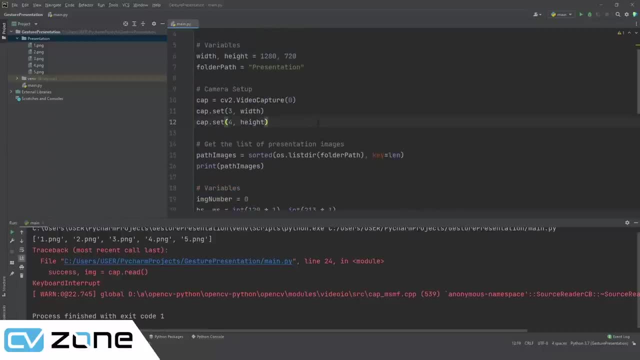 on that. we are going to apply some gestures. so here we will add our hand detector, so we will write here hand detector and uh, we will simply write: detector equals hand detector. and the detection confidence, detection, confidence, we want as 0.8, which means that if you're 80, sure that? 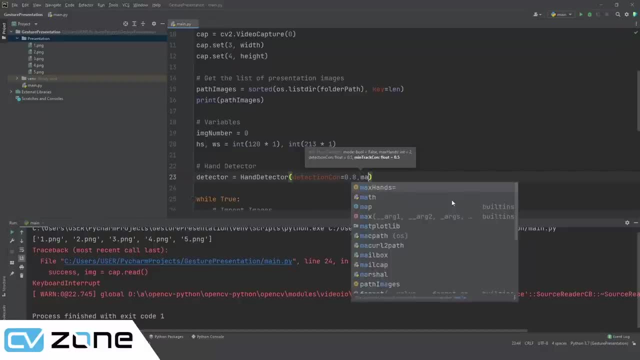 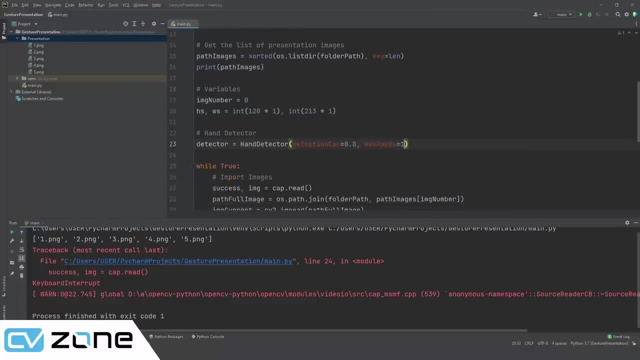 it's a hand, then consider it a hand, and then the maximum number of hands we should have are one, so we don't want multiple hands. once this is done, it's very simple to do: to add, to detect the hand. all we have to do is we have to go down here and let's just 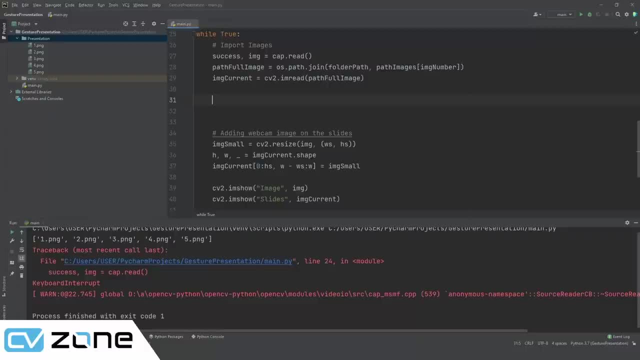 make some space here and we are going to say that detector, detector dot, find hands and we want to find it on based on this image. so once it finds the hands it will put it in hands and then it will output the image back so it will draw on. 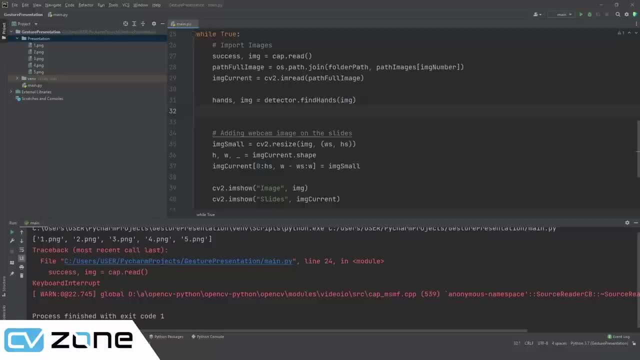 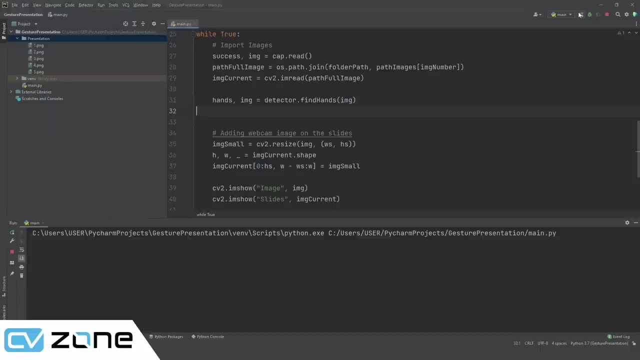 the image as well. so that's good, and once we get those hands, we can. okay, let's just run it first and see if everything is working so far, and then we'll go on to the next step. so there you go. so I have my hand here and you. 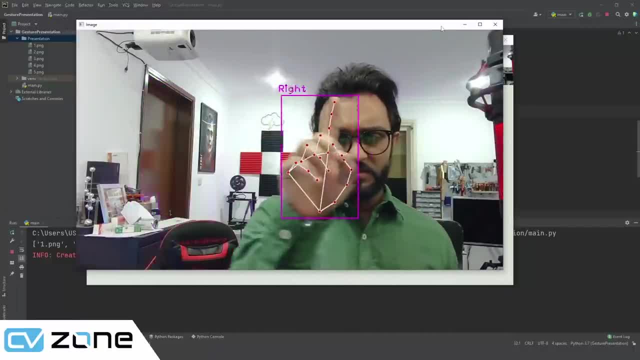 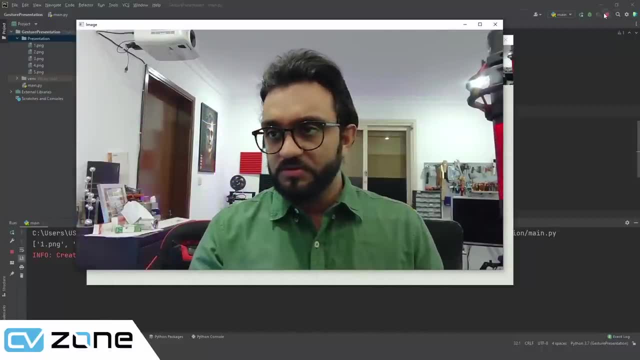 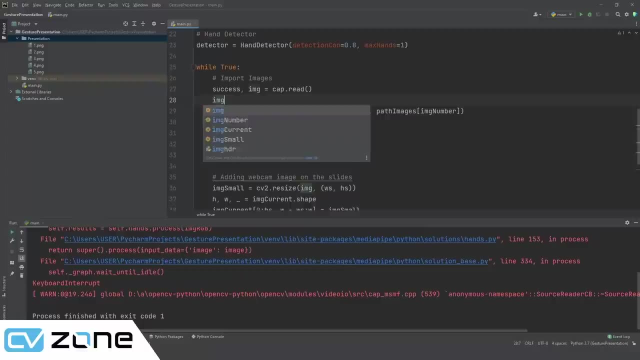 can see, it is a right hand being detected. but again, you, you can see, the problem here is that if I move to the right, it's moving to the left. so we need to flip the image. so it will be convenient when we are drawing, so it will be easier. so here we can write: image equals CV 2 dot flip and we want. 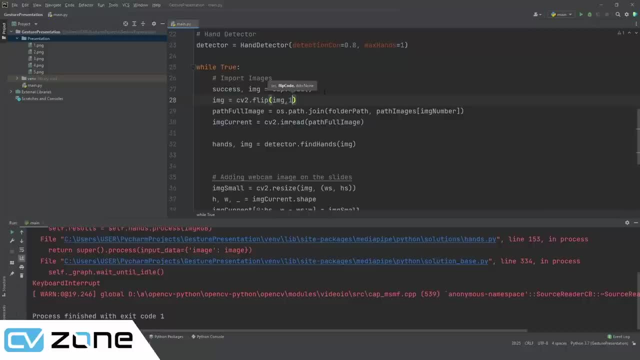 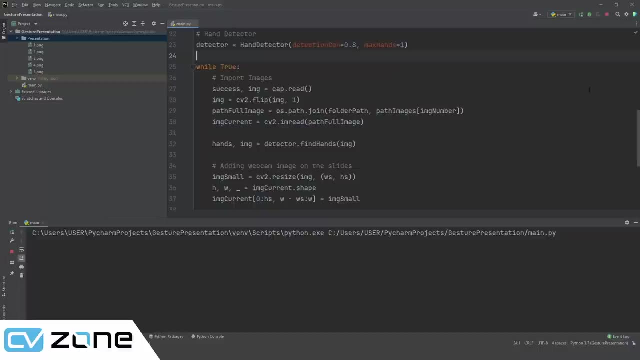 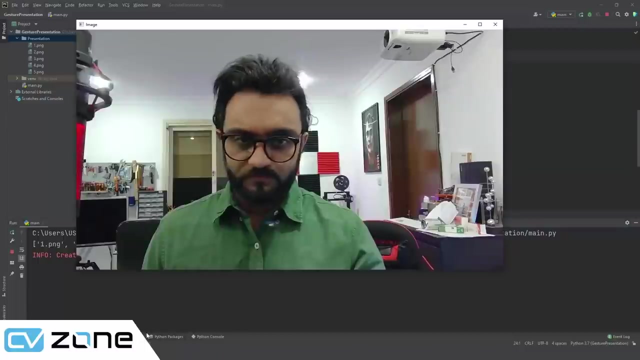 to flip our image in the horizontal direction. so 1 means horizontal, 0 means vertical, so we don't want to flip it in the vertical. so now, if I move it, you will be able to see there you go. so here you can see, this is our hand. if I move to the right, it's. 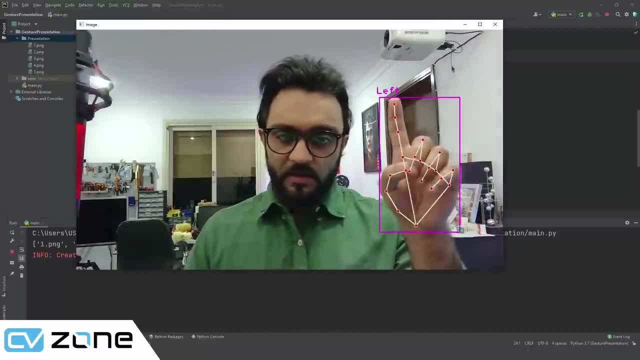 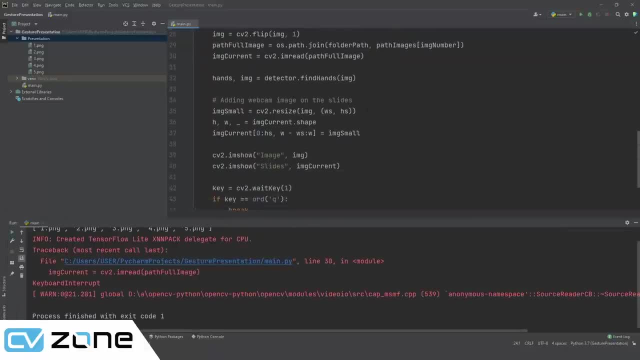 moving to the right. if I move to the left, it will move to the left. but the problem here is that it's saying left. so it's not really a problem in this case, because we are not going to use that functionality, but what you can do here. 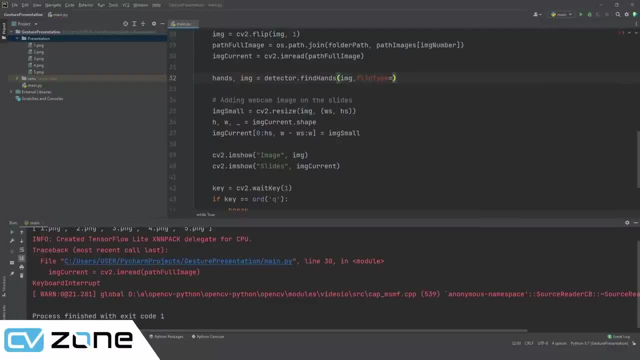 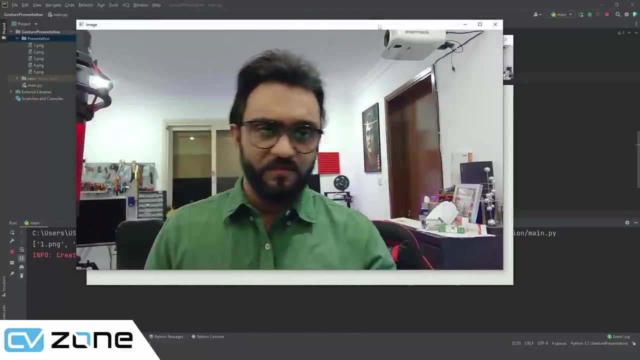 is. you can write here: flip type equals, I believe, false, false. so if we run that, that should solve that issue of left and right. so there you go, I'm gonna add two right, so let's go back here. and there you go. so now it's a right image, so everything is good okay. 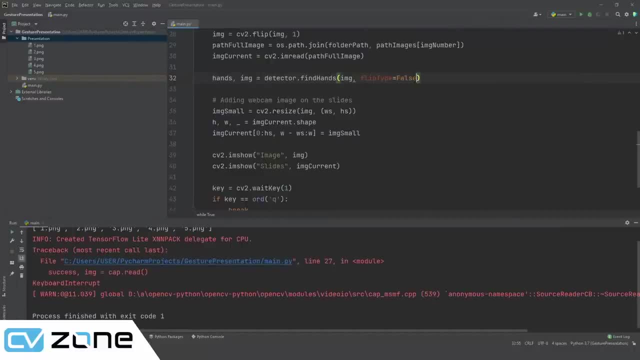 so, once we have this, we need to find if there is a hand detected, if we have hands, if anything is present in the hands- it's basically what you call the list- then we need to get the landmarks of this hand. so, and we also need to get the number of fingers that are available, that are up, so what? 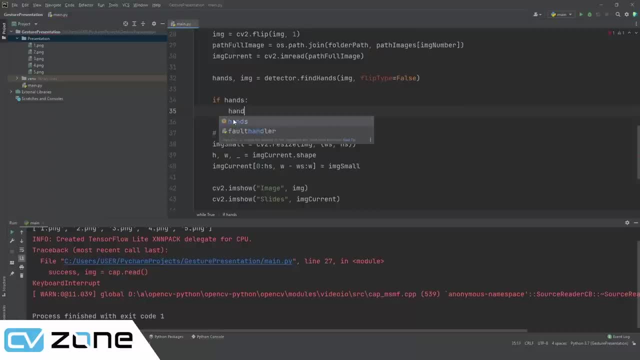 we will do is, first of all, we will get the hand- so hand equals hands- at zero. again, it is a list, so it can have multiple hands. it can have one, two, three, four hands. so what we will do is we will get the first one and we know it will be only one, because the maximum number of hands equals one. 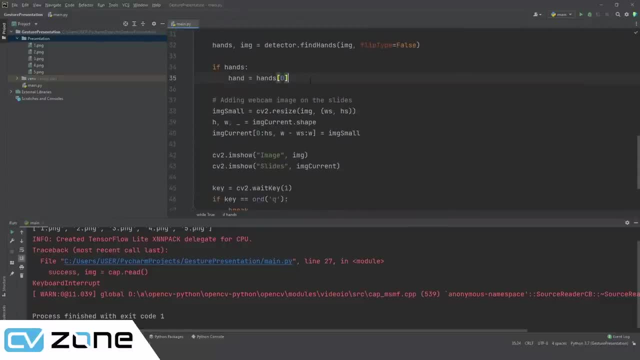 so that's why we are putting zero, because we just need the first one. once we have that, now in order to control the gestures we need to know how many fingers are actually up. so we have a very convenient function to check that. it's called fingers up, so we can write: detector dot, fingers up. and which hand do you want to check? 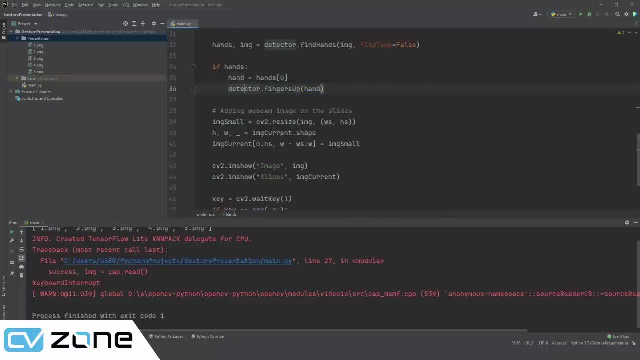 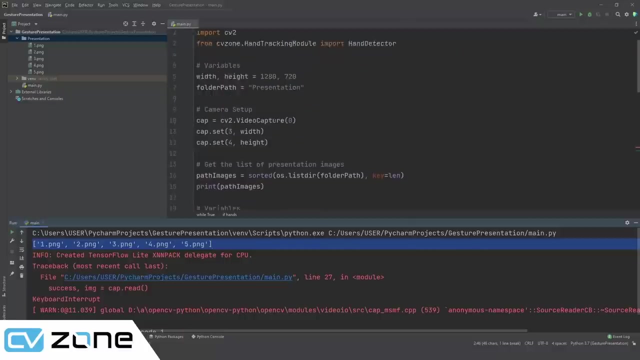 you have to give in the hand so it will check how many fingers are up and it will give us a list. so here we will call it fingers and then we can print it out to see what it looks like. are we printing anything else? no, so that's the first one. we can remove that as well. 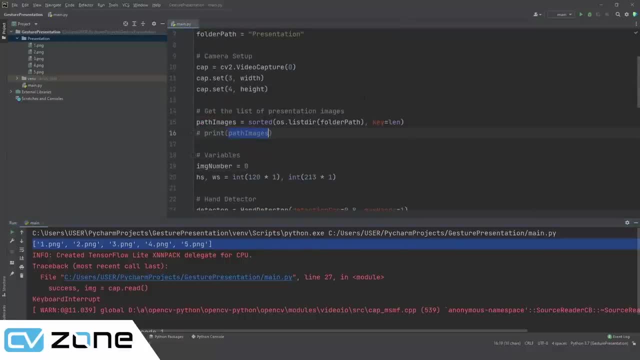 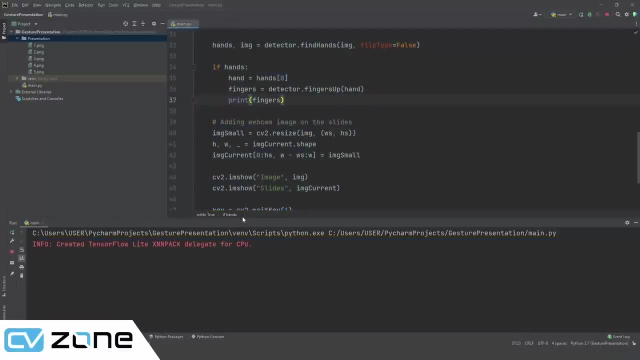 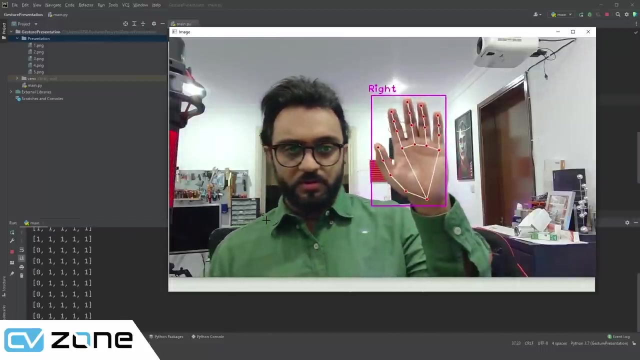 so let's just comment this and yeah, so we will go to fingers and let's just see what it looks like so that we know what we are applying um later on. so here on the side, you will see on the um, on the console, you will see that i have, uh, the fingers up at this point. so if we close, 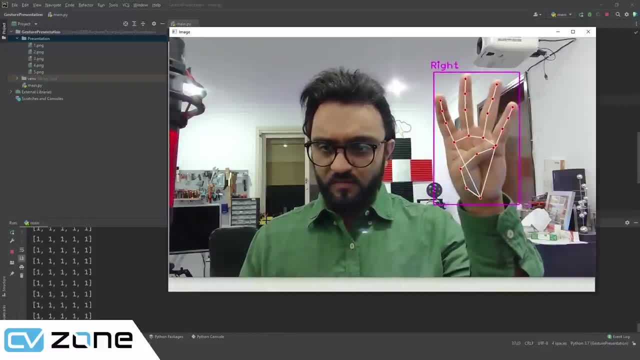 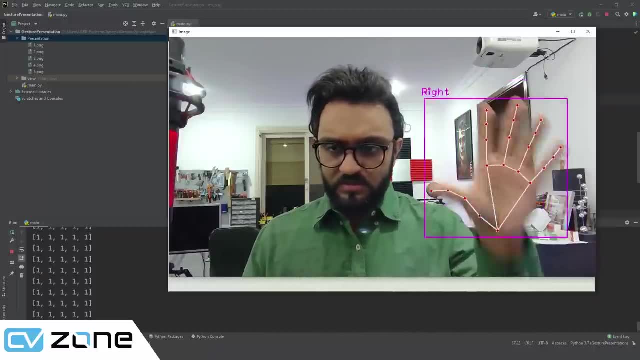 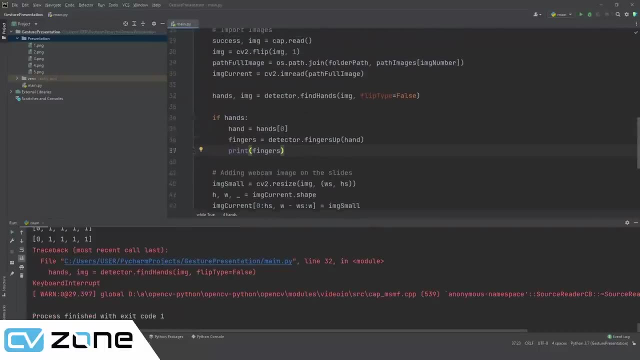 you can see this is one, two, three, four. so right now, uh, the, the left and right are wrong. uh, let's just check. why is it wrong? uh, because i believe it's the left and right problem, so we might have to fix that. are we going to use the thumb? uh? 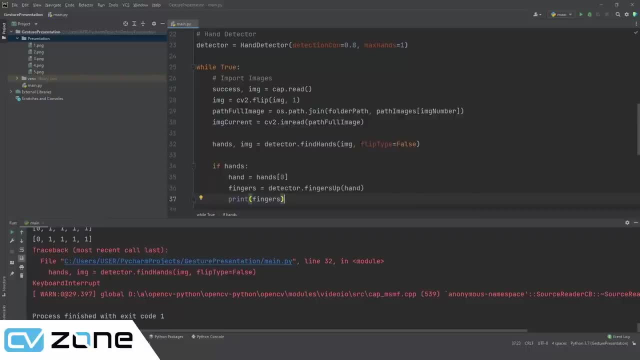 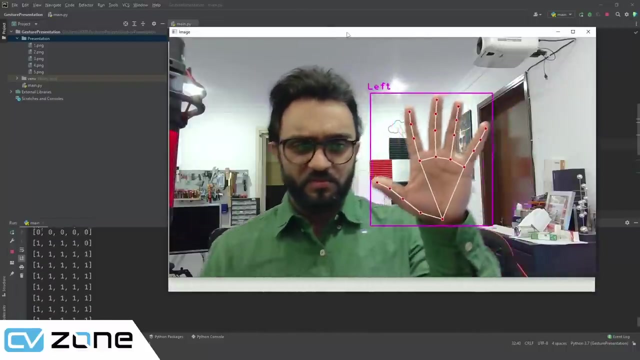 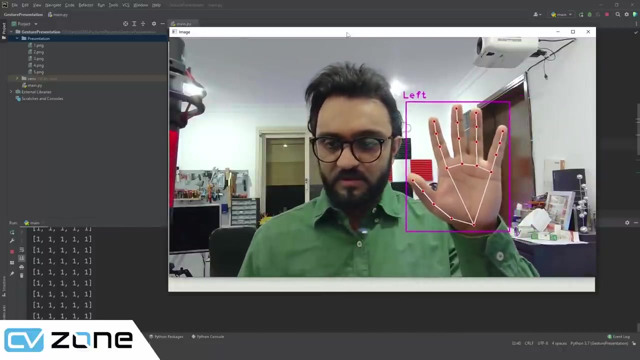 really so we are not really going to use the thumb, so it might not be a problem. let me just remove that. let's try that here. yeah, so now. now it's fine. so the only thing, the problematic part is this number, it's this value that says left the string. but other than that, now it's. 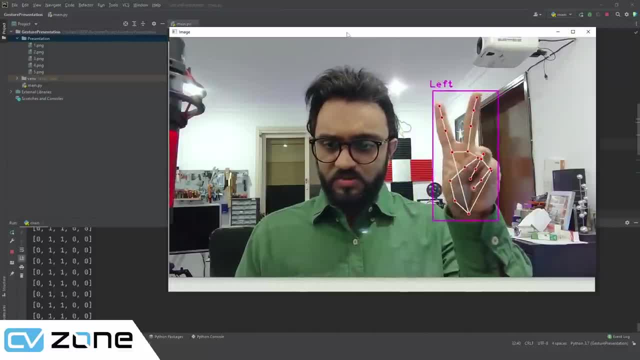 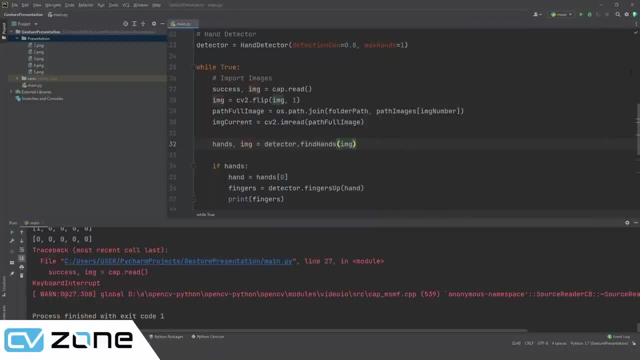 working fine. so we have one, two, three, four and five. so all of them are working fine. so that's good. so what we will do next is we are going to, based on these- what do you call number of fingers up, we are going to apply some gestures, so, but 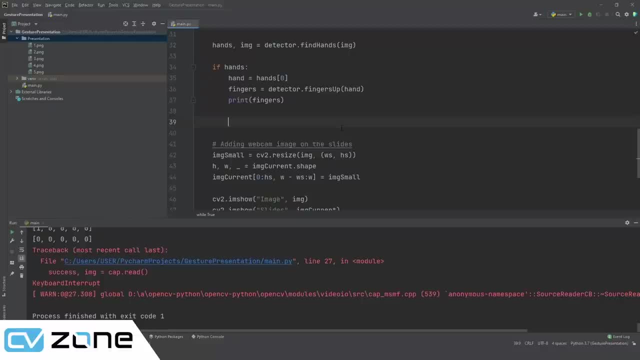 before we do that, what we want to make sure is that when we apply a gesture, it has to be close to your face, actually above your face, so that when you are presenting, when you're normally presenting, it should not have an effect. so if you don't do that, then anytime you. 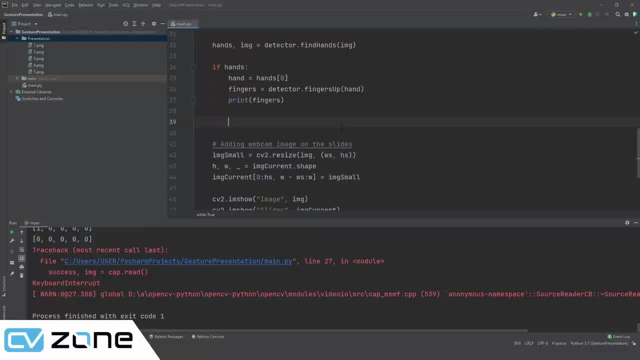 are moving your hand, your fingers might become one or two or something like that, and then it might trigger the problem, it might trigger the slide. so we don't want to do that. so normally in a presentation you won't put your hand up above your face so that that could be a good place to add a gesture, and it will not look. 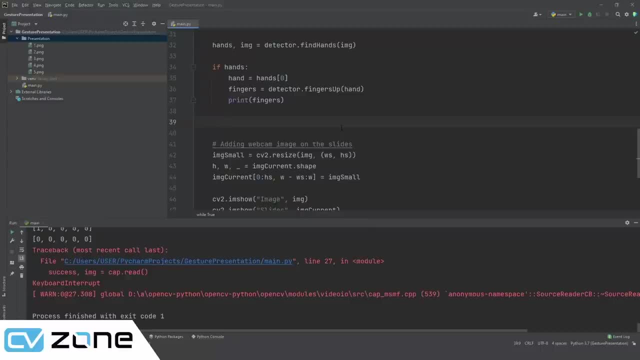 that good if you are moving your hand above your face and you are moving your awkward when you apply it only once. so let's, let's have a look at how it looks like. so what we can do is we can draw a line to check the threshold. so let's. 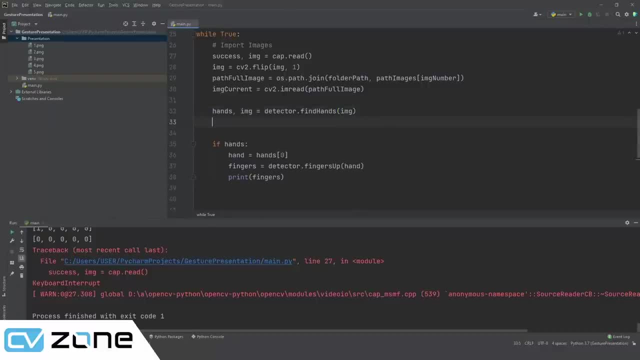 just call it draw. draw a line, cv2 dot line and we want to draw it on our image. and we we have. we have to define a threshold. so let's say, in the variables we define it as a gesture threshold equals, let's say, 300. so if the value is 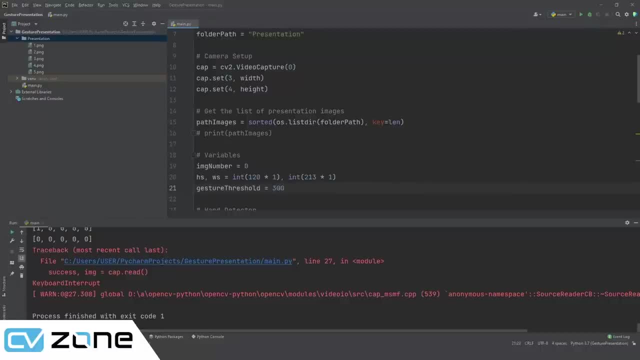 below 300, which means it's above my line, then we will say that detect the gestures. so here we are going to write zero gesture threshold. so this is the starting point. so the width will be zero and the height will be the gesture threshold and then the the point number. 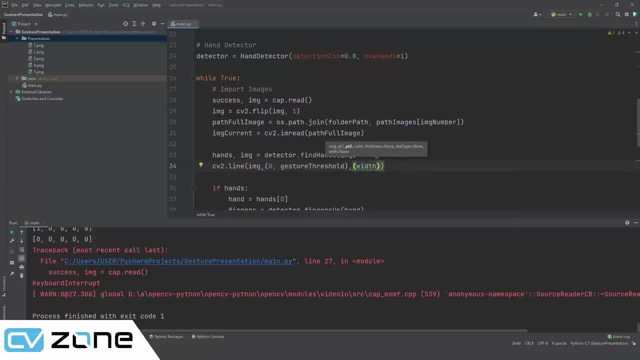 two will be the width at the end of the image and then the gesture threshold again, so you will see what it looks like. it will be more clear once we see it and then we will give it a thickness of 10. we're giving it a big thickness so that we can see it in the smaller image as. 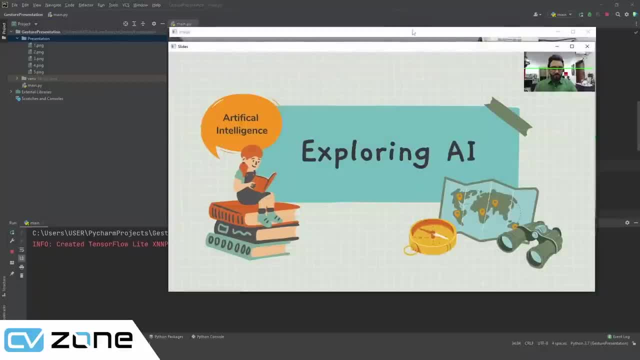 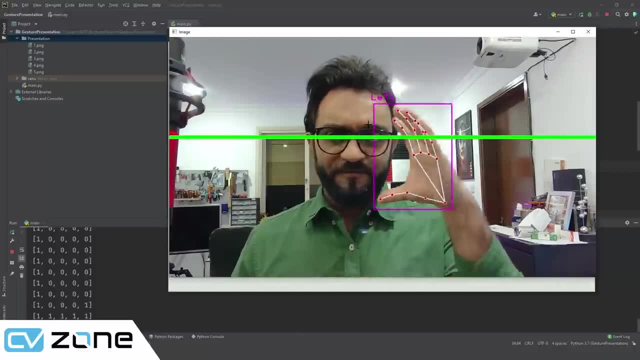 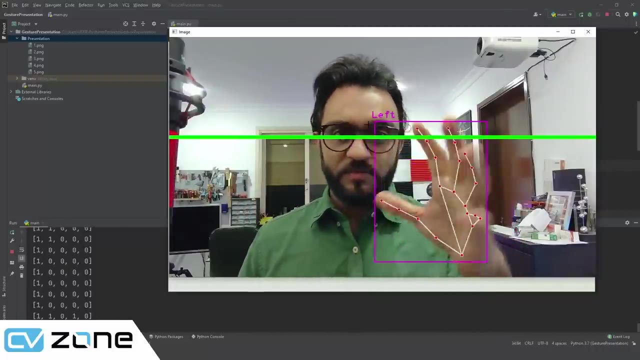 well, so there you go. so this is the threshold. so what I recommend to do is that put your face put align your camera so that your face is in the middle of this line, so, while you're presenting that, that should be the placement of the camera. so then you can simply do this and you can do the. 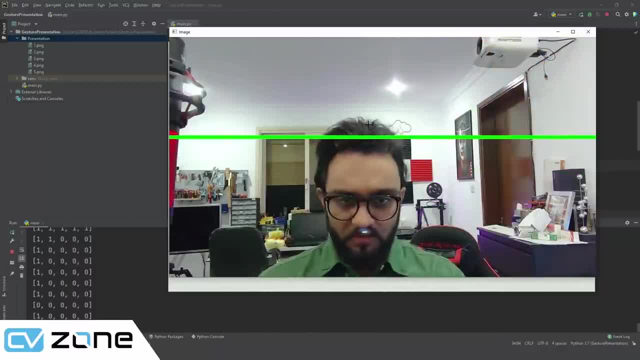 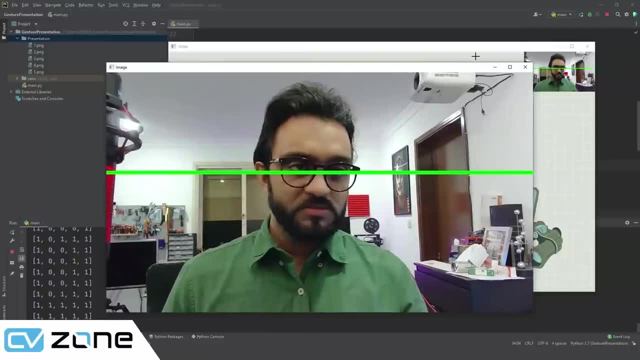 gesture. here it doesn't look that awkward, but if it's like really below a and you go up, it will be a little bit weird. so try to align it to the center of your face, so then here you can see it as well, the line. so that is good. so now 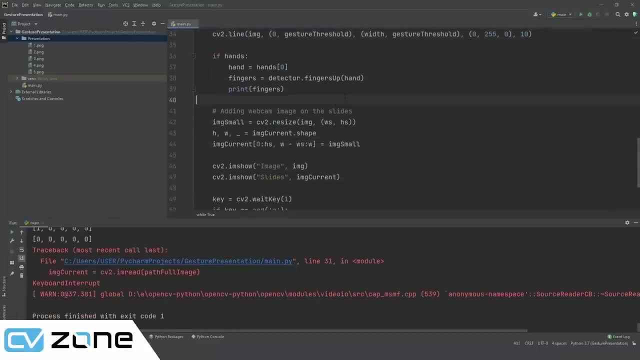 that we know this position. we will check that. if, if our, the center of our hand is above this point, above this line, then we are going to accept the gestures. so first of all, we need the center point of that hand. so we will write center X and center Y equals hand and we will get. 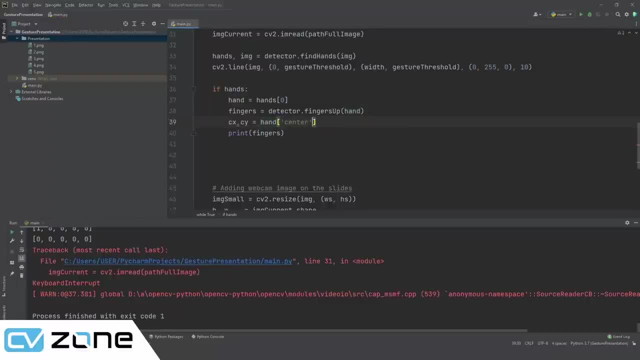 it's a dictionary, so we will write center and it will give us the center values. so now we can simply write: if our C? Y is less than or equal to the gesture threshold, then we are going to check the gestures. so here we are basically writing. if hand is at the height of the face, if hand is: 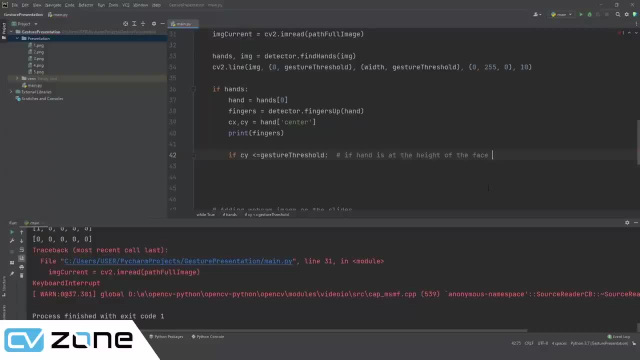 at the height of the face. so if that is the case, then we are going to check the gestures. so this is gesture number one. let's say that this is left. and then we well, so this gesture number one. what do we do? we will check if the fingers equal. 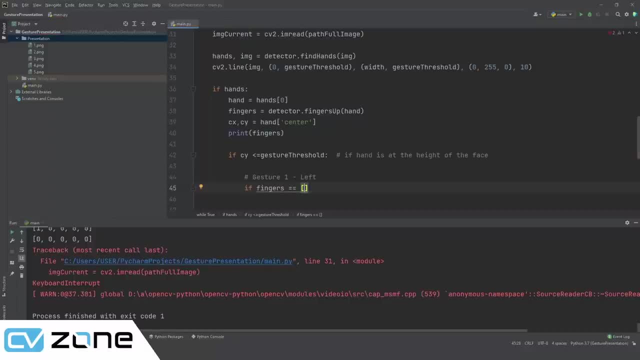 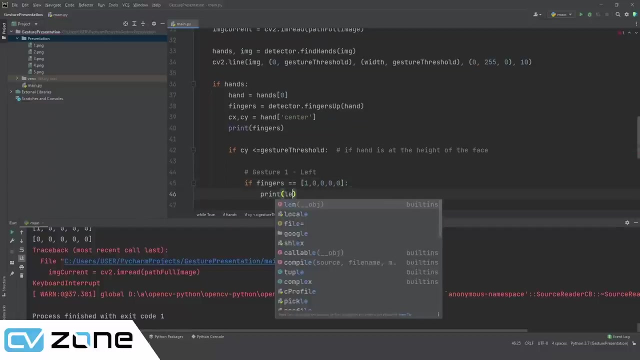 so what we will do is we will use the thumb and the pinky finger to go left and right, so it's very simple to use that. so what we will write is is: one. so this will be: thumb, zero, zero, zero, zero. so if this is the case, then print left. 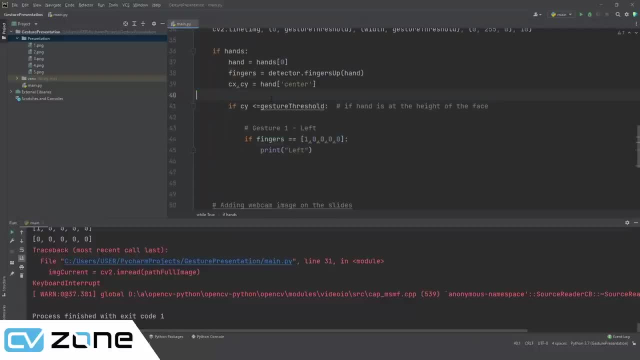 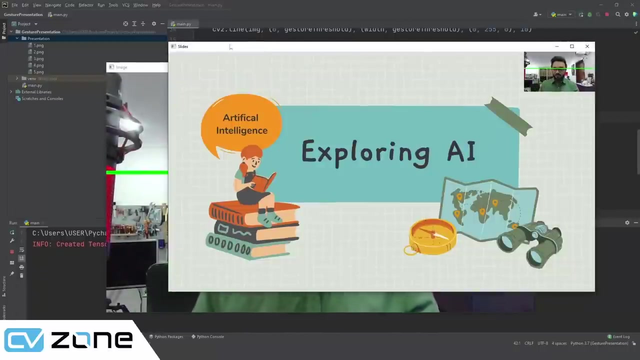 so let's just try to understand what we have done so far. first of all, our hand must be above that line and if we point uh, if we uh, open up our thumb and close everything else, then it should go, it should print out left. so in this case, okay, let's bring this in front in this case, if i do, 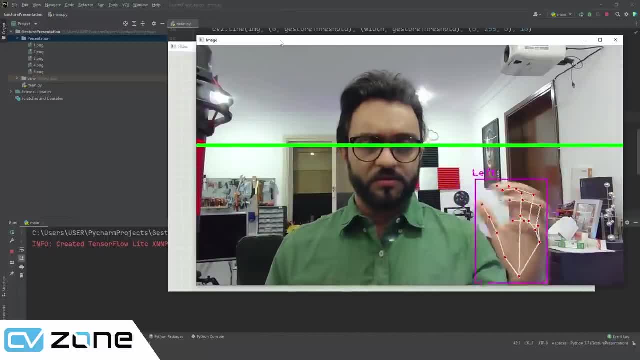 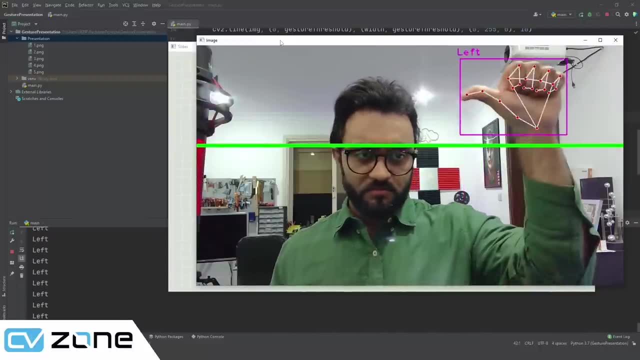 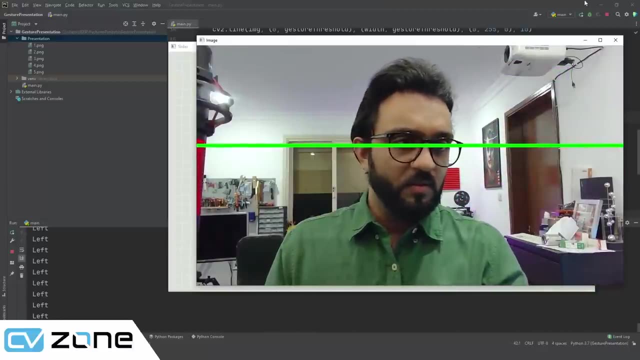 this. it will not print anything. you can see, there's nothing on the console. but if i go above and do this, then it says left, left, left, right. so we can do that. and if we go down, nothing will happen. if we go up something, or let's say we will go to the left side. so this is good. now we know. 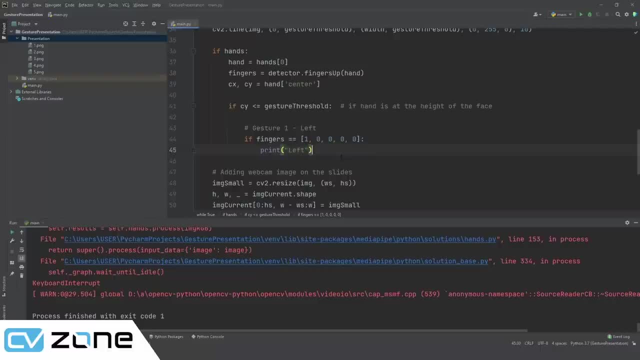 that left is working, and the same thing we will do with the right. actually, let's copy the comment as well. so this is gesture one, and oh, what happened there. so this gesture two, and we will write it as right, and this one will be zero, and now we will use the pinky finger, so it. 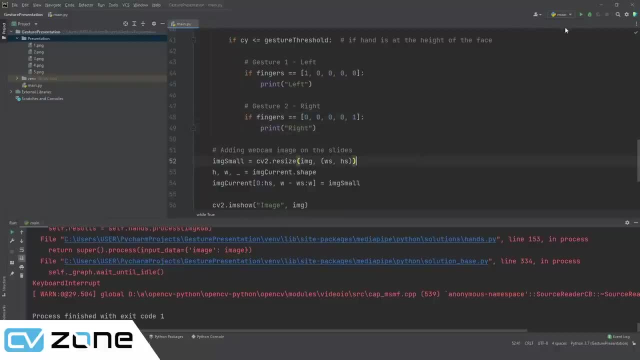 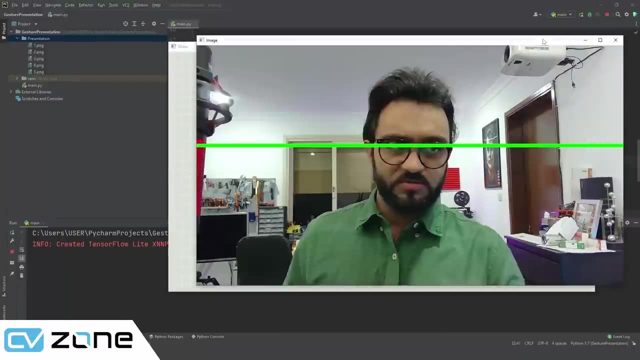 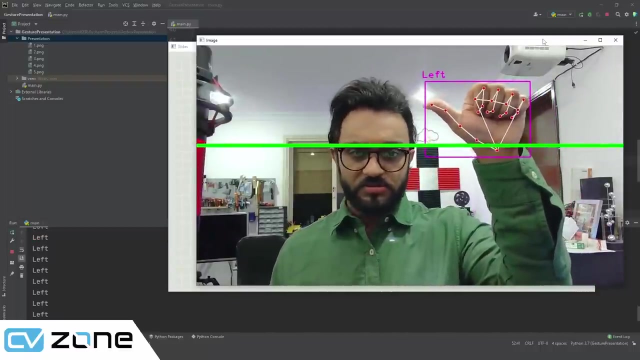 will be one. so here we will write right. so let's run that. so we are just testing the gesture at this point and later on we will assign something to it. so here, if i do left right, nothing happens. but if i go up and do left, it goes to the left right, it goes to the left right, it goes to the. 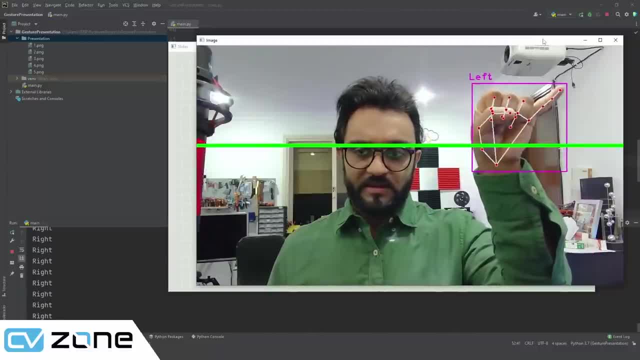 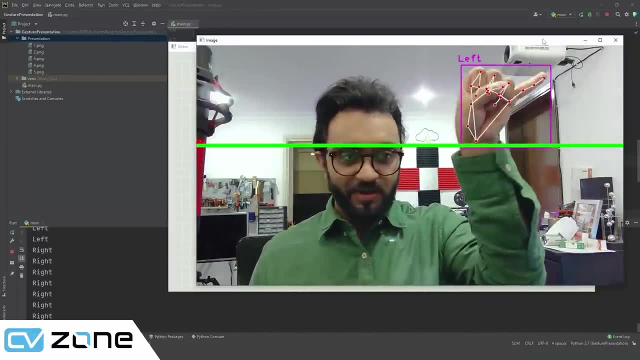 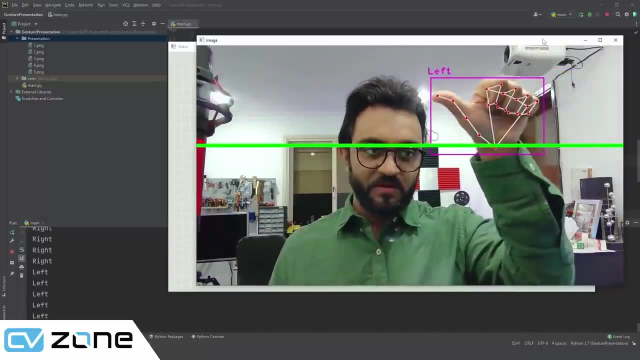 left, it goes to the right. there you go. it's very simple and normally you would not do this in a slide or in a presentation. so this will be weird if you are doing this in a presentation, uh, without any context. so this is a good place to start. so it is like a semicolon, like you normally don't use. 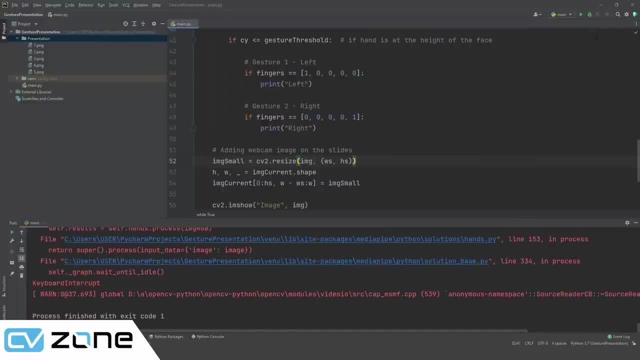 that's why you have that in programming languages, that it's the end of line anyways. so then, what we will do now we are going to do is we are going to do a little bit of programming. so we are going to do now we need to assign when this is pressed. so what we will do, we will write here that the image. 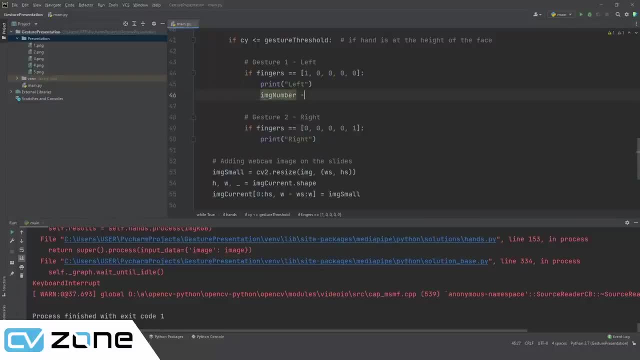 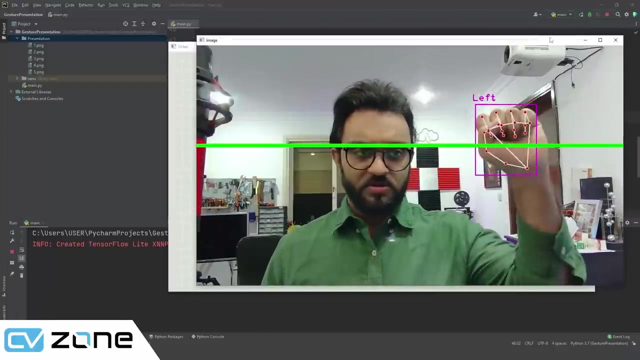 number minus equals one. so if we want to go to the left, just reduce the image number, and if we want to go to the right, just increase the image number. that's how simple, it is, right. so let's run that and see if it works. okay. so let's go to the right and we have an error. uh, it was left, by the way, but again it's. 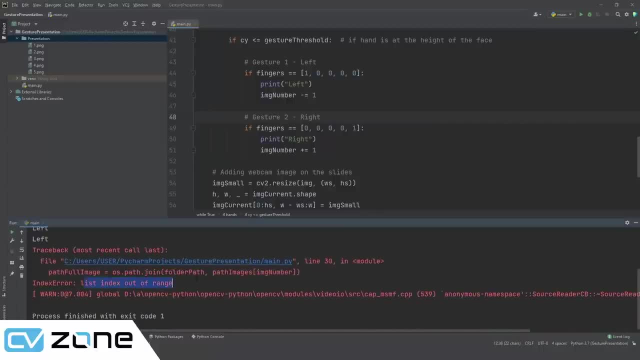 an error. what's the error? the error is that the list index is out of range. so we were already at zero. we were at zero and then we told it to go negative one, so it became minus one. so now there is no list at, there is no value. so what we need to do is we need to make sure that if the image 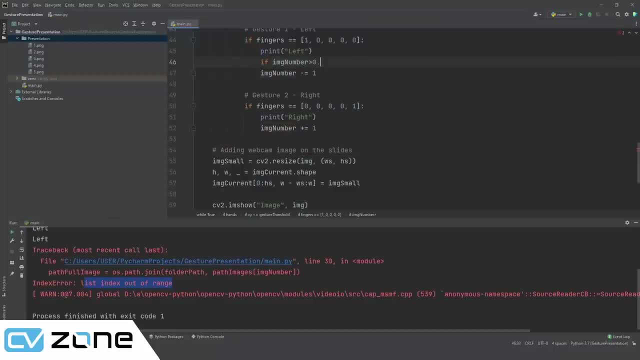 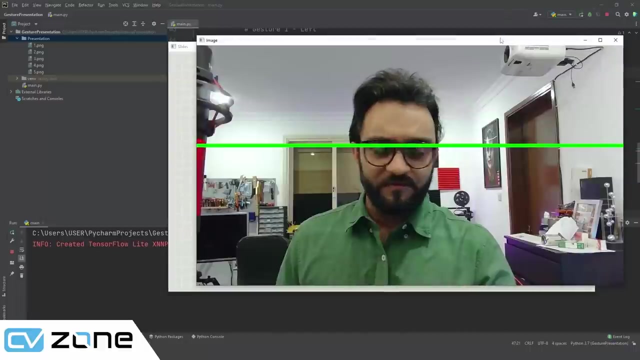 number is greater than zero, then we do this. otherwise, if it's not, then we will not change the number. okay, so if it's greater than zero, then we will do this. so in in this case, if i put the left again, it will not give me an error. 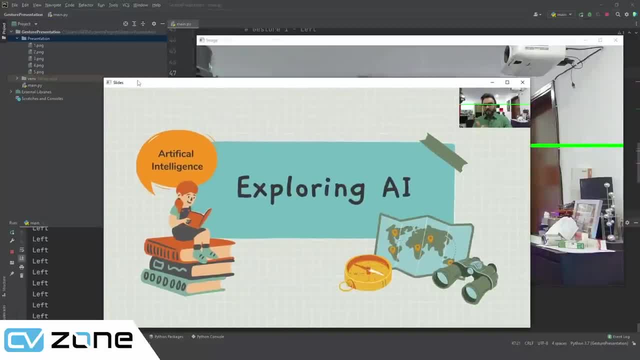 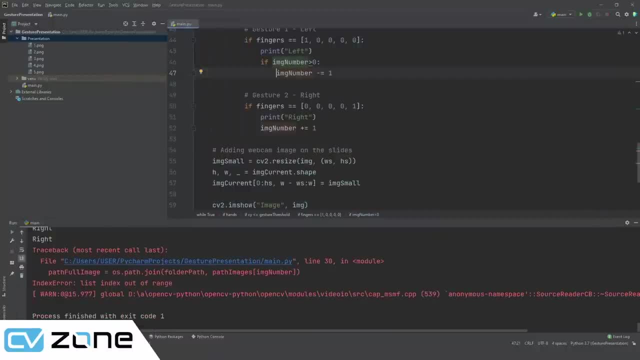 but there is no left slide, so it will not go any further on the other direction. but if i do right, you saw it actually went a little bit further. it went till the end of the slide, it went till number five, and then it gave an error again. it gave an error because it went to slide number five and 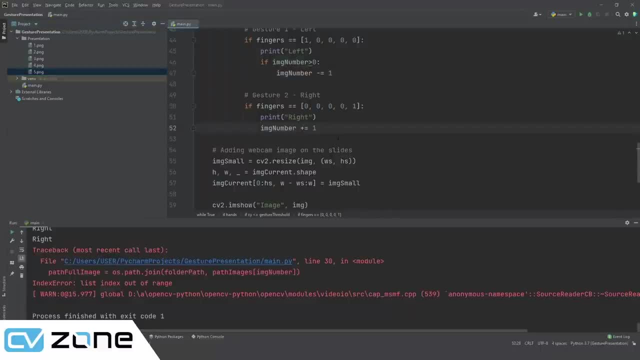 then it added one more, it became five or six, and then that number was not present in the list, so it gave an error. so that's it. what we need to do is we will give an limit here as well, that if the image number is less than 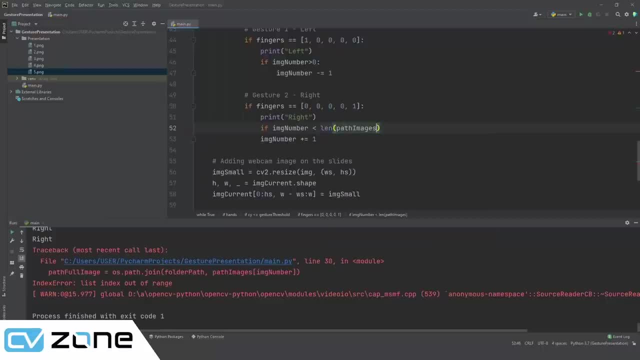 the length of our path images. so this is the path images where we loaded all the numbers. so if we go at the top, uh, yeah, so these are the five that we have, so this value will be five, so but we will write minus one, so if it is four. 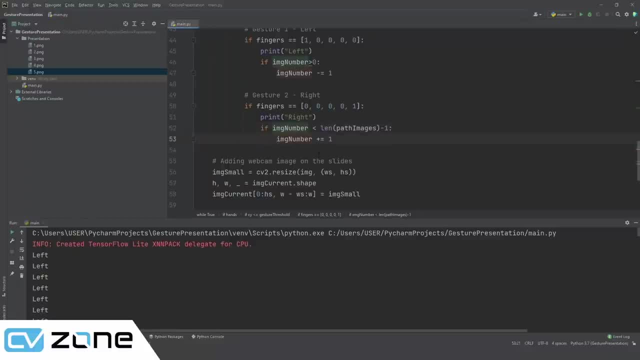 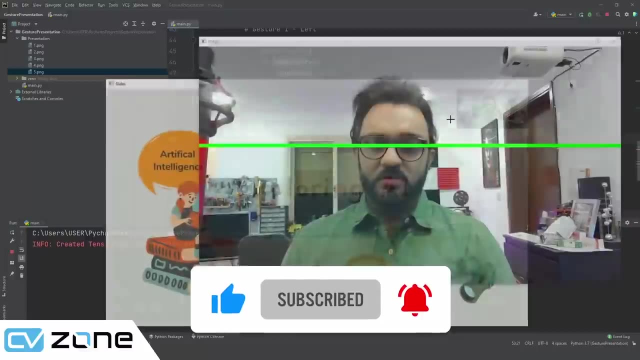 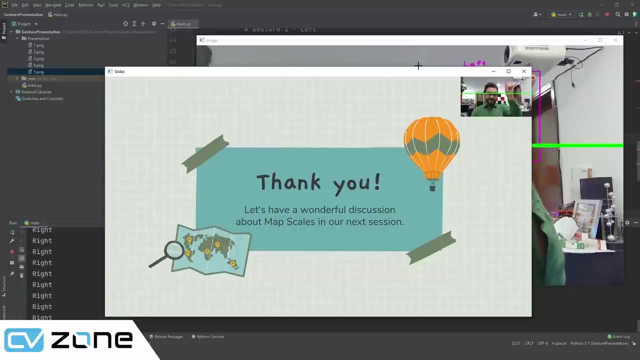 then we can add one more right. so that's the maximum you can call. so you can go more than that. so let's try it. so, uh, yeah, so if i go to the left, nothing happens. if i go to the right, it goes till the end, but it doesn't give you an error. and if i go to the left, it. 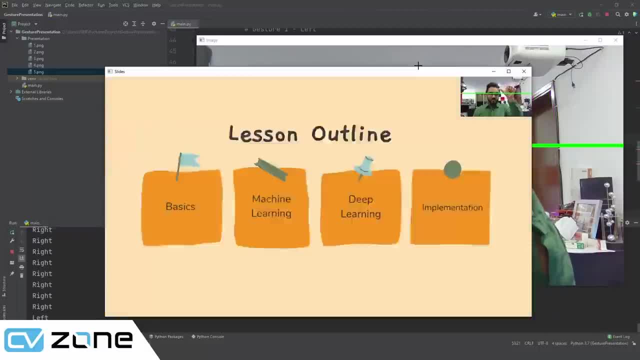 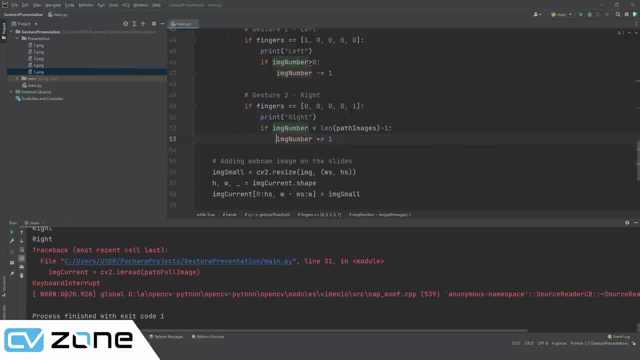 quickly goes to the left and right. so this is a problem. so it is happening so fast that there is um. it's clicking multiple times, so it is triggering all the slides at once. so we need to fix that. how can we fix that? it's very simple: we need to introduce a variable called button pressed and 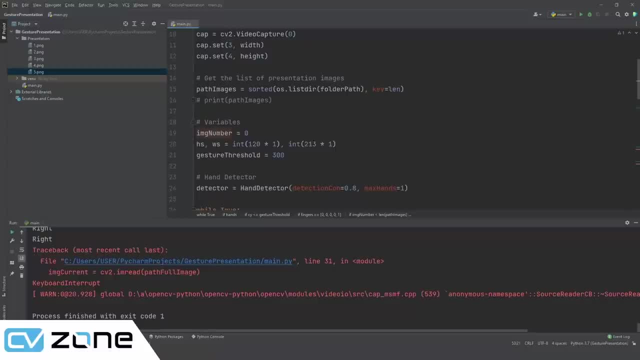 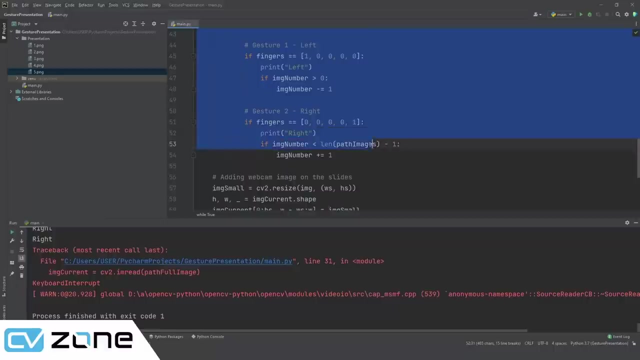 whenever it presses the button, we are going to wait till we can press the other one again. so here we will call it: button pressed equals false and to to do all of this, to do all of this, the button pressed should be false. so if there is a hand available and 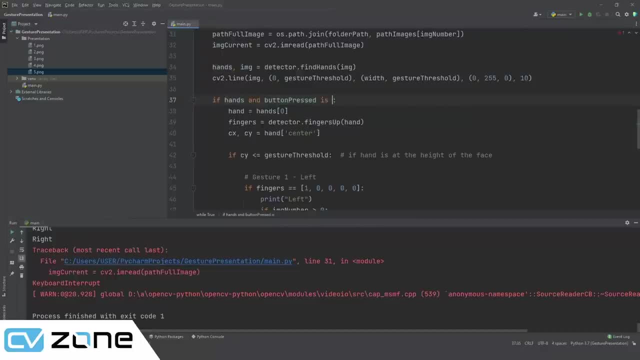 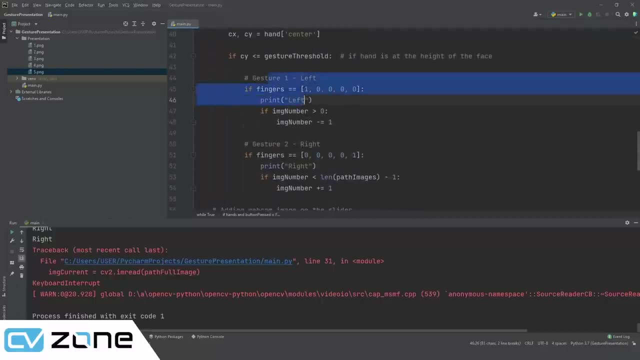 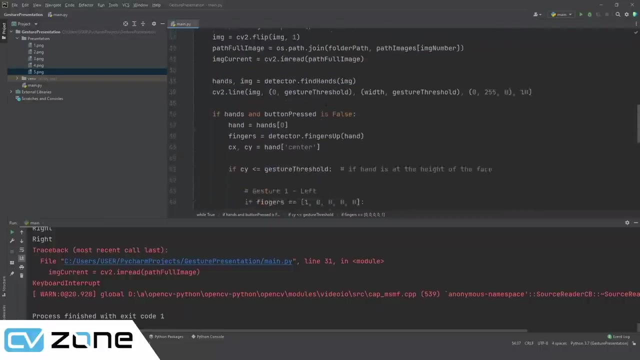 the button pressed is false, then it will do this right. so whenever, whenever there is a gesture applied, we will write here that the button pressed becomes true. so, whether it's this gesture or this gesture, whatever it is, we will say: the button pressed becomes true, so it will not go here. but then it will never go back here unless we make it false. 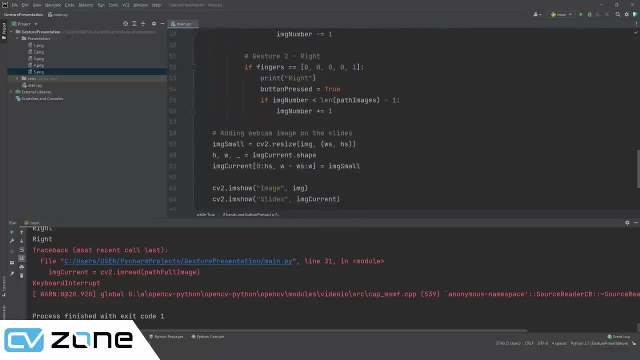 again. so when do we make it false? we go down here and outside the loop, outside the if statement, outside this if statement, we, we, we going to write here, so let's say, button pressed iterations. so here we are going to write a little bit of iteration, so we will write if we'll write here, if button. 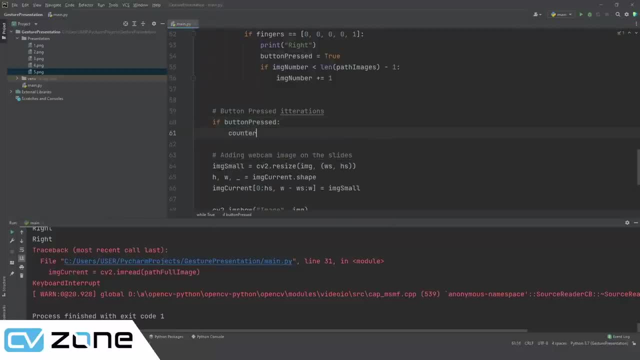 pressed. if that is true, then counter plus equals one. so we will- or let's call it button counter button, counter button. counter plus equals one. so we will go back here and here we will write: button counter equals zero. so here button counter plus one. and then we are going to say: if the button counter button, 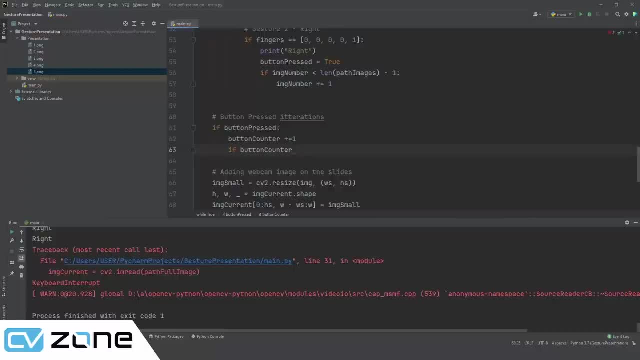 counter is greater than is greater than the delay. so now what is the delay? or let's call it button delay, button delay. so button delay will be a value. for example, it will be number of frames, so 5 frames or 10 frames, it should not do anything, it should not accept another button press. 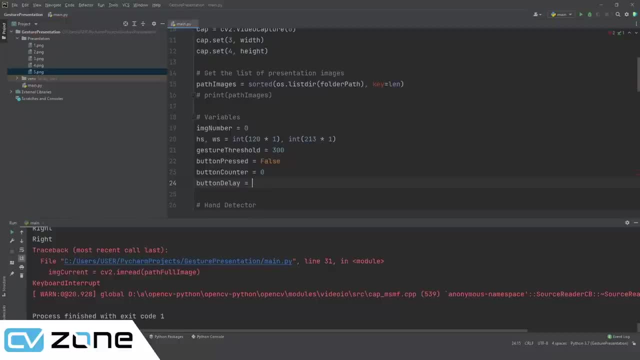 so button delay. we will call it, let's say, 10, so 10 frames. it should not do anything else. so if it's greater than 10, then we will put the button counter as 0 and we will put the button pressed equal false. so now it will accept another button press. 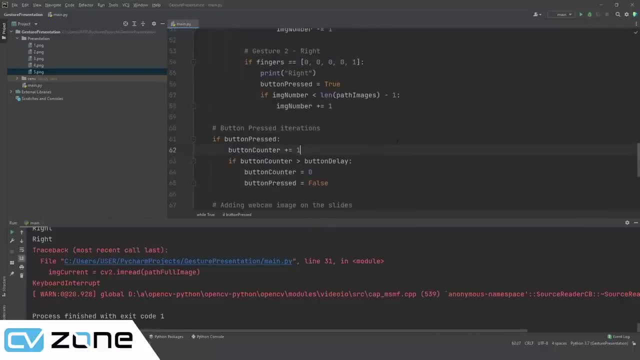 spellings are wrong here. there you go. so yeah, so that is the idea. so we have now: whenever the button is pressed, then it will accept. another button press, so now accepts. actually, we can put it here inside, because if it's outside it's not really adding or reducing a number. so, yeah, we can put it here. 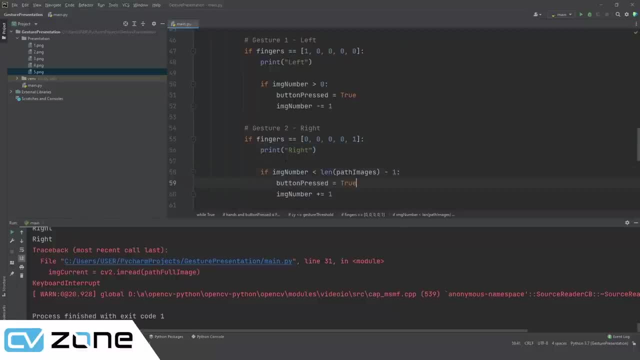 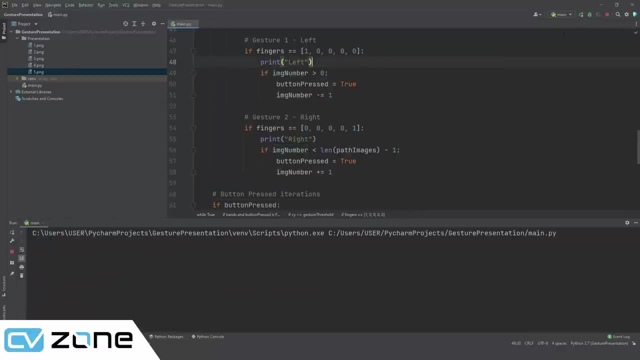 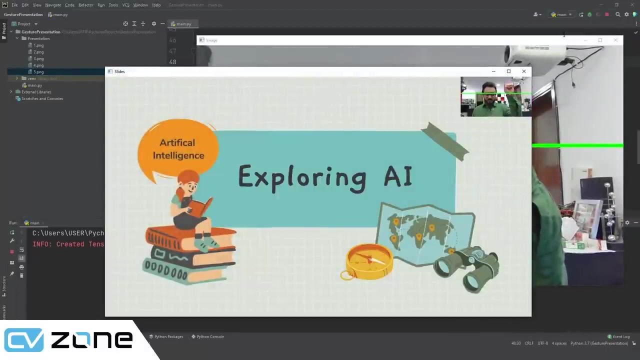 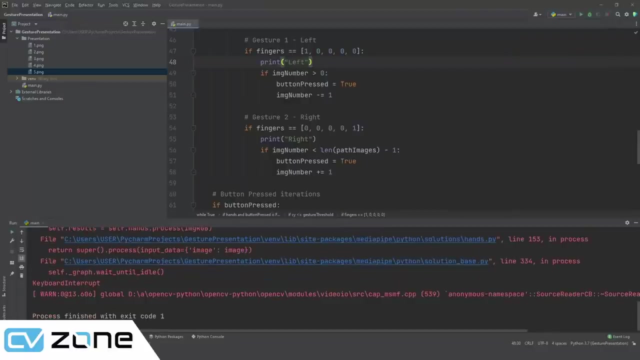 so let's put it here when it's actually making a change. oh, there you go, so let's run that and see if it works. so now i will do. uh, right, oh, it is still a bit fast, so let's change it to what is it right now? 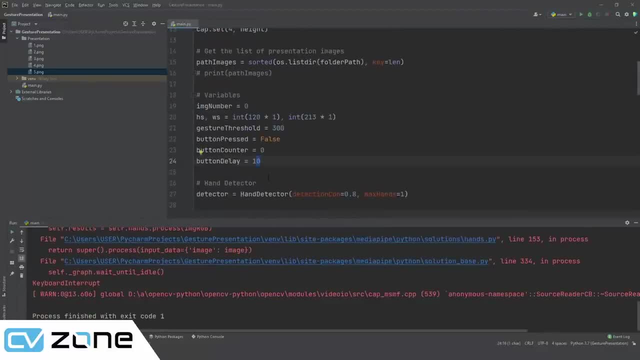 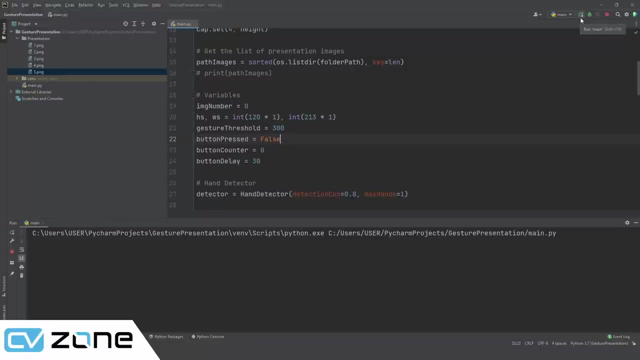 10. actually it's going really fast. maybe it's going more than 40 frames per second, 40, 50, because the camera i'm using, the webcam, can go up to 60, so maybe it's really fast. so let's put 30, 30 frames, let's see so 30 if you're running at 30. 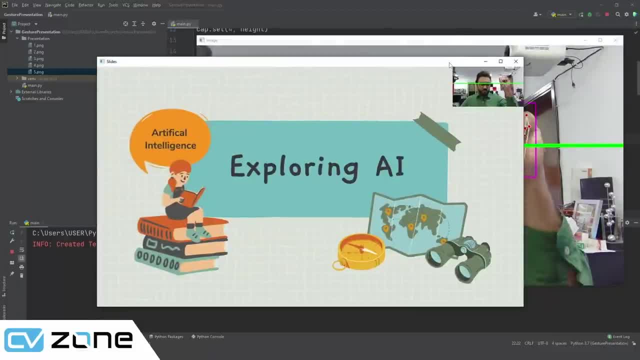 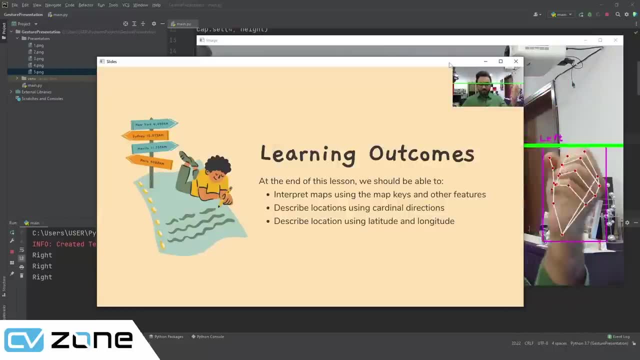 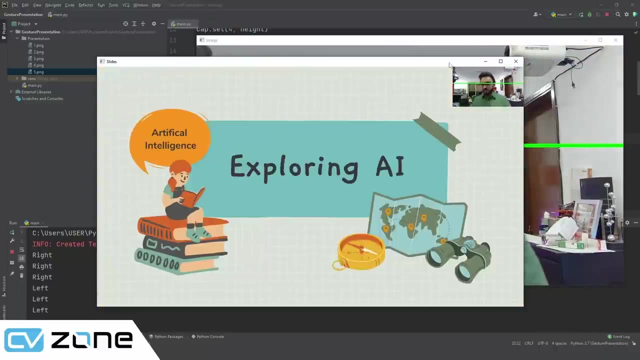 fps. it should be one second. so let's do this. there you go. now. it's, uh, more reasonable if i do that again. it goes forward, again, goes forward, backwards, backwards, backwards. so now it's more responsive and it is something that is more usable, so it is easy to work with. 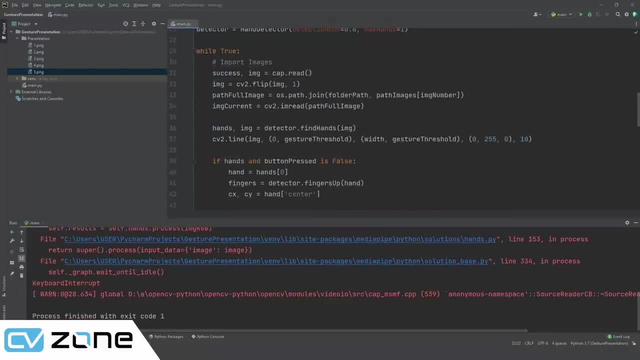 there you go. so now the back, and uh, fourth gesture is done. so we have done two of them. now the third one will be to actually draw. so the drawing part is actually a little bit trickier than this. it's not as simple as the other gestures, but it is quite simple. it's not that hard, so let's. 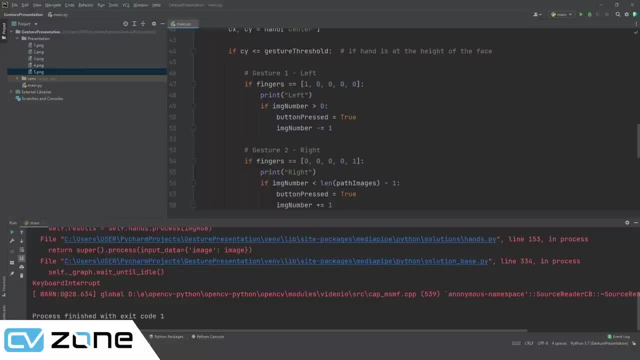 go ahead and start with the drawing. so the first step here will be to actually add our pointer. so let's write here that this is gesture 3, show pointer, and what we will do is, whenever we have two fingers up the index and the middle finger up, it will show us the pointer. so we 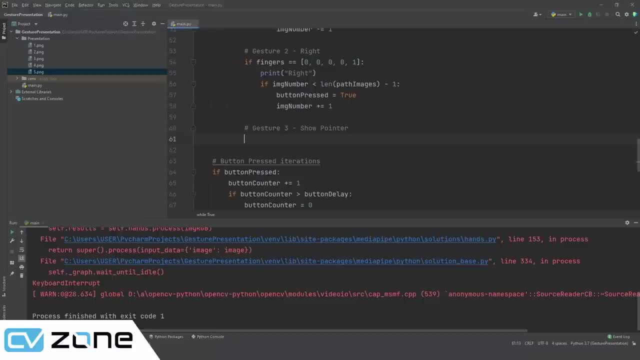 will not draw it, but it will be a pointer. we want to draw it with a single finger because it will be easier. otherwise you can flip the idea as well if you wanted to. so here we will write: if fingers- let's copy that because we are lazy- if fingers, uh, if both of them are up. if index and. 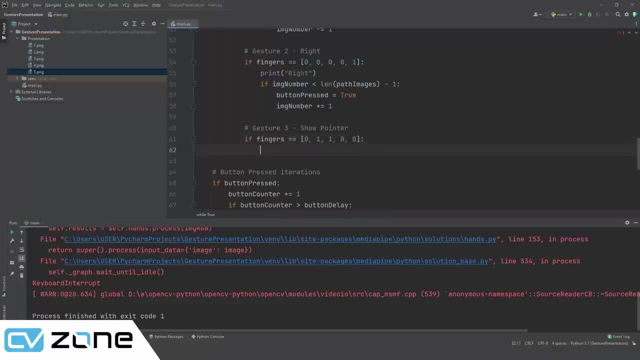 the middle finger are up, then we are going to draw a pointer. so the pointer will be cv2 dot circle and we will draw it on our image current, not on the image. and because image current is the slide, so we want to draw on the slide, then we have to draw, uh, our 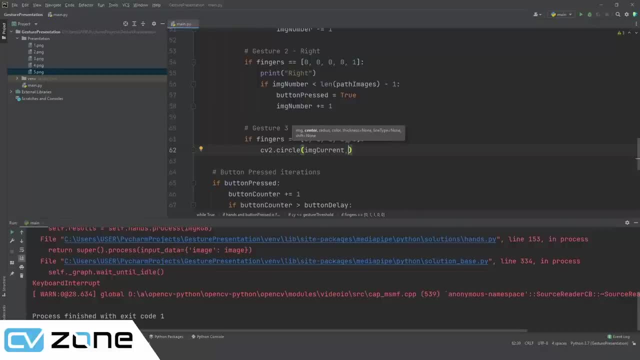 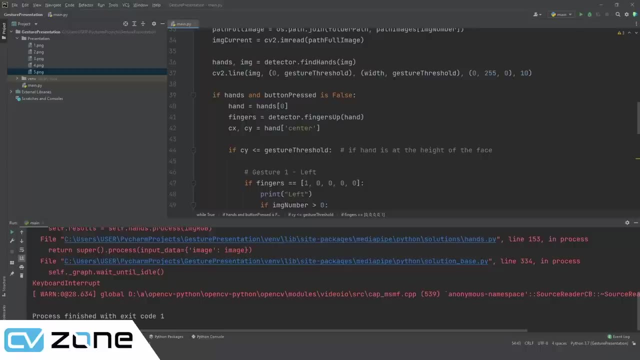 point where the index finger is. so where is the index finger? uh, we didn't actually get it, so, um, let's, let's get it here. so our index finger equals: um, it will come from the lm list, so let's find the lm list first. so lm list. 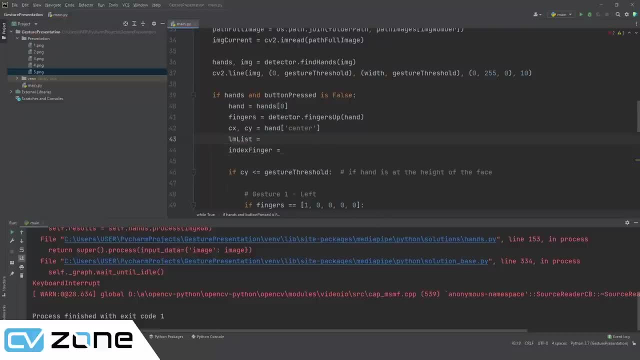 basically it means landmark list is basically the hand and we will get the dictionary, the value of lm list. so from this lm list we want to get the point number eight. so the point number eight is basically the index finger, and we want to get- uh yeah, we want to get the value number zero and we want to get the value number one. 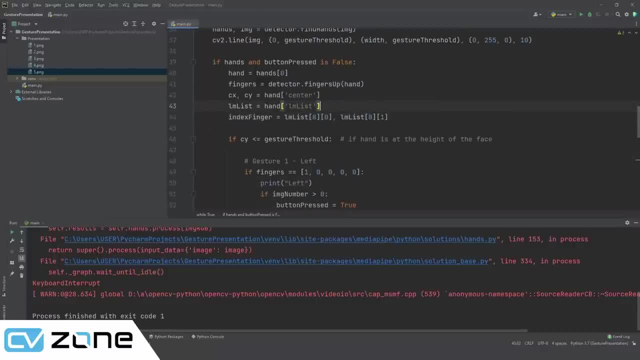 so these are the two values that we need. so that will be our index. it will have the third value as well for the z, but we don't want that. so this is the index finger. so here we are going to write that we want to draw the circle on the. 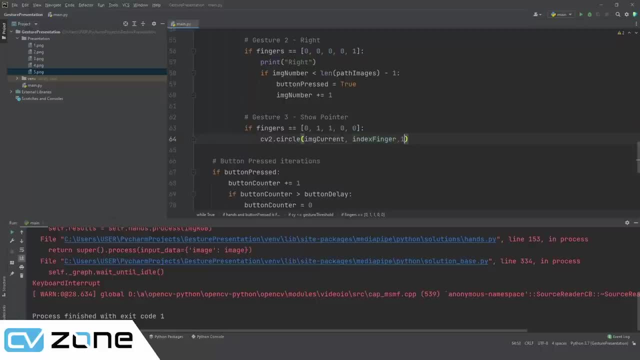 index finger point and we will give it a big value, let's say 12 for the radius, and we will give it a color of red. so 0, 0, 2, 5, 5, and then we will write cv2 dot filled. we want it filled. 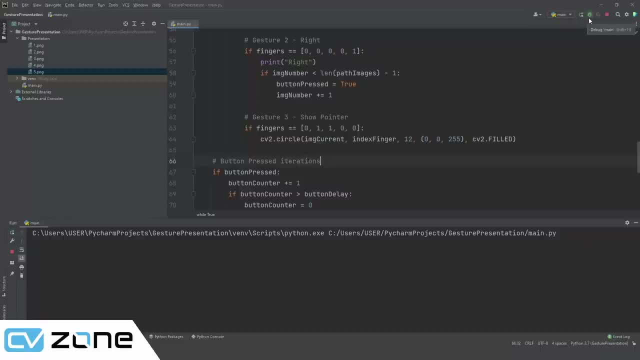 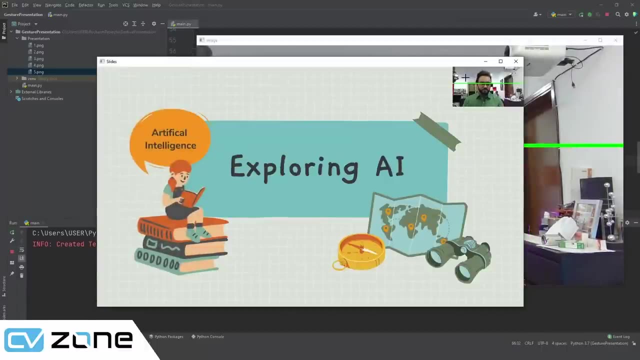 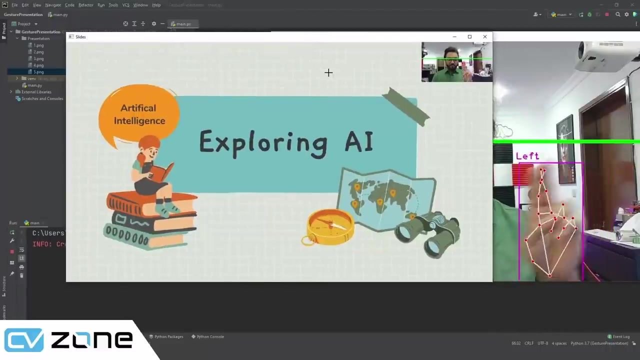 so that should be good. so let's go ahead and see if that works. um, so here if we put, okay, what is happening? okay, here, if we do put two fingers, nothing happens. so this is a problem, because we don't want to, uh, have the limitation of- uh, what do you call this line to actually draw? 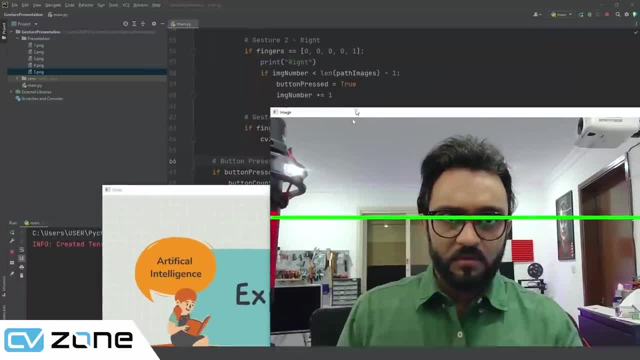 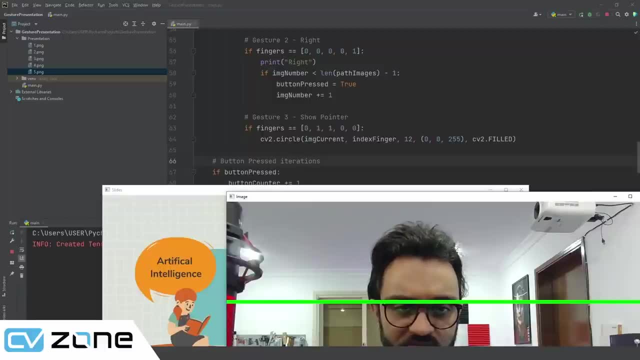 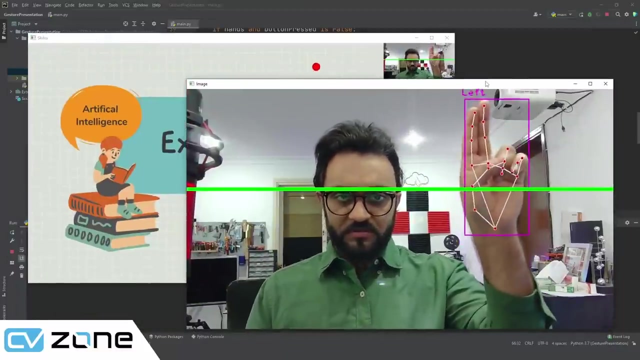 the circle. wait, why is it not drawing at all? uh, if fingers one, one circle, image, current index finger, all of that, yeah, it should draw. so right now it's drawing only when it's above this. so it should draw here. yeah, there you go, so you can see the pointer now. but this is bad because we don't. 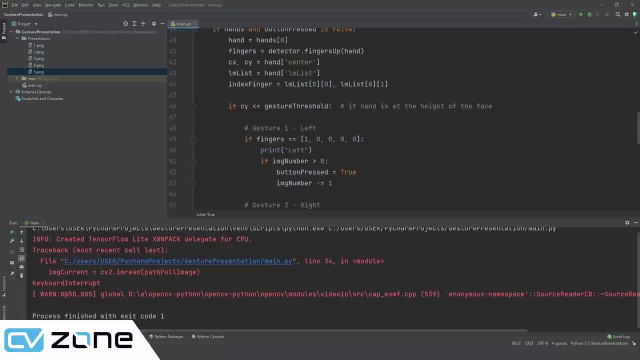 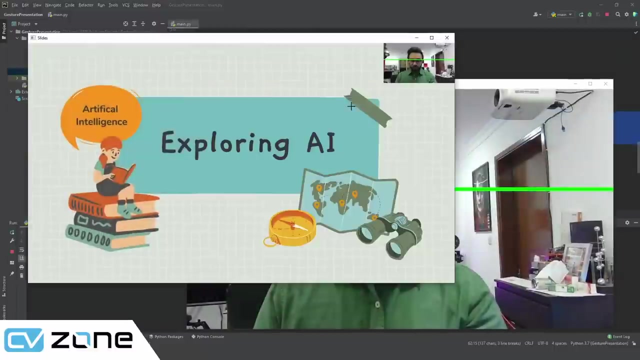 want it to be only when it's above this line. so we will take it out of this uh loop. so here we will go back one step. so the gesture number three is outside this if statement. so let's run that this time around. now you can see wherever we go. 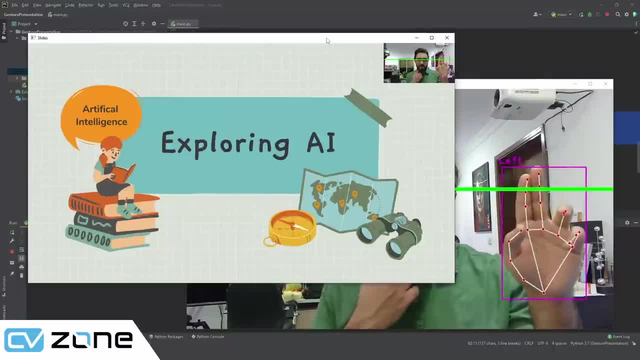 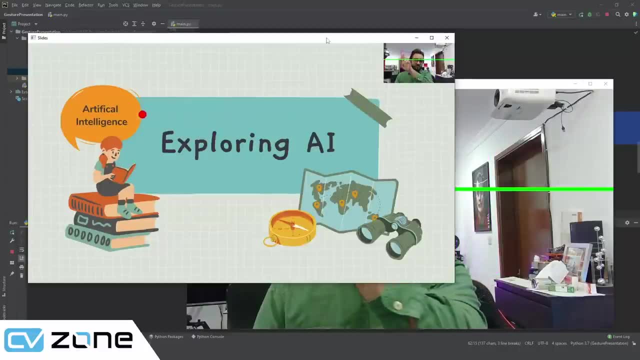 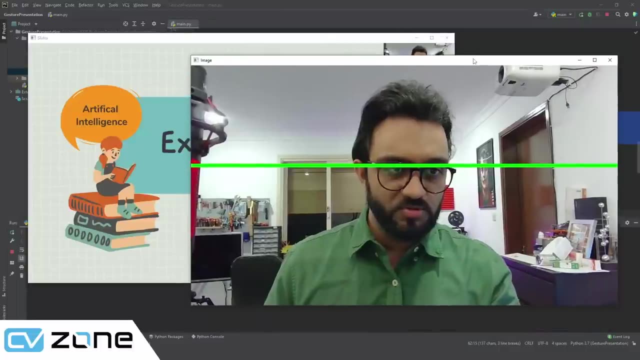 it actually draws it. but here we have an issue. the issue is that if i go to the left, i will have to go all the way to the left to reach that left point, and this is not very easy to do, especially in a presentation. you don't want to go like this. 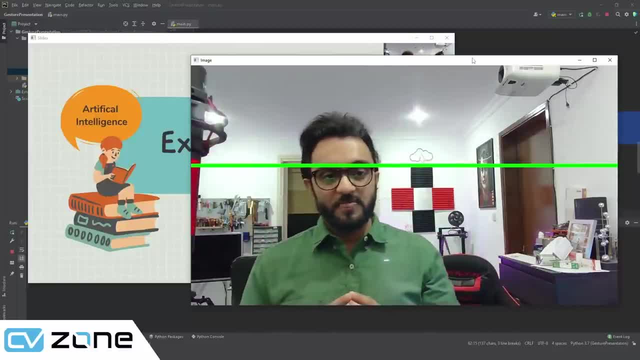 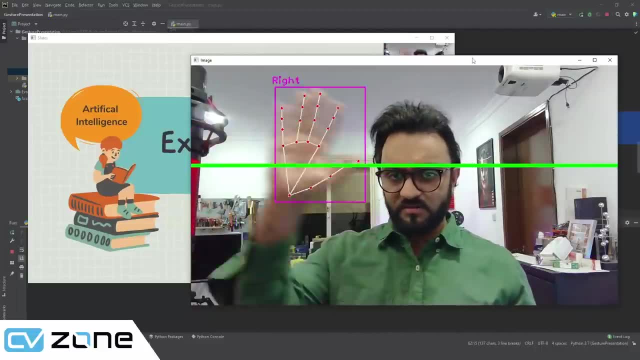 it's just, it's just weird. so what we want to do is we we want to keep it in this area. if i'm using my right hand, it should be in this area. if i'm using my left, it should be in this area. so what we will do is we will limit the values. so we will start from here, from the mid of the image. 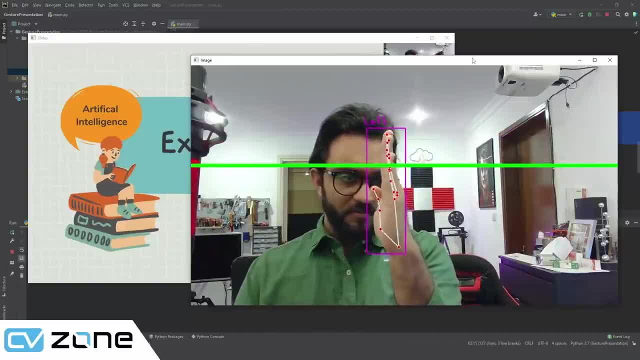 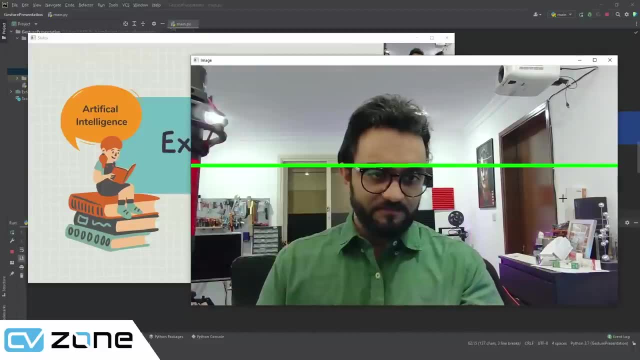 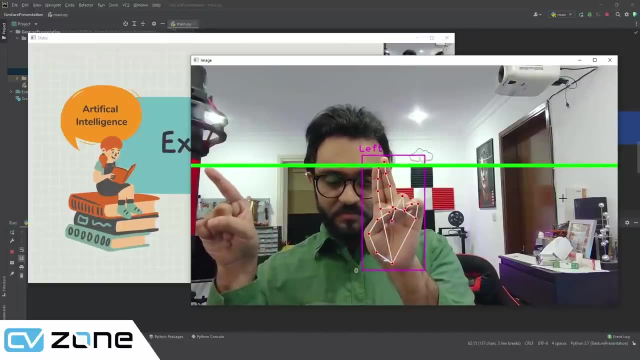 and we will say till the end of the image. so we will use the values of this to scale up to the whole image. so if i'm in the center, if i'm here in the center, so at this point the pointer should be here at the end, right? so this will make it easier to go for us to. 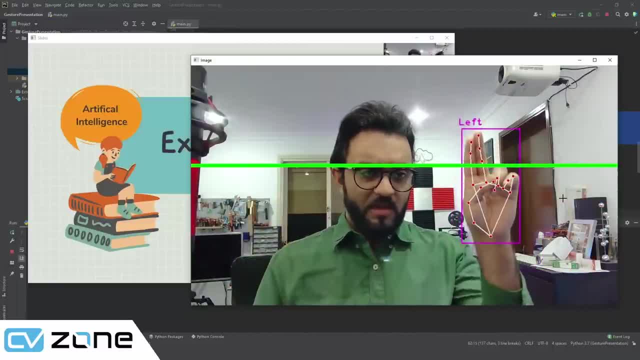 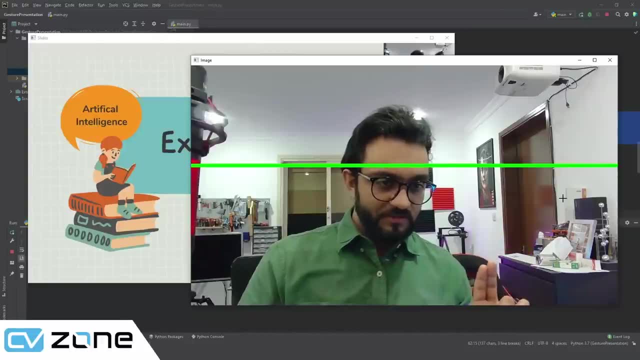 go left and right and then we will do the same for the up and down, because up is easy to go and it will be fine. but if you go down, you see the detection is going down and we will go up and down. bad, the detection is shaky, so we don't want to go till the end, so we will have 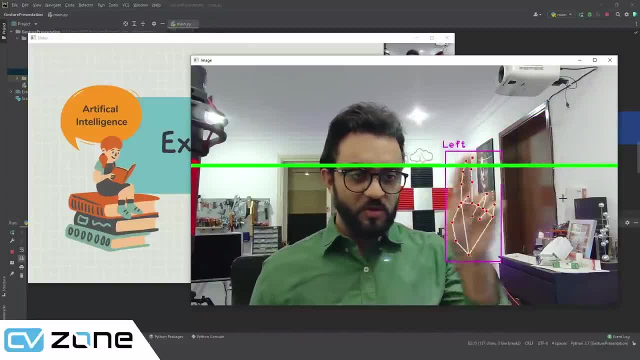 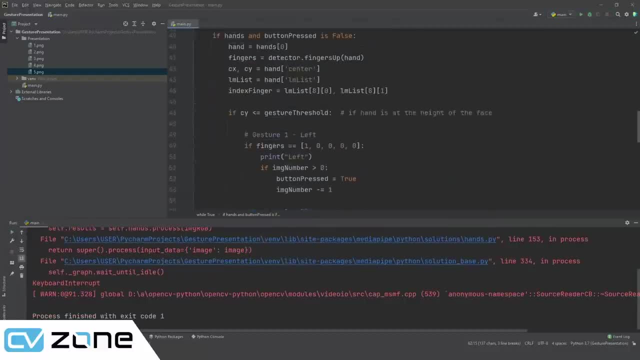 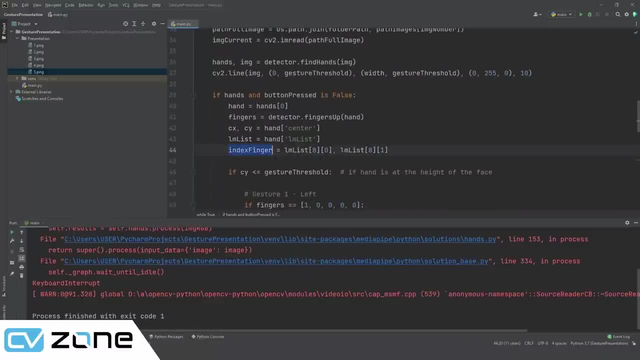 let's say this region in which we will go left and right and up and down. so we will constrain that region. so, to do that, what we will do is we will constrain our value once we get it over here. so this is the index finger, so we are going to. 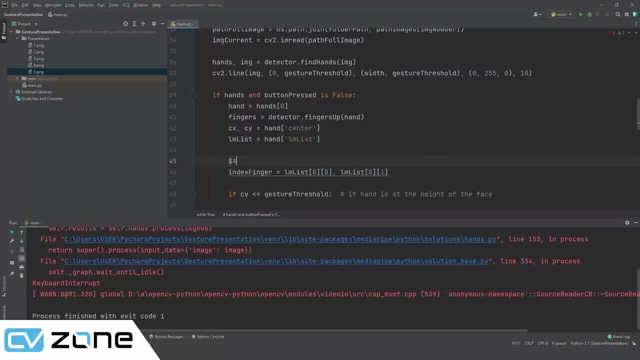 constrain it here. so let's write here: constrain values. for easier. let's say: drawing: okay. so what we will do is, once we have this index finger value, or should be, okay, let's. let's do one thing. we will write here: X value, X value equals. so what are we going to do? we are going to use numpy, so numpy has 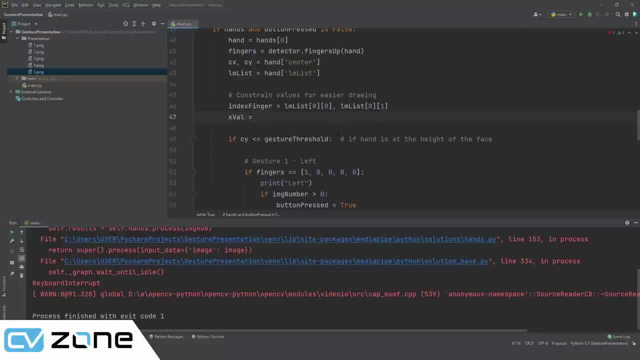 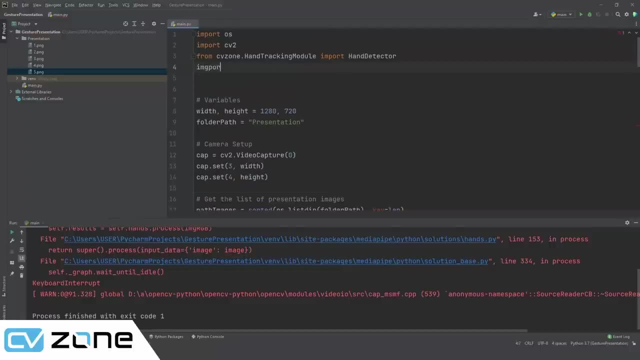 a function that basically allows you to go from one range to another range, so it converts that. otherwise you can use basic mathematics to do that as well, but here we will use numpy, so imports numpy as NP, and then we will go down and we will write that NP dot interp. 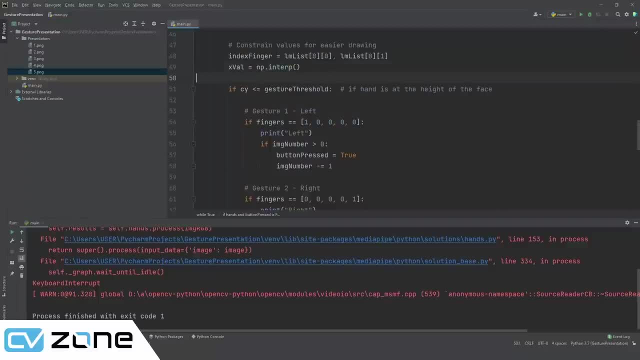 so which value do we want to change? we want to change this value. so: LM 8: 0, so this is the X value. we want to change this value. so the range of this value should be from width: width of the image divided by 2, so this will be the. 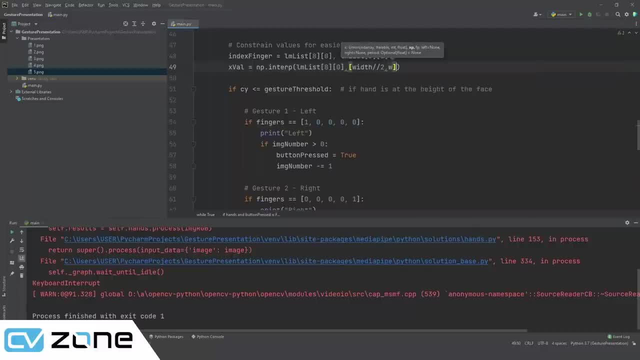 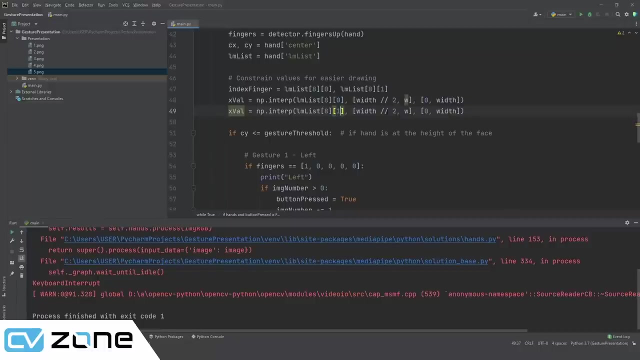 halfway, so starting from there till the end of the image. so change this value to 0 to the total width. so we will do the same thing to our Y. so for the Y, as I mentioned, we just we don't need to do half, we can remove a few pixels from. 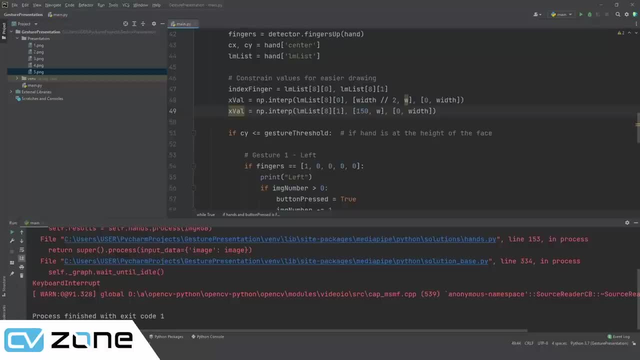 the top. let's say we remove 150 pixels from the top and then we remove 150 pixels from the height for the Y, so we need to add 50 pixels to the next stage from the bottom. so that's it. and then 0 to height. so this will be the value of. 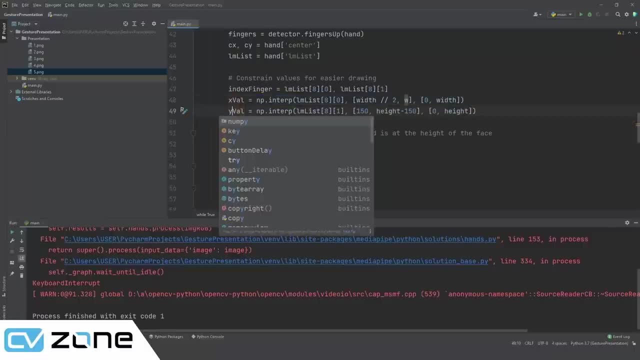 our X and Y, so let's put this as Y and yeah. so the output of this function is not integer, so we need to convert it into integer so that it doesn't give us an error. there you go. so if you didn't get this, basically what we are doing, we 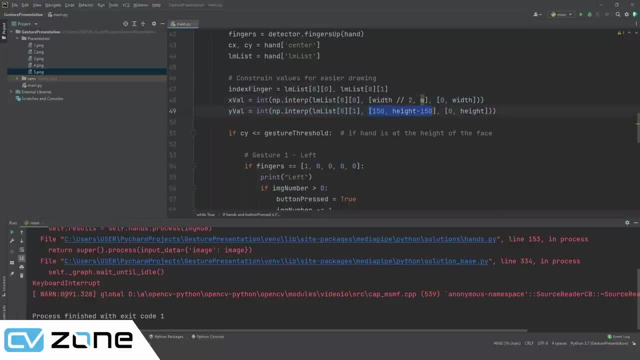 are converting one range to another range, and which value are we converting? we are converting this value, so that's pretty much it. we can remove this, or do we need it? yeah, instead of writing that, then we can write: index index finger equals X Val and then Y Val. 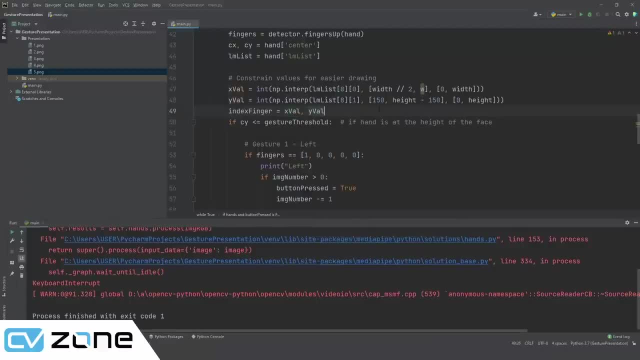 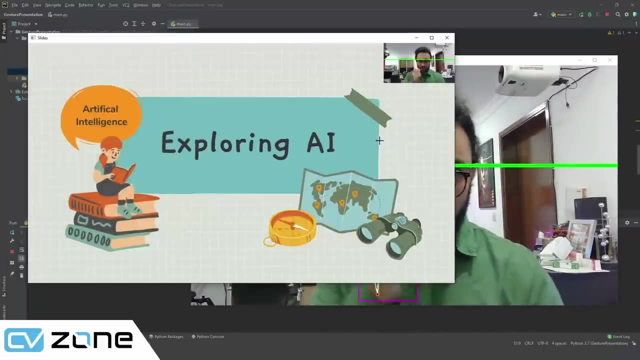 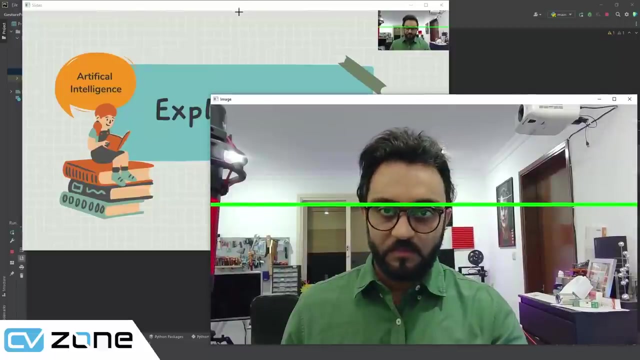 the A here is small. okay, so now it will automatically convert everything over here, and then it will be easier for us to move around. so have a look at this. I will try to put it here on the side. there you go. okay, so I'm on the right. 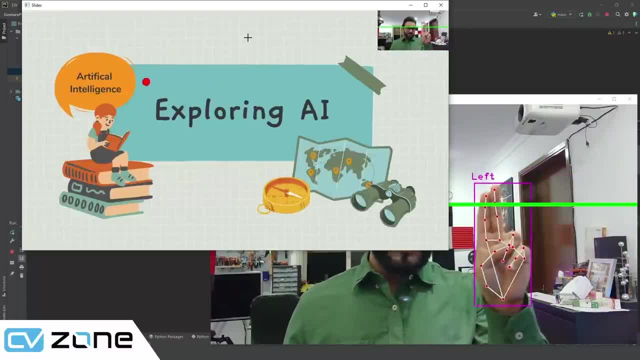 side now and I have two fingers up, so if I go till the middle, you can see it goes to the end. so that's perfect if I go to the right and then I go to the left and then I go to the right and then I go to the right. 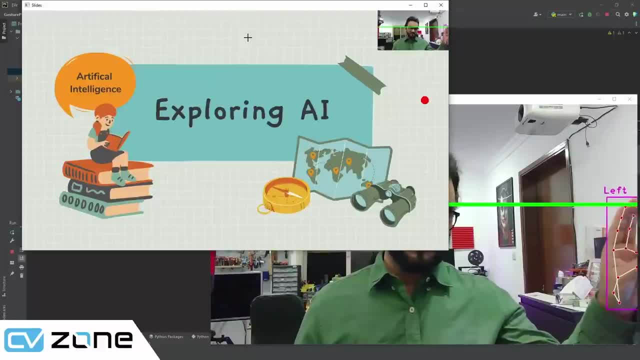 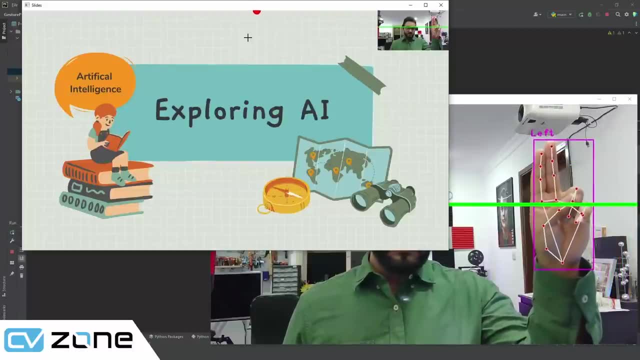 at the end it goes to the right. so kind of right, so you can. you can remove some width from here as well if you want more room. and then the height. if I go up you can see I'm not at the end, but it's the pointer is at the end, so that's good and 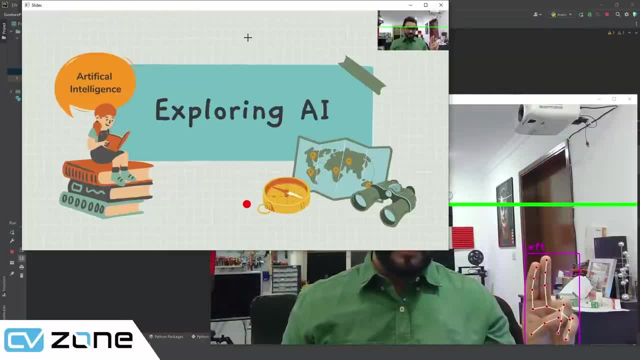 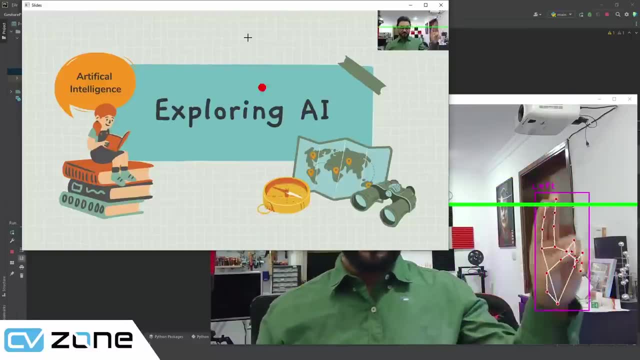 if I go down you can see the pointer is not at the end, but it is almost at the end on the image. so now I have this playing area where I can move this pointer. so this way it will be easier. we don't have to go all the way there. 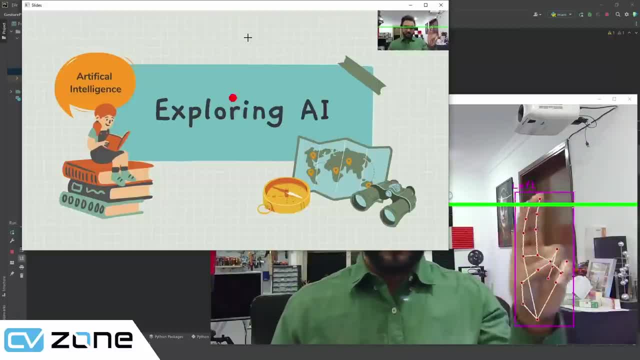 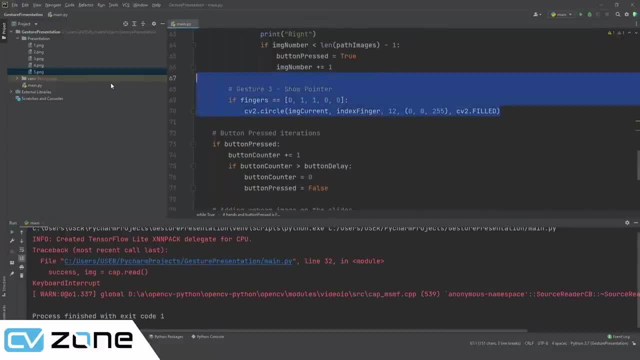 which is quite awkward position. so here we can move around and we can display. so the next step is to actually draw. so right now we are showing the pointer. the next step will be to draw. so here this will be just your number for draw. so the drawing one will be when we have only the index finger, so when we have the. 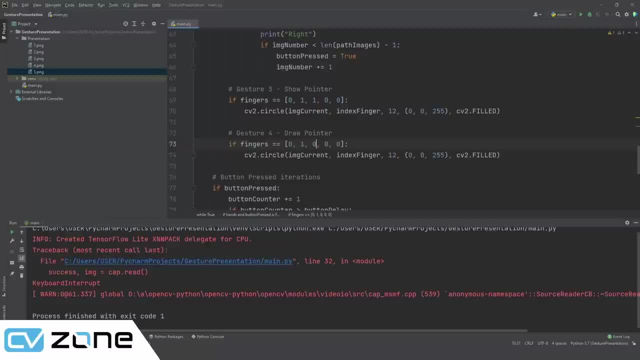 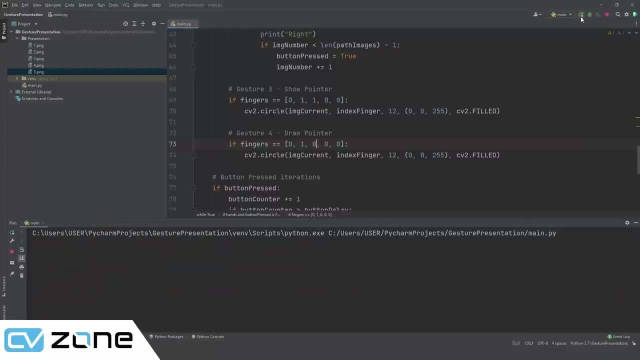 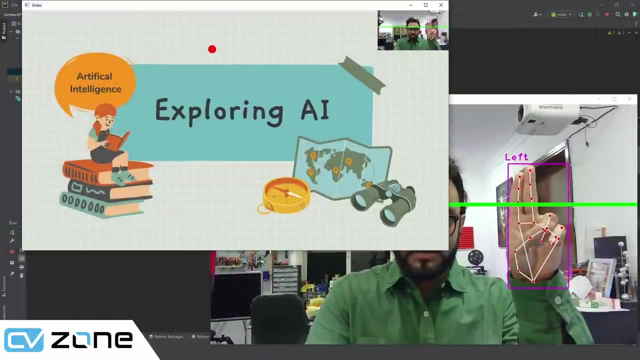 index finger we are going to draw. so this is basically the idea, and then you will see that if we run it now, nothing will change actually, because it will be exactly the same. so if I have one finger or two fingers, nothing is changing. it's just drawing a circle and that's it. so what? 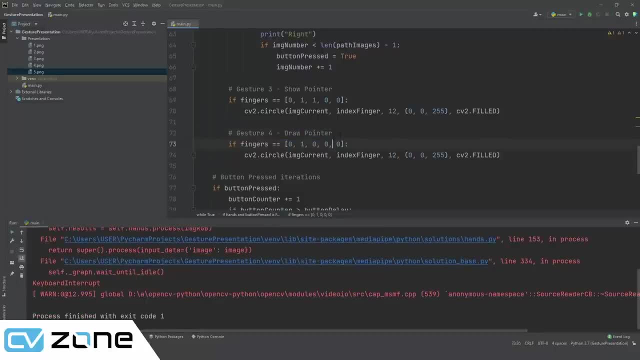 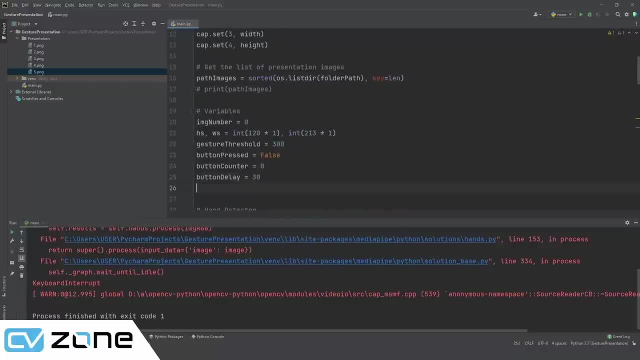 difference does it make when we want to draw? so, for drawing, what we will do is we will create a list and this list we are going to call annotation and notations. so this will be an empty list and whenever we have a new point, whenever we raised only the index finger, whenever we want to draw, we will append. 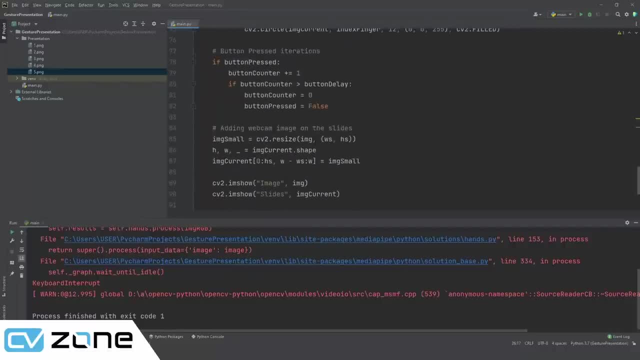 this annotations file, sorry, annotations list. so here what we will do is we will say annotations, dot append, and we want to append the index finger and down here we are going to draw all the annotations. so here we can simply say: for annotation in annotations we are going to draw a line, so we are going to. 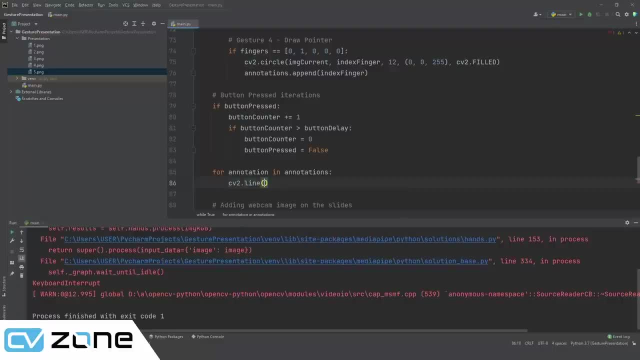 write cv2 dot line and we will draw it on our image current and then we will draw it, we will write annotation. actually we will need the iteration number. so we will write here I and we will write here enumerate, enumerate, there you go, and we will say annotations at 0 or at I and then annotations I minus 1. so 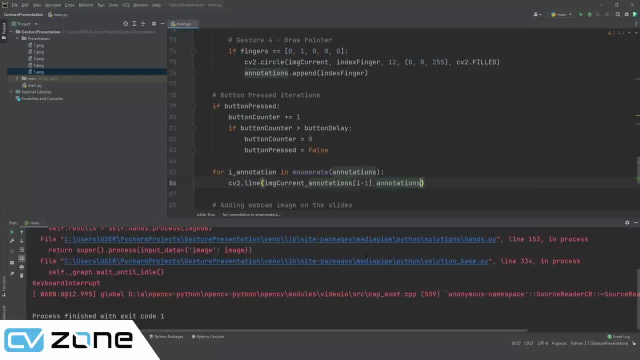 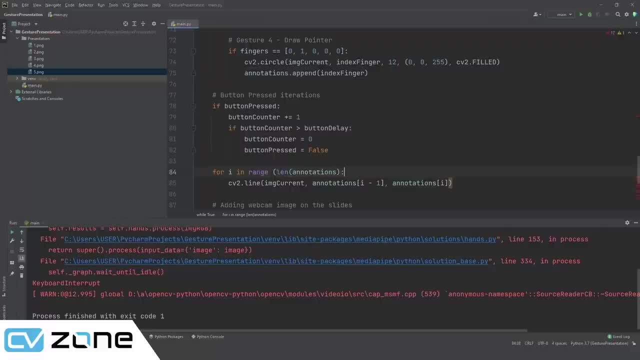 in range of length. we can write it like this: so this is fine. basically what we are doing is we are saying that take all the points and draw lines between these points. so here we will say that the color of the line should be 0, 0 and 200, 200, and then the size is 12, the thickness. 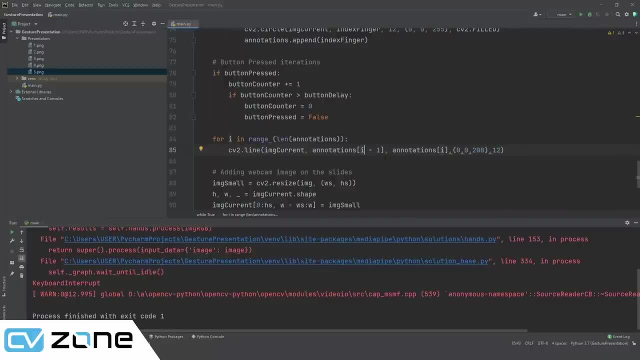 but the issue here is that right now, if I run it, it will give an error because the the first value will be 0, so 0 minus 1 will give us minus 1. so there is no point minus 1. so we have to write if we will draw the lines, only if. 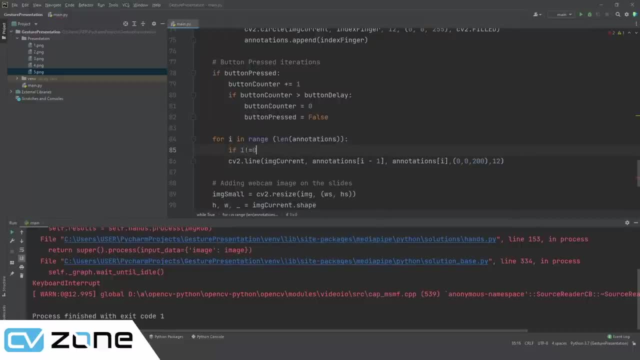 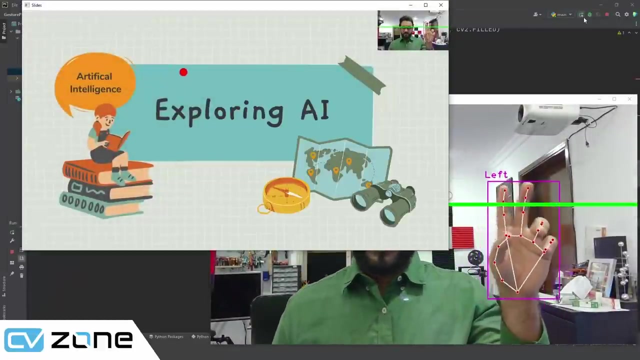 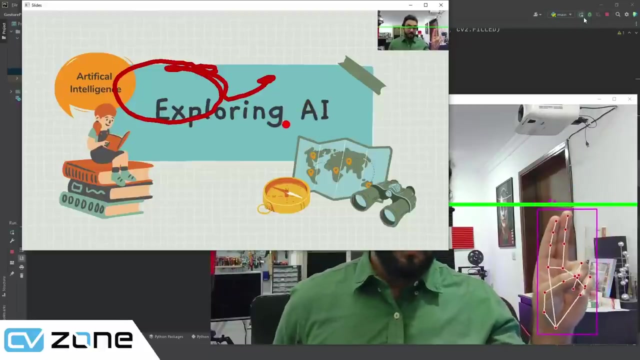 I is not equals to 0. I is not equal to 0. so if that is the case, then we are going to draw, so let's run that. so here, if we have one finger, you can see, it started to draw. if you put two fingers, it doesn't draw. but now you are going to see a big 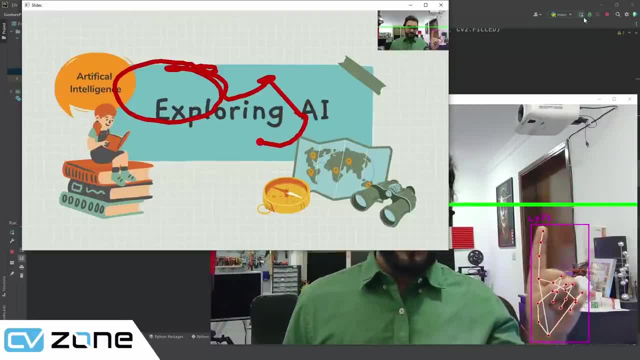 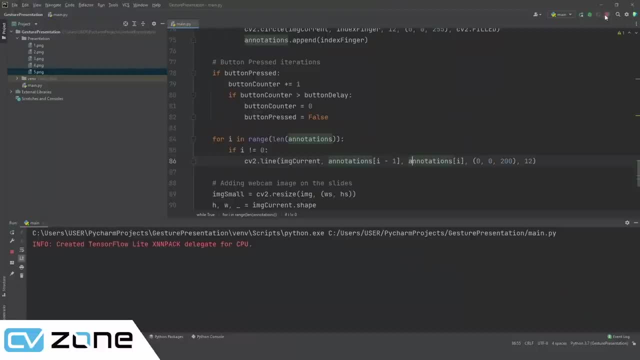 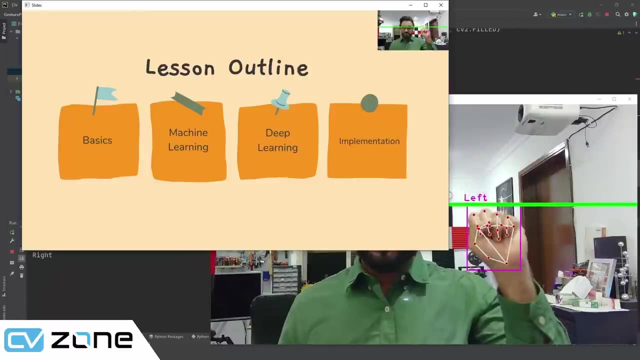 problem. if I put my finger down you can see, it creates a line between the previous annotation and this annotation. so let's say I was drawing, I was pinpointing something. let's say I will go to the next one, and here I have these four of them. so what I'm doing is I'm 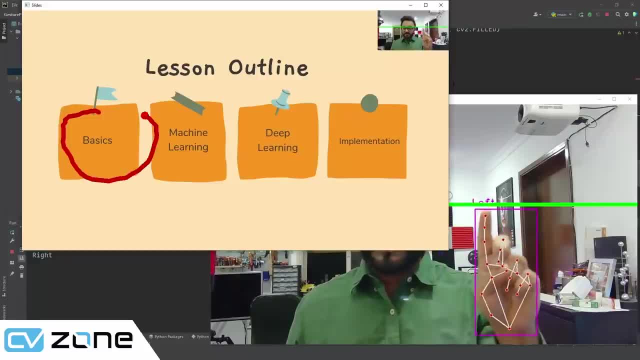 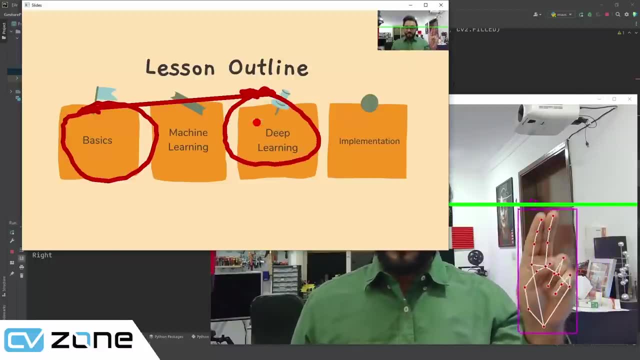 pinpointing the basics. so I will draw the basics. I will say these are my basics, and then I'm talking about deep learning. so I will draw on the deep learning. but you can see now there is a line between that and that's not good. it doesn't look normal and if I drew another one it will. 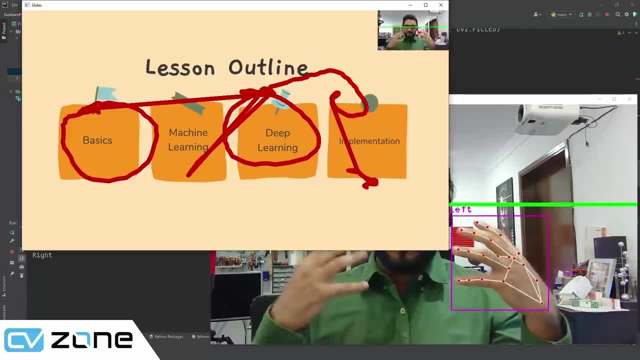 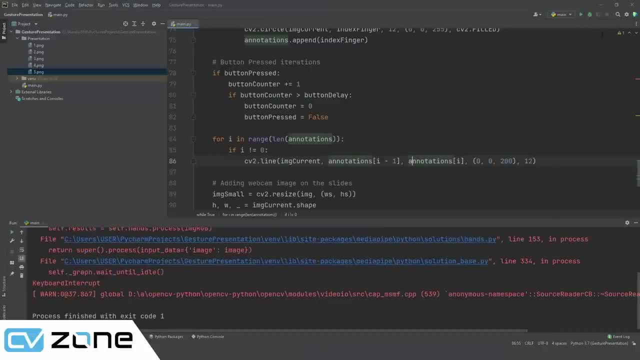 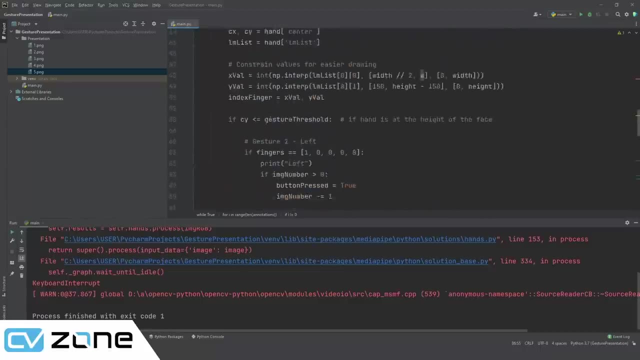 start again from that point. so it it doesn't recognize the difference between different annotations. so this is a problem. so how can we fix this? we can fix this by creating a list within a list. so in this annotations we are going to create another list of annotations. 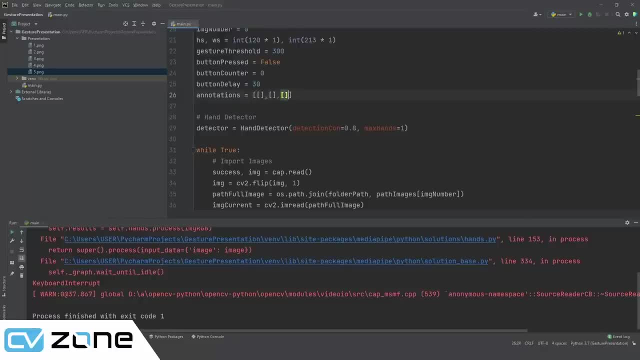 so each one of these will be like that, so it will have multiple points. so let's say five and ten, and then it will have twenty and thirty. so this here is one annotation. this here will be a different annotation. this here will be a different annotation, so each one will be different and it will treat it as different. so 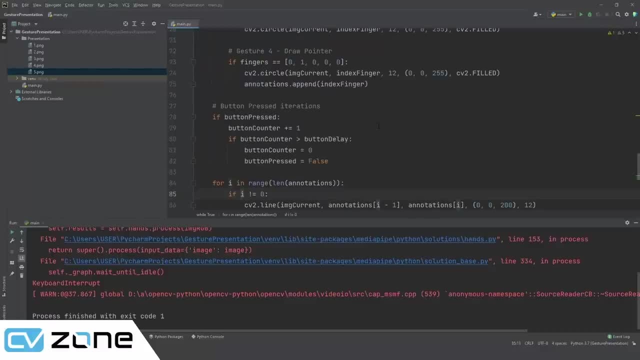 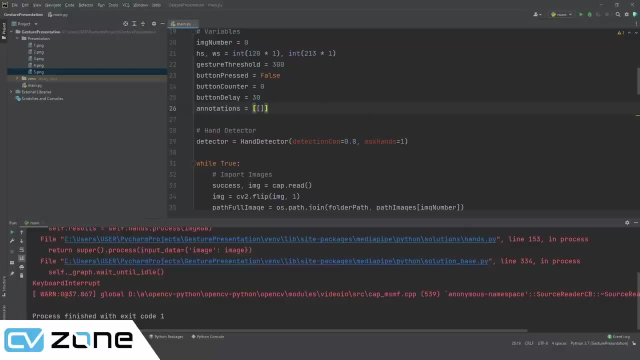 let's write it down again. it will be empty. so now we pick one annotation and let's give it a name. because we did so here, we will go back within the operation one. we need to define an annotation Number and then we need to edit that annotation as the nodetation number and 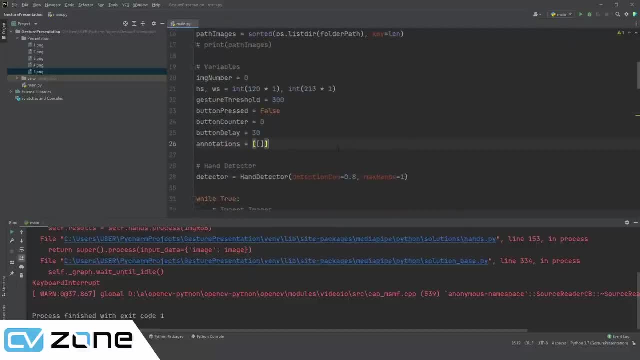 according to the message that we will send to the system, we will write it a list within the list. so that's our annotations, but then we will have to make some changes. first of all, we need to define an annotation number. so whenever we annotate, we will give it an annotation number, and once the annotation is complete, then you have to do new requirements under projectатmallcom and after that you have to go to the next one so that we can, so you can update, we can add another one. so the first annotation will be zero and then this annotation will be flied up. 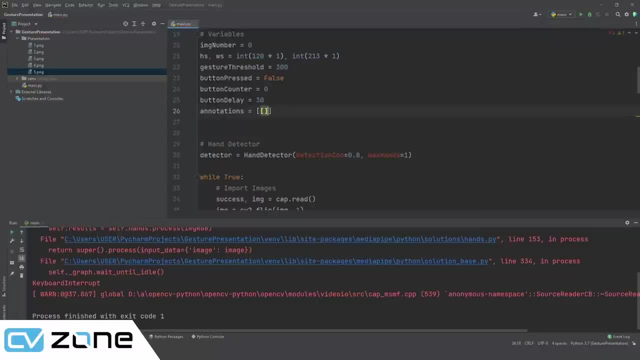 the second one will be 1, then 2, and so on. So here we will write: annotation number equals. we will start from minus 1, so the first one will become 0 when we add it. I will I will explain later on. Okay, this is annotation number, and then: 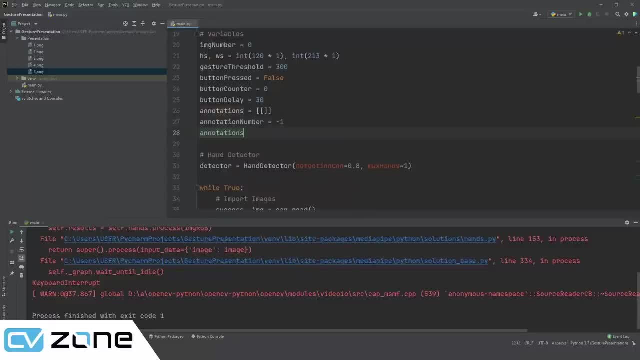 we need to give a flag called annotation start. So in the beginning we will keep it as false. So whenever we start we need to know the starting and the ending point of the annotation so that we can separate these lists inside this list dieser lans talents- erwart's singers. 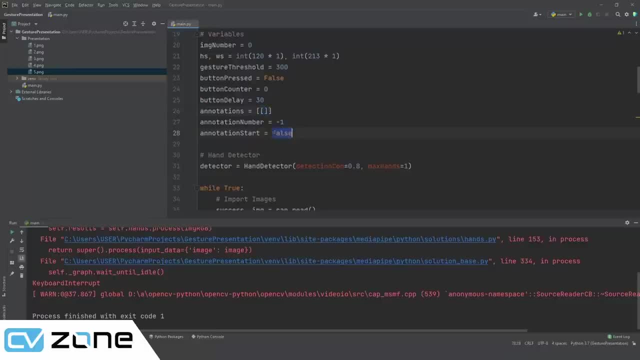 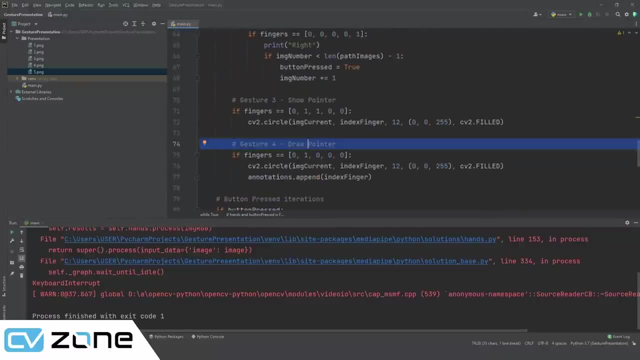 eleven in our relational table, here, wandering. So in the annotation start. initially it will be false. and whenever we put on one finger it will become true. So whenever. So whenever we have the first春이, it will become true. So, whenever we have the index, whenever we have the draw pointer, it will become true. So here we 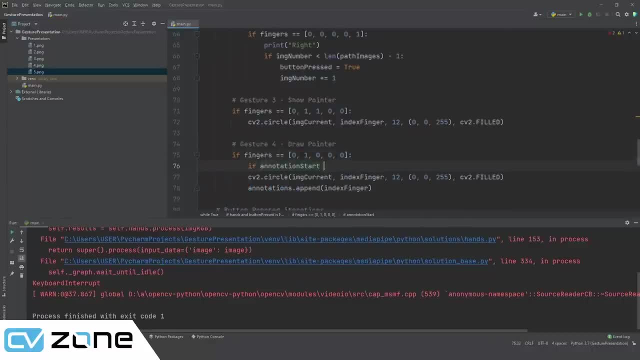 will write: if annotation start is false, then annotation start: come on, start. why is it not writing: start is true. Okay, so now, whenever it is false, for the first time, it will make it true, and once it makes it true, then we are going to start. 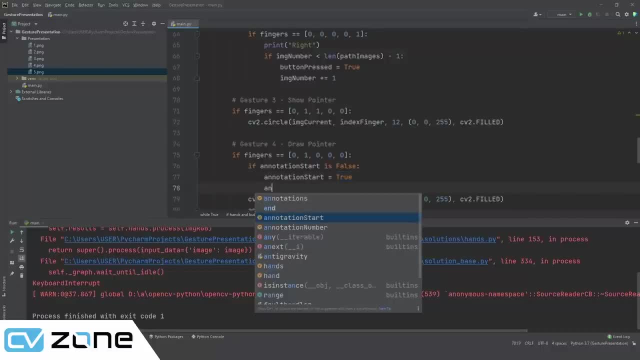 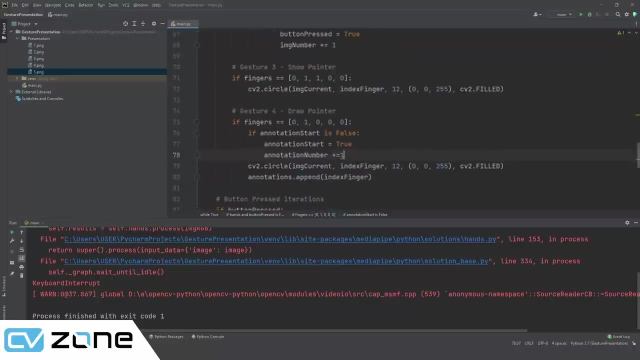 our process. The first thing we will do: we will increase the annotation number plus equals 1. so it was minus 1, it will become 0. When it was, when it will be 1, it will become 2.. When it's 3, it will become 4.. So this is the idea. so it will. 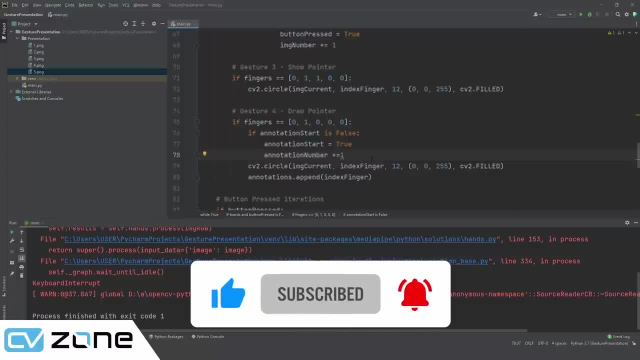 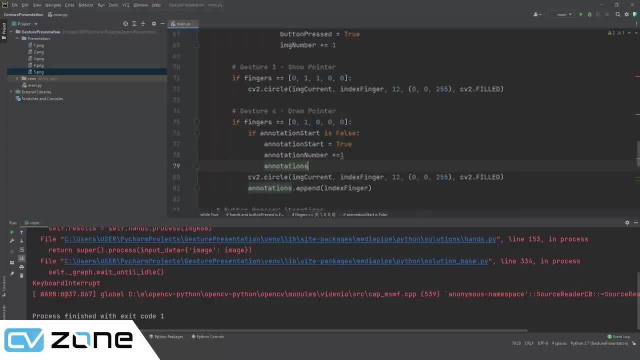 become plus 1 and then what we will do is we will append an empty list. So here we are going to write annotations, dot append, and we will append an empty list. so in this list we are going to keep adding the points. so that's how it will. 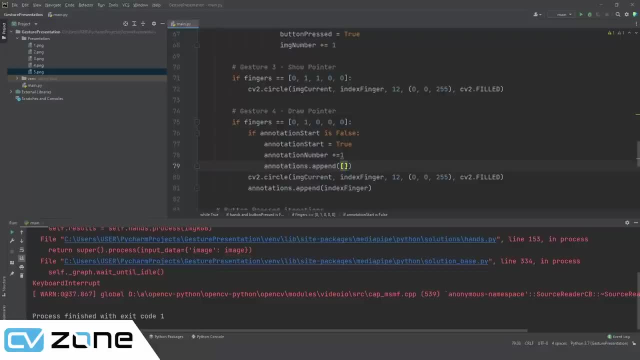 work. If we don't add this list list, it will give us an error because we are directly going to tell it to put it in list number zero. so what do I mean by that? so here in annotations we were simply saying append index finger. but this time we cannot say that. we will say: in annotations there is a list, that list is. 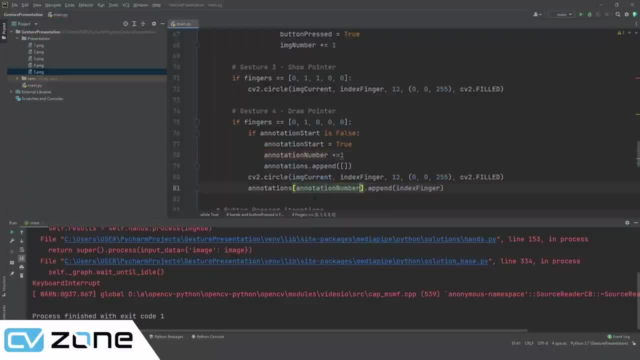 basically annotation number. in that annotation number list, append index finger. so right now we are directly calling that list. if we don't write this, there will be no list to call and it will give us an error. so we need to add this empty list. so here, until it is true, it will keep adding to. 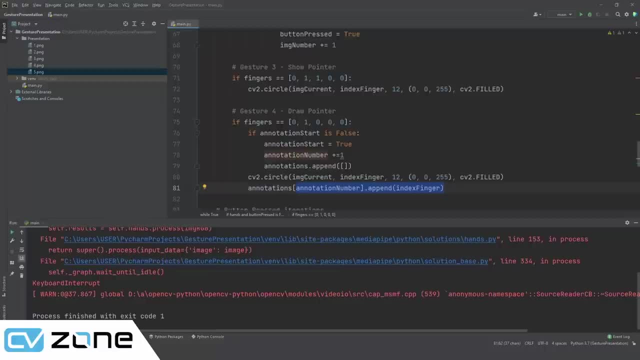 this. once it becomes false, then it will become true again and it will add to this list. so next time it will not add to this list. so next time it will not add to this list. so next time it will add to this list, it will add to another list that it has created. so putting it true is correct now. 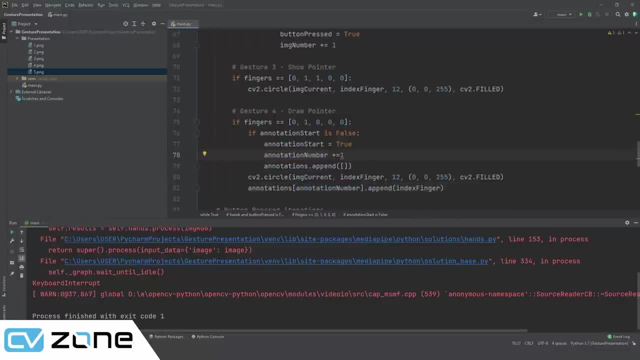 but putting it false. we didn't do that. so when it starts the annotation, we know, but when do we end the annotation? it should end the annotation if the finger is not this, right. if there is any other finger, it should be false, right, so here we can write else: annotation. 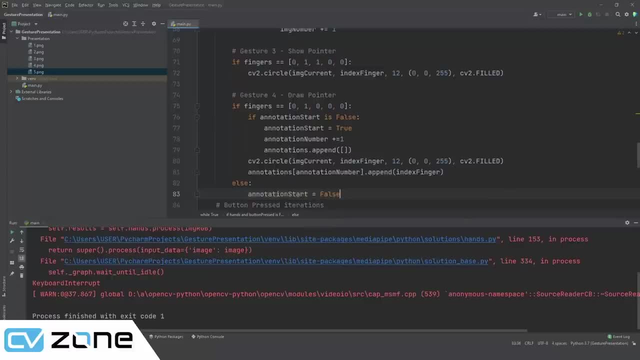 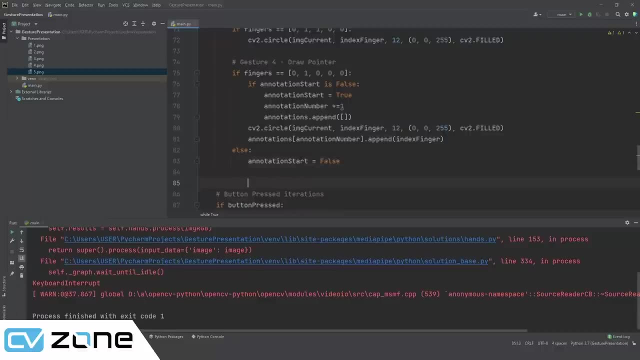 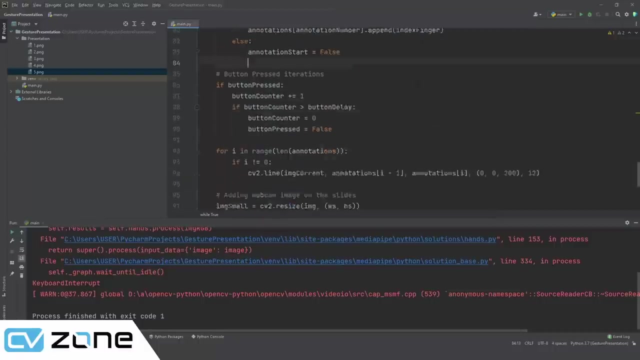 start equals false. so whatever the other one is, it will make it false. so let's try that. and now, now we have multiple lists, but in the drawing we are simply drawing the same thing again. so we cannot do that. so what we will do is we will change the code here a little bit, so in annotations we 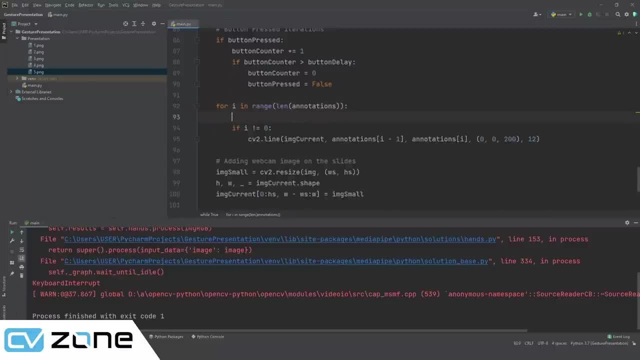 have our annotations, that's good. then we have to put another loop for j in range the length of our, the length of our annotation at i, so it basically will loop through all the points and then we will check if j is not equal to zero. if j is not equal to zero, then we will check if j is not equal to zero. 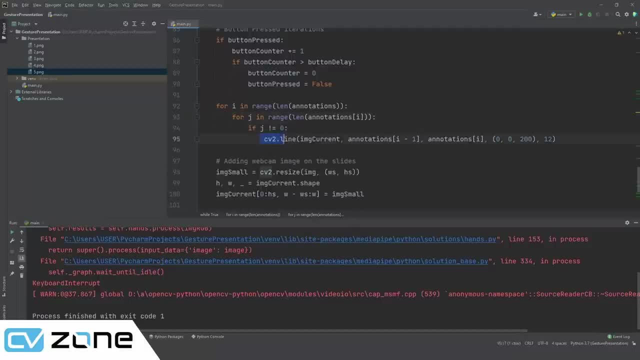 if j is not equal to zero, then it will draw this, but this time around it will not draw from annotations. uh, actually we do need that because it's not from annotations. or we can write here: annotations i and we can write here: annotations i, and then this will be. 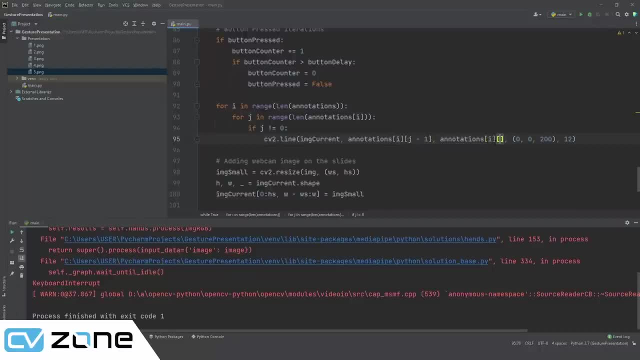 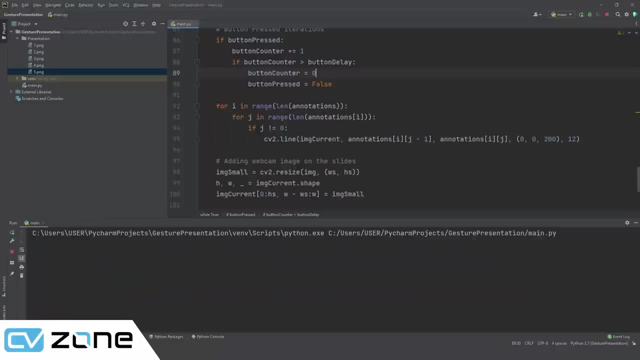 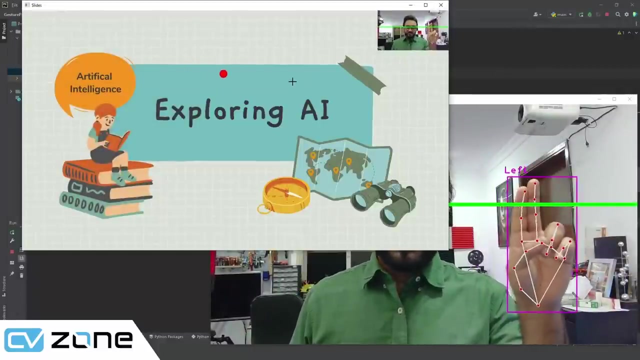 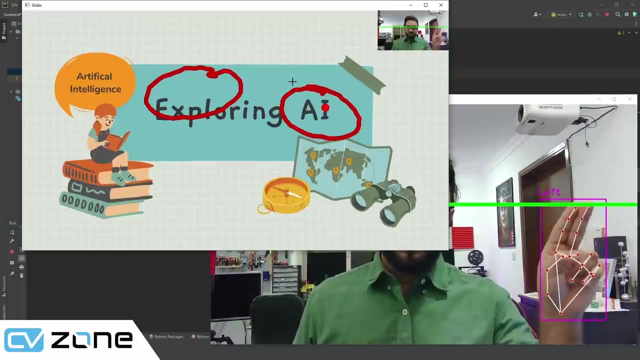 j minus one, and this will be j. there you go. so yeah, now it should, uh, work as expected. let's go ahead and try it out. there you go. so here we have two fingers, and then we put one and we create a circle, we close, and then we go to the other one and we create another circle. there you go. perfect, so now we 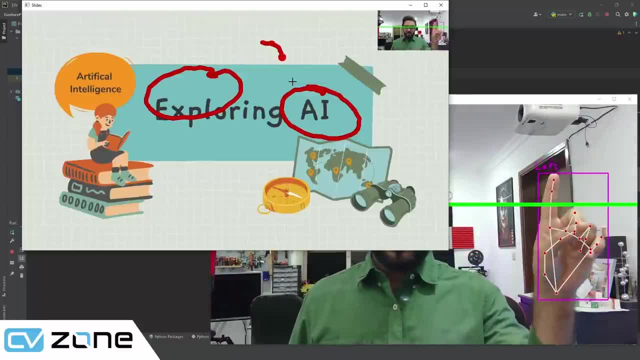 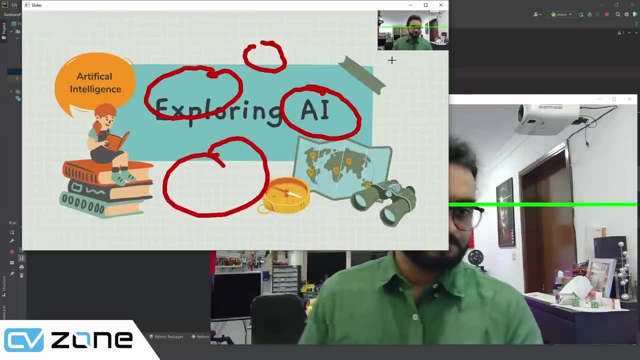 can have different ones, and if we go back, we start drawing. so if we go back, we start drawing and we can close, and we can start drawing, and we can close and we can start drawing. there you go now, it is perfect. there you go now, it is perfect. 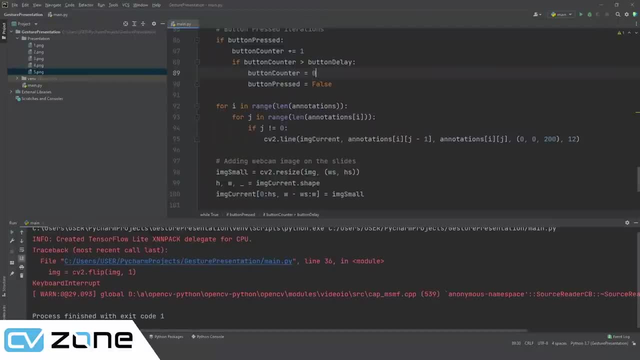 there you go. now it is perfect. so this is good. so this is good, so this is good. now one more thing that we can do now. one more thing that we can do now. one more thing that we can do. uh wait, did we test? let's test it with. 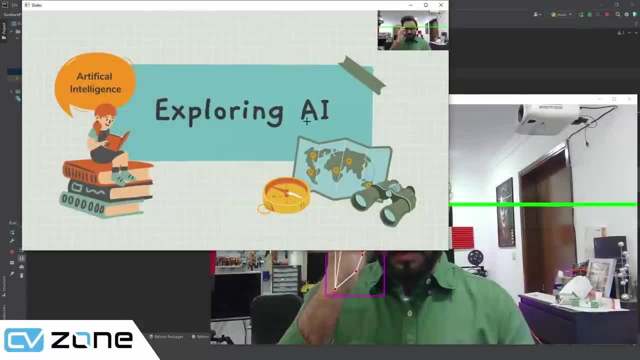 uh wait, did we test? let's test it with. uh wait, did we test? let's test it with the, the, the, with the other gestures. maybe it will with the other gestures, maybe it will with the other gestures. maybe it will give us an error or something. give us an error, or something. 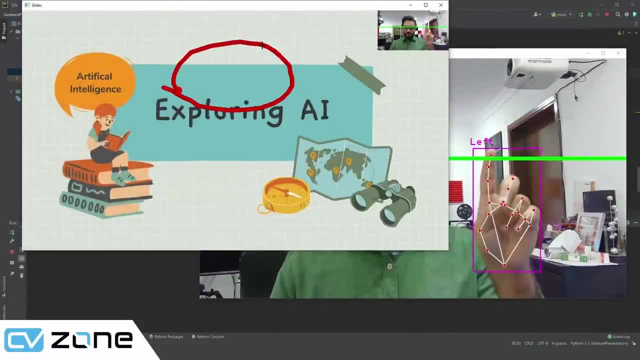 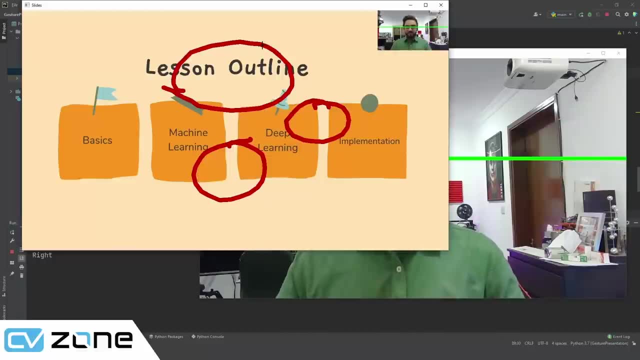 give us an error or something. so let's say: if we draw, so let's say: if we draw, so let's say: if we draw, there you go, there you go and there you go. that's a problem. we go back and we can. we can still draw, we can still draw and it. 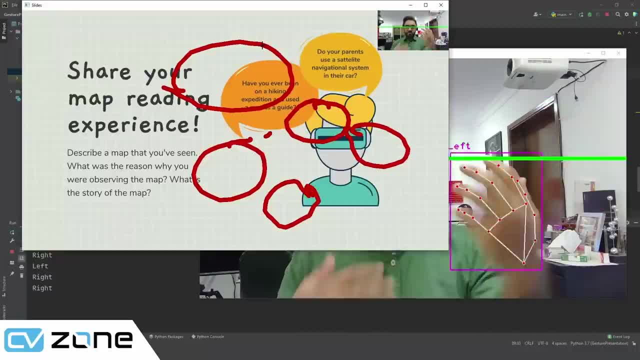 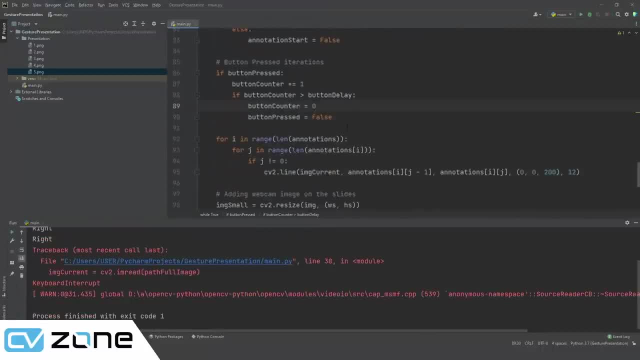 works. but, uh, when we go to the next slide, it should remove all the drawings so that we can draw on the next one. so, whenever, whenever, um, we are going left or right, we need to reset all the drawings. so how can we reset? uh, we can reset by using these three lines of code. annotations are: 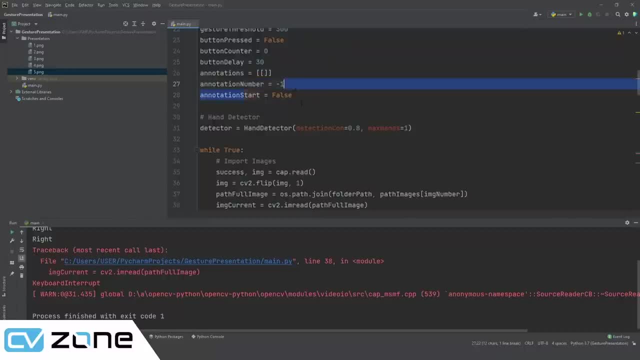 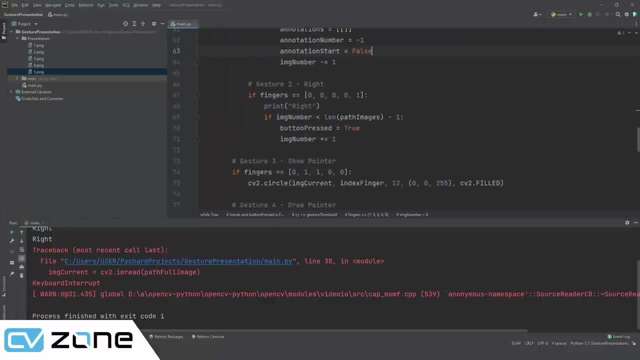 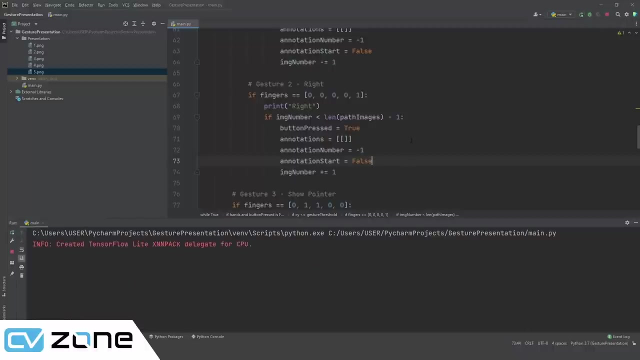 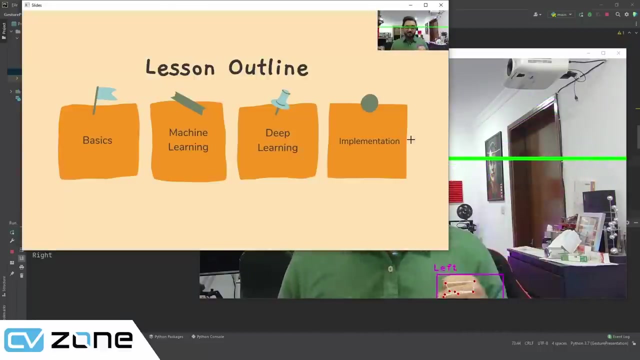 zero. annotation number is minus one. annotation start is false. so we can use these three lines. so here we can paste it like this: there you go. so if we run that- uh, let's see if it works- there you go single double. then we go forward- it's gone. we go backwards: it's gone, so now we can go forward. 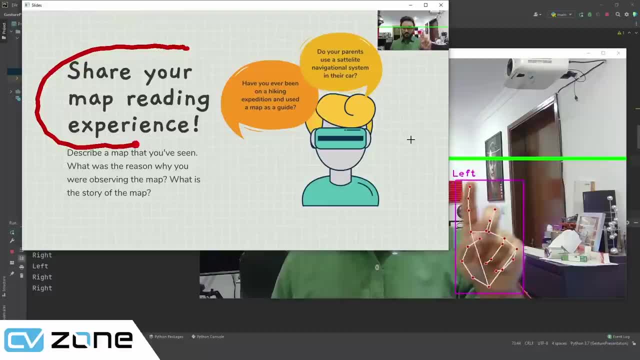 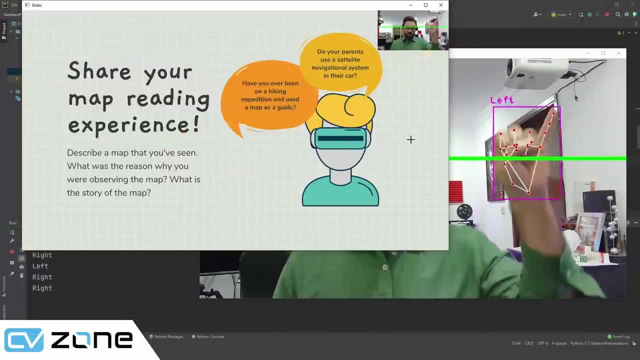 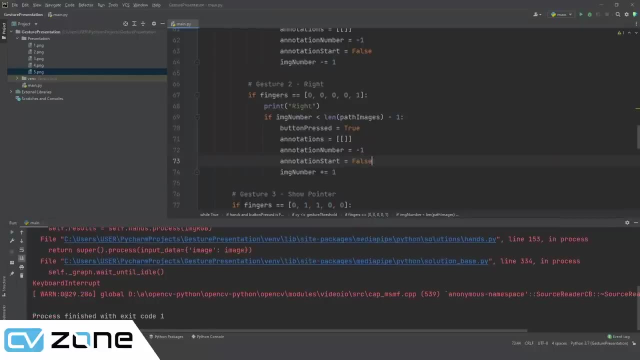 and backwards, and then we can draw. and we can draw multiple- uh, what do you call? points- and then we can go forward and backwards, and it's all good. so that's good now. one last thing we can add is, um, the the erasing. so sometimes we want to erase. 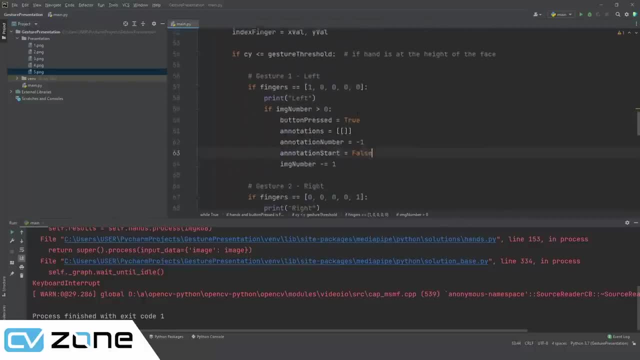 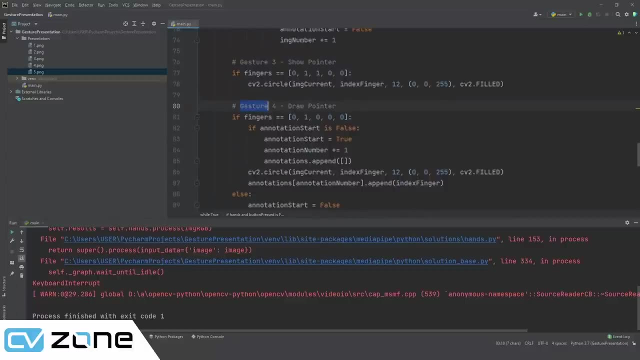 and we did a mistake, so we should have the option of erasing. so here this is gesture number four. so let's add a gesture number five that will allow us to erase. so let's write here: gesture five: erase. so let's say that if fingers are three or four, 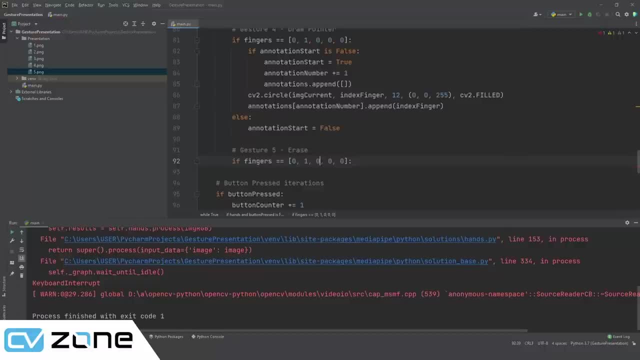 let's put three. it will be more unique. you can add your gesture, whatever you want here. let's just put three. if there are three of them, then we will. um, then we will remove. so first of all we need to check, uh, if the annotations are present. so if there are any, 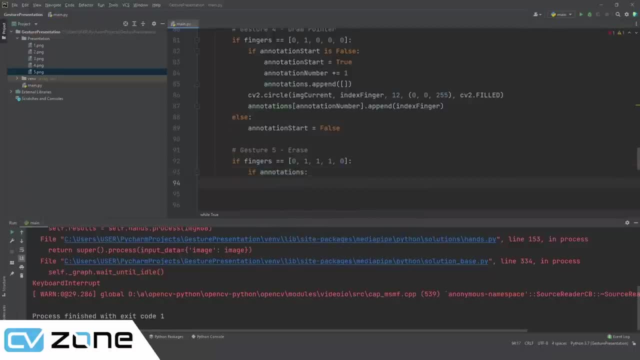 annotations. if it's not empty, then we are going to remove the annotations. annotations: dot pop minus one, so it will remove the last one that you drew and we need to. if you remove the last one, then we need to change the annotation number. uh minus equals one, so whatever the number is go. 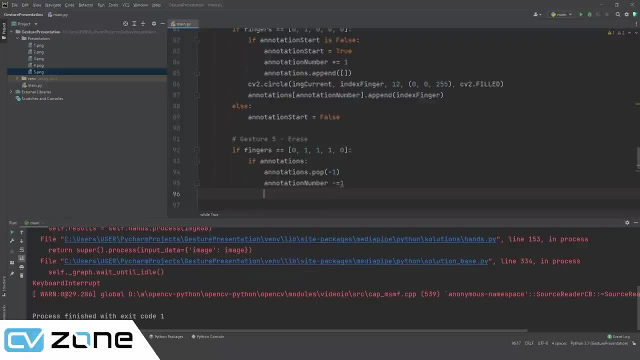 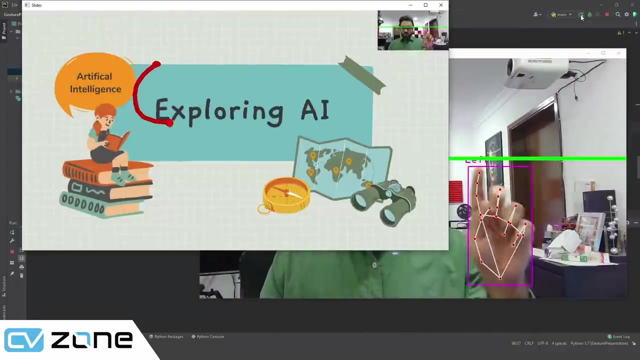 back one one more time. and again we need to add here that we have button pressed, otherwise it will do it so many times that it will be very difficult to work with. so yeah, so this is good, let's run that okay. so let's try this out. so we are drawing, then we draw here, and we draw here. 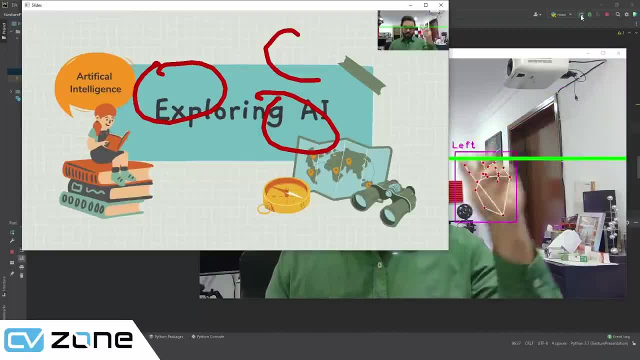 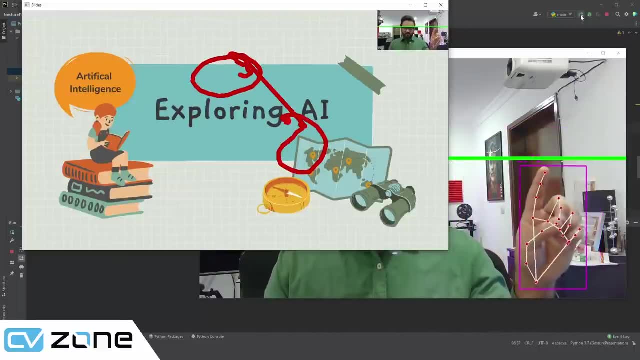 and oh, i made a mistake. i'll do this and it will erase, erase, erase, erase. so as many as you want you can erase. oh, what happened there? it actually went all the way here. the annotation number was the same. uh, it didn't change the annotation number. why is that? 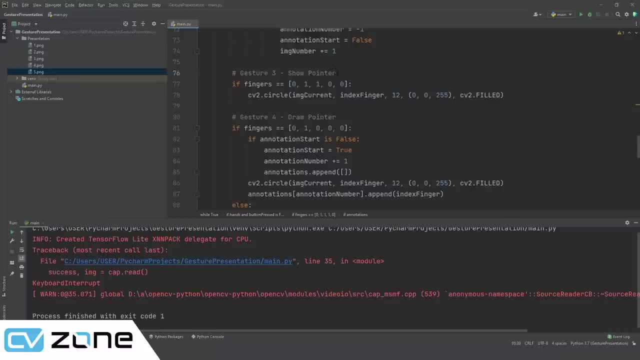 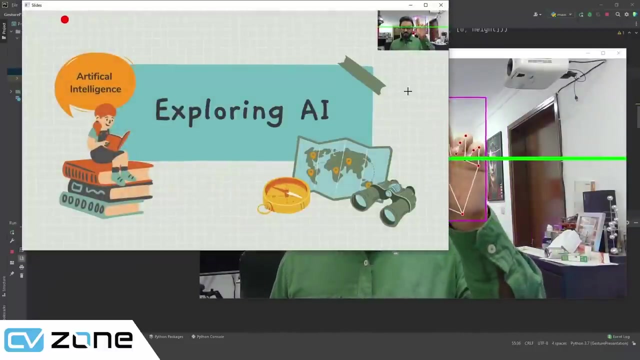 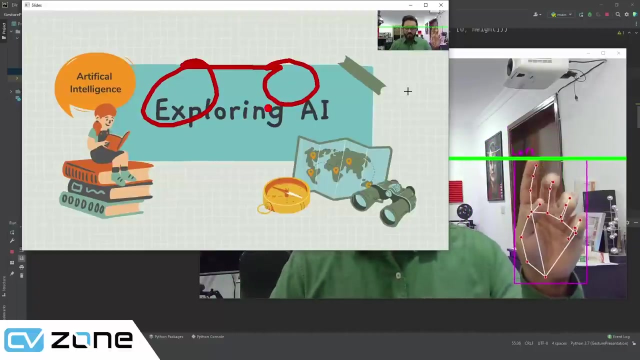 so if we have the pointer here, show pointer, okay, let's do one thing we can put here if it's show pointer, annotation is false. and then, uh, if any of these annotation is also false, just to make sure, so let's try that again. so here we create a circle. we still have that issue. why is that? 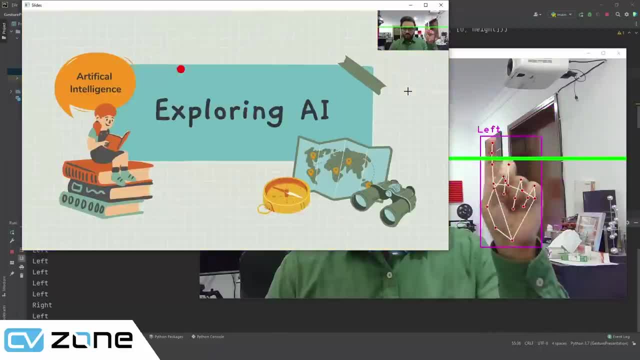 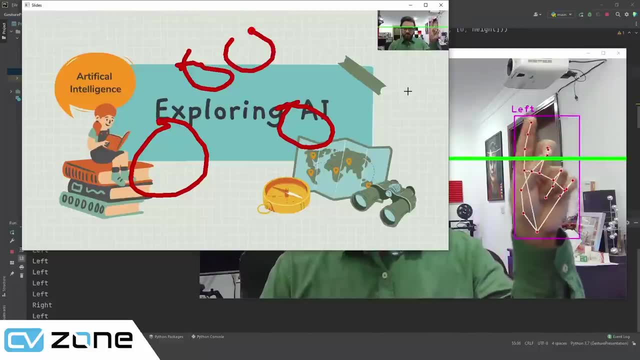 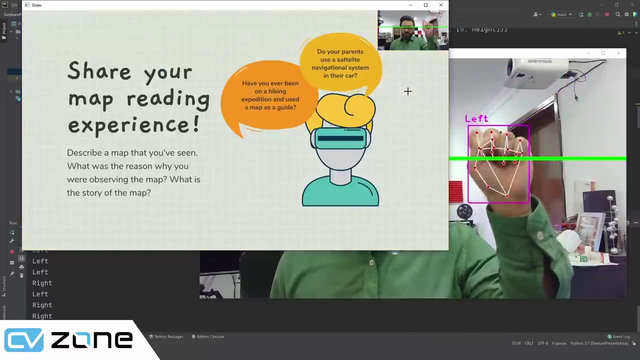 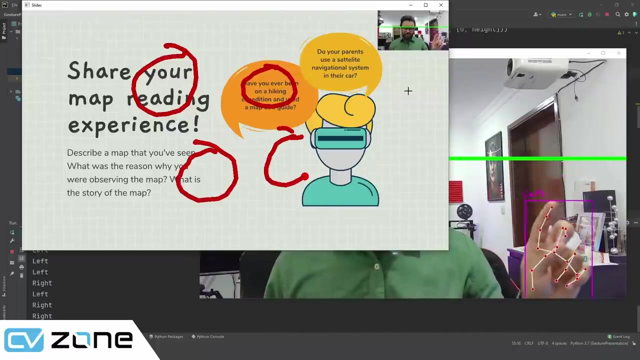 earlier it was working fine. so let's go forward backwards and we are drawing, we are drawing. so sometimes it's working, sometimes it's not. not sure what the problem is. let's go forward, forward, forward and let's draw again. so it happens at a very specific point. not sure what that point is, though. 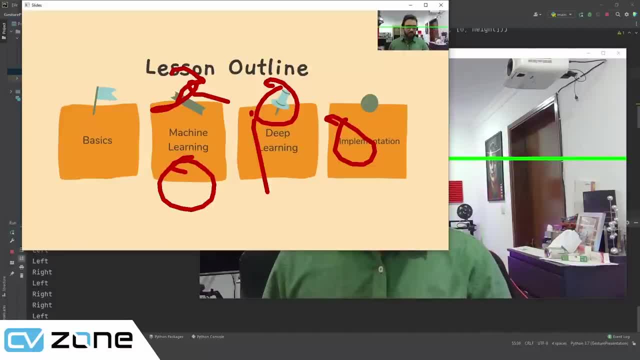 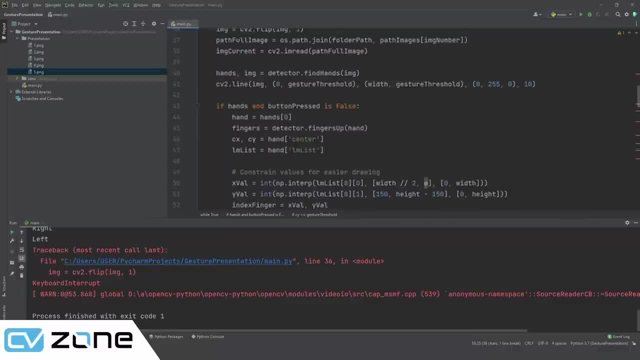 seems fine to me. now, where else can we add this annotation: start is false if this is pressed, or maybe when the hand is lost? oh yeah, that could be a possibility. so if, if both of them are false- um yeah, we can put an else here as well. 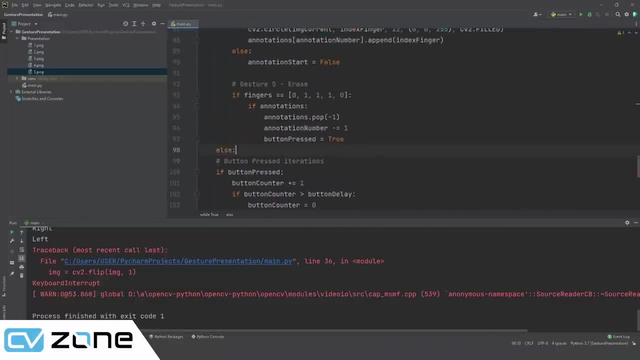 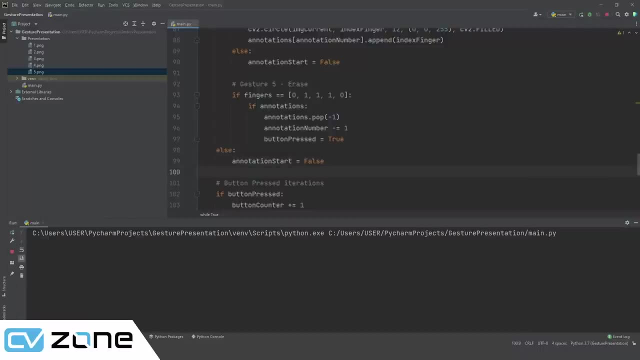 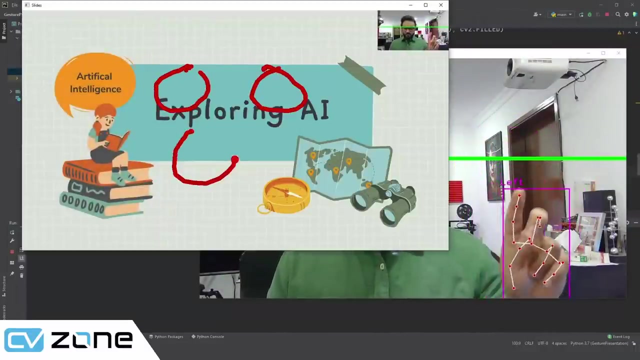 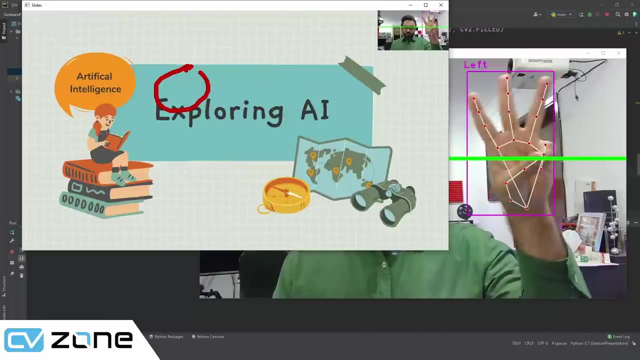 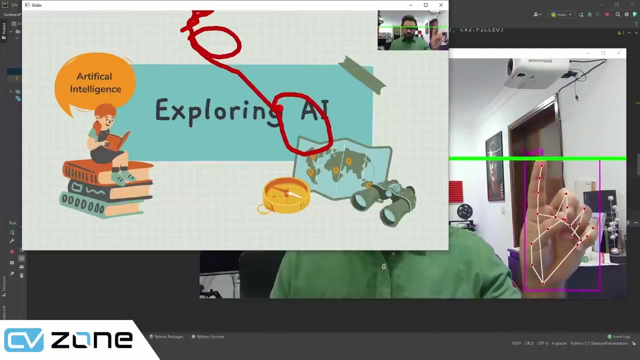 and this is gesture five. so here we can write else and then we can add this annotation: start is false, so let's try that. hopefully this will solve the problem. uh, let's try to draw and then draw, draw, draw. that worked fine. let's try to draw again. so there you go. then we draw here. still, there is a problem. 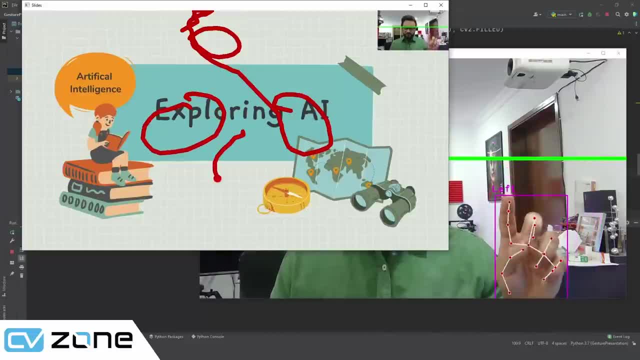 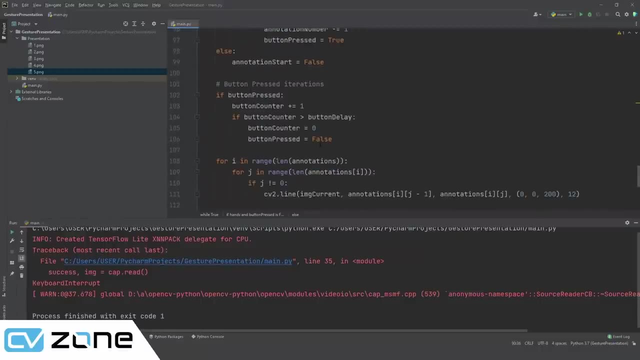 so there you go, then we draw here. still, there is a problem. is it that when it's really fast or what happens, where else can we add? this button is pressed, So annotation start is false as this. Oh, maybe that's the problem, So we need to put this over here. 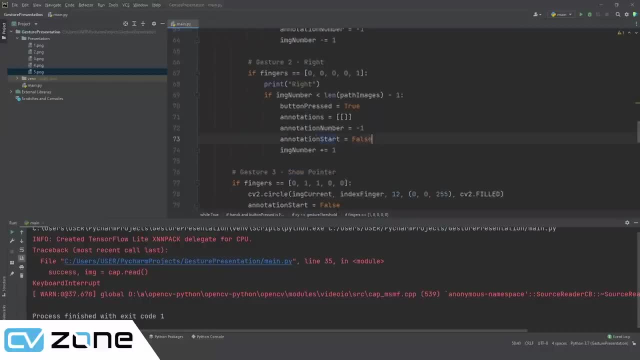 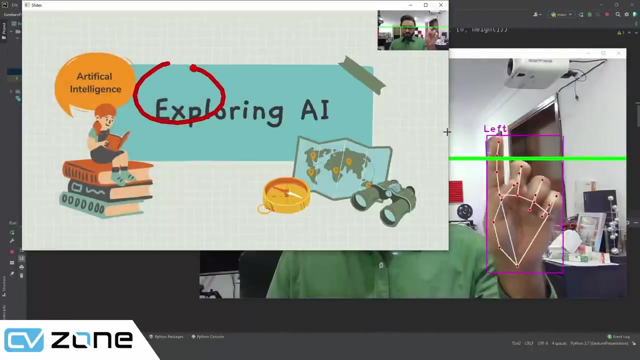 Yeah, maybe that's the problem. Innotation start should not be in another if statement. It should be directly that: if this happens, then do it. Maybe that was the problem. Okay, let's try. Let's try it out. So circle, circle, circle, circle. 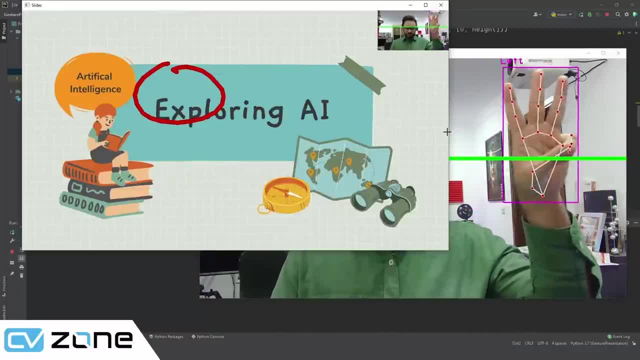 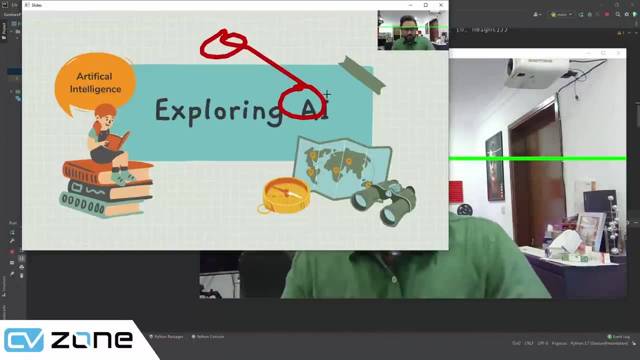 Seems fine right now. Didn't happen, Let's try it another time. Oh, it happened again. To be honest, I'm not sure why this is happening. So it's going from here till here. It means that the, The index number, is not updating properly. 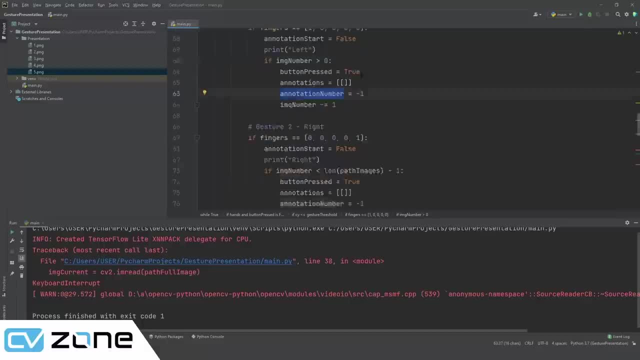 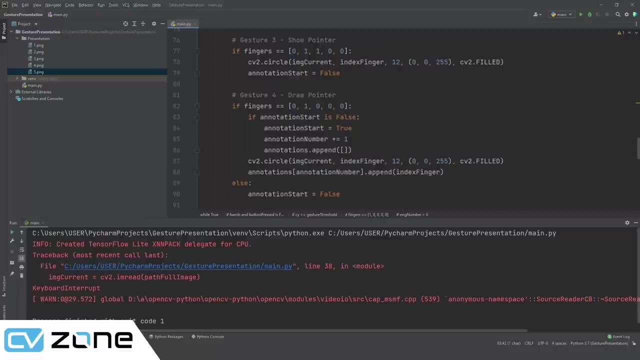 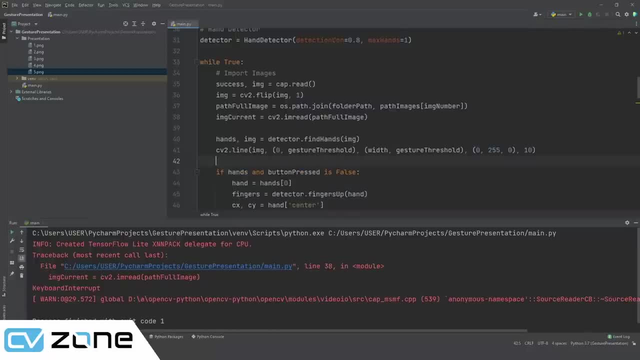 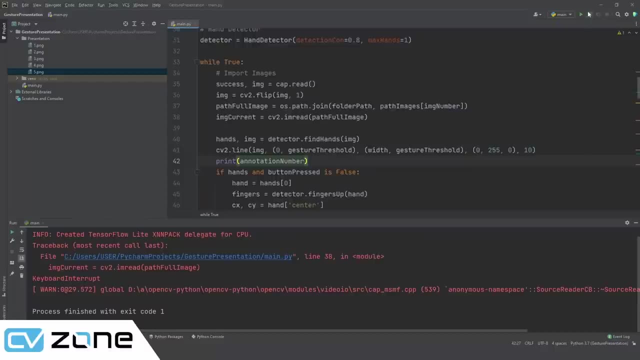 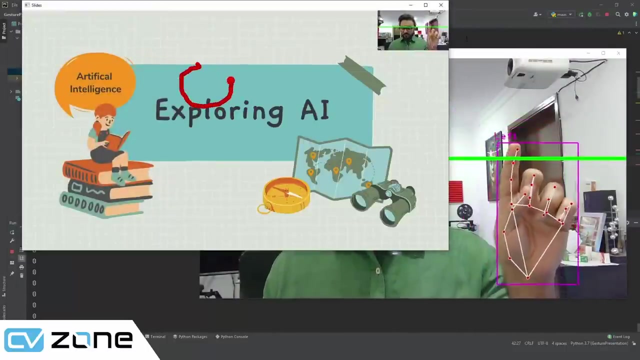 Let's try to bring it into. OK, let's try to bring it into. try to print the annotation number. let's see if we can find something there. so it is minus one right now. we drew and it became zero. now we draw again it. 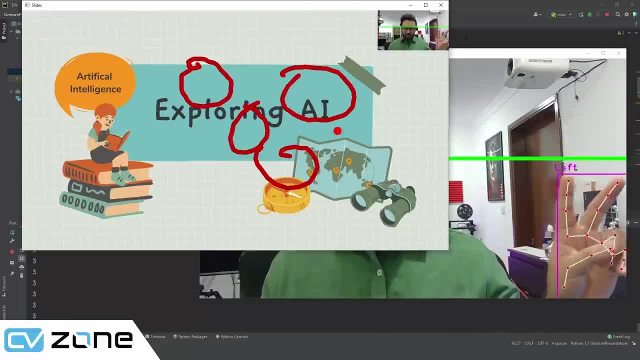 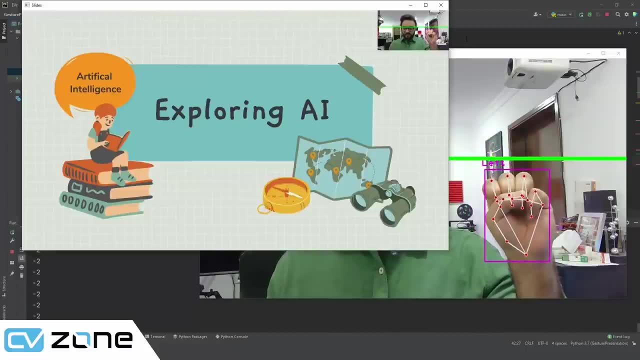 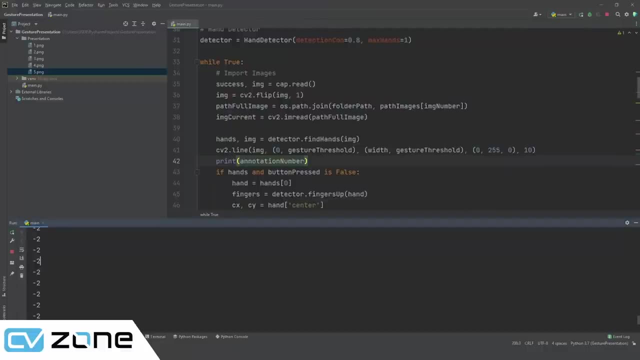 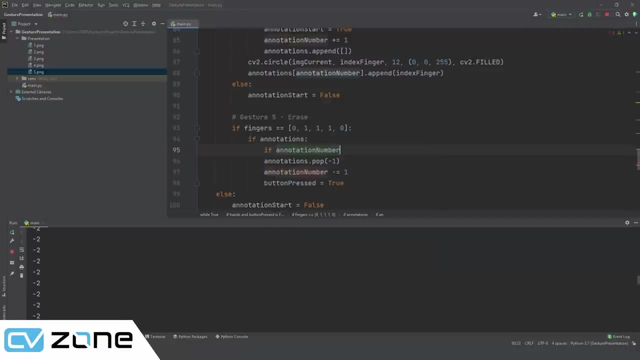 becomes one, draw again becomes one. we delete, delete, delete, delete. this is the problem: it becomes minus two. why did it become minus two? so notation number. so whenever we are popping there is something, annotation, if annotations, if annotation number is greater than minus one, then only you can. 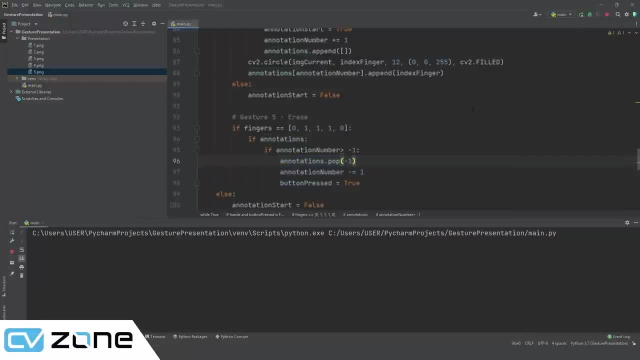 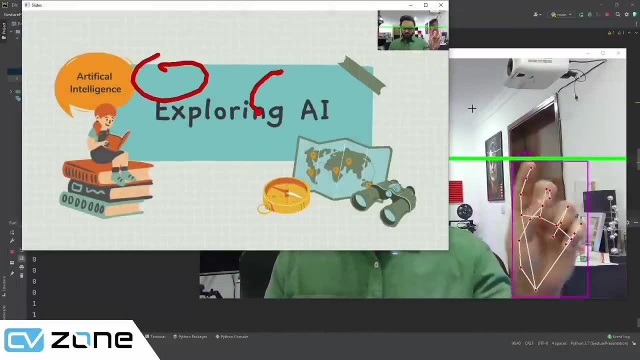 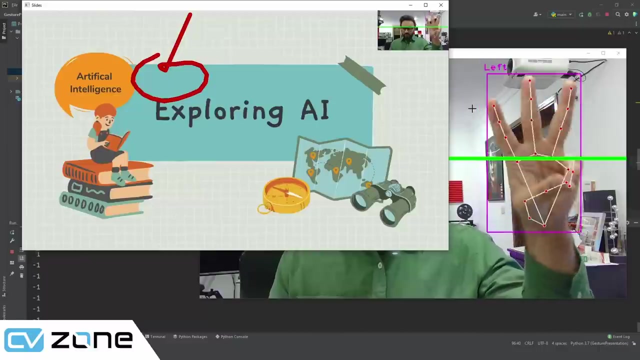 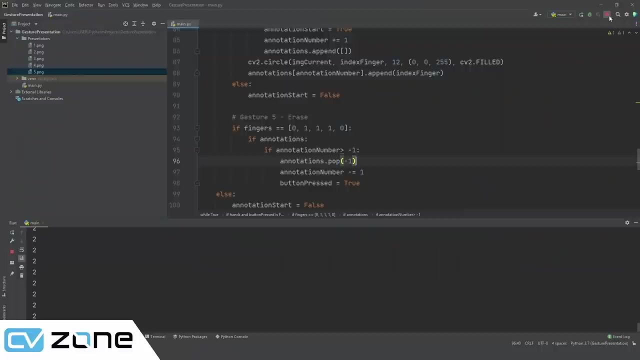 do this. let's try that again. so draw, draw, draw, delete, delete, delete, delete. you cannot delete more, so it has another one, but it's not able to delete. so this is minus one, so now it becomes zero. so yeah, this is the issue. so the annotation number is not correct. 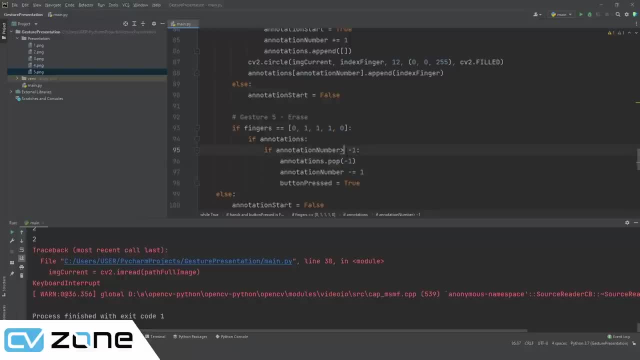 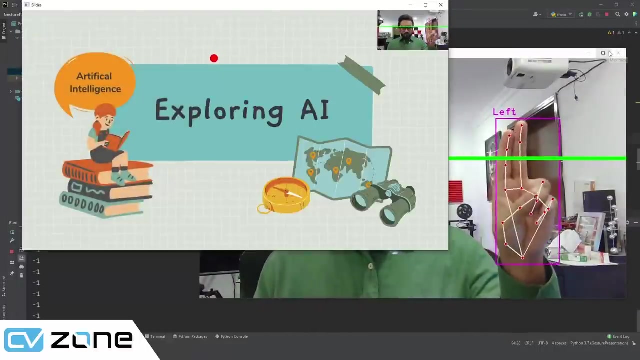 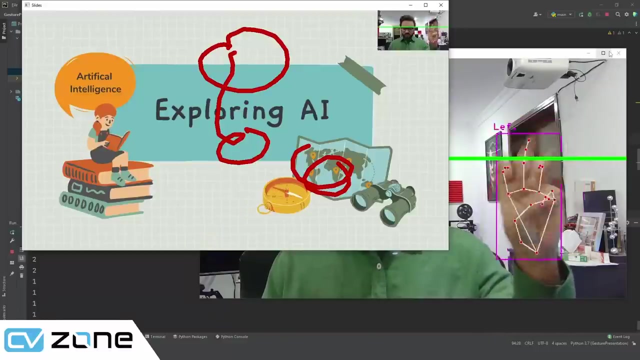 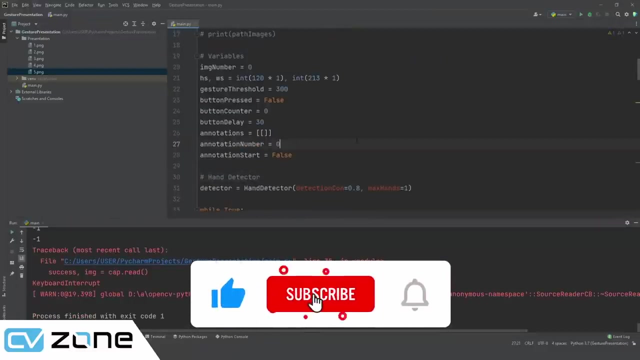 greater than or equals to zero should be the same thing. try that out. so this is the first one. second one, third one: delete, delete, delete. so yeah, we are not able to delete the last one. so why is that? okay, let's try to put this as zero. 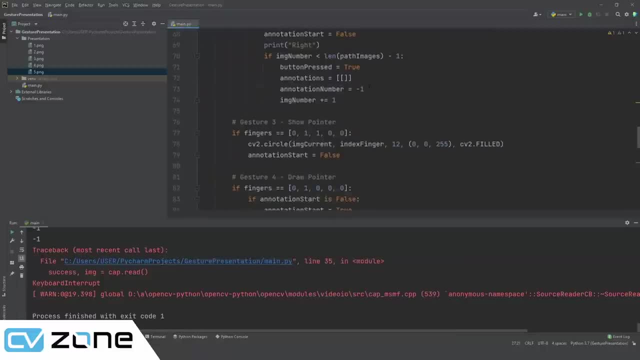 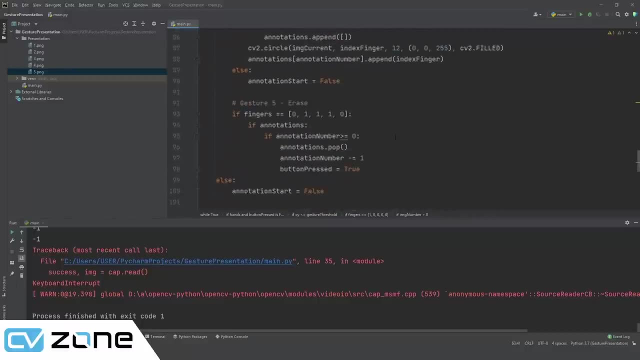 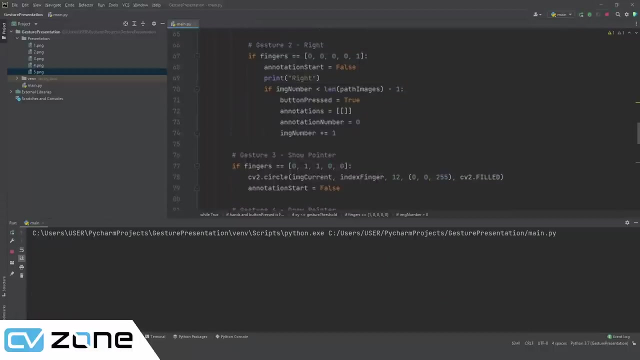 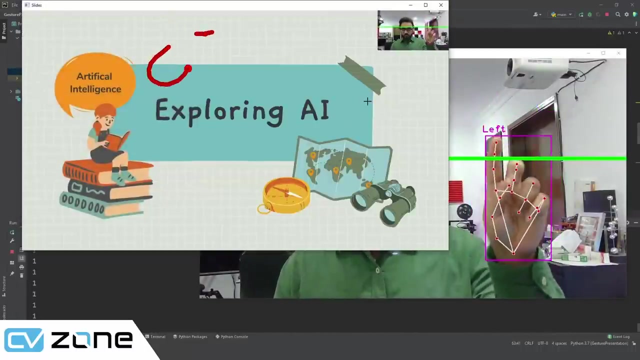 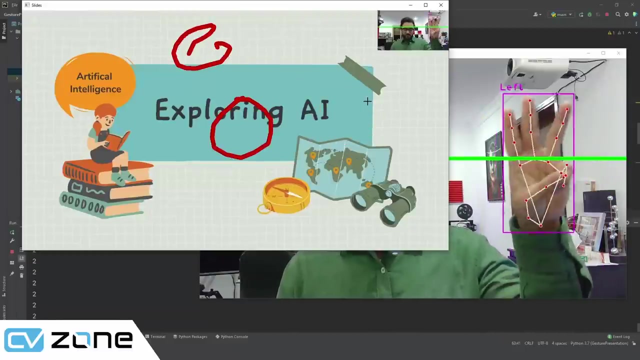 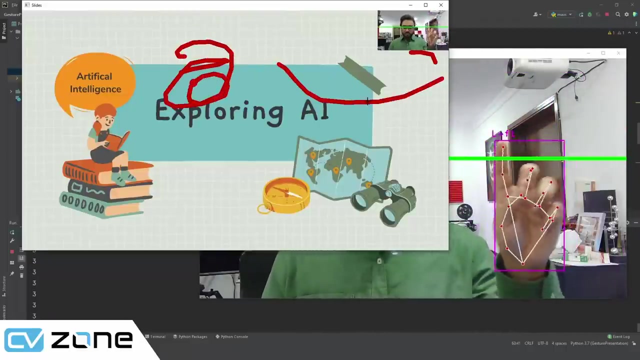 and then we will put this zero, well, and this zero as well. is there any place, I don't know. so let's try that. so this is one, two, three. one, two, three, four. yeah, now it seems fine. one, two, three. so there you go. so hopefully, this is the problem. 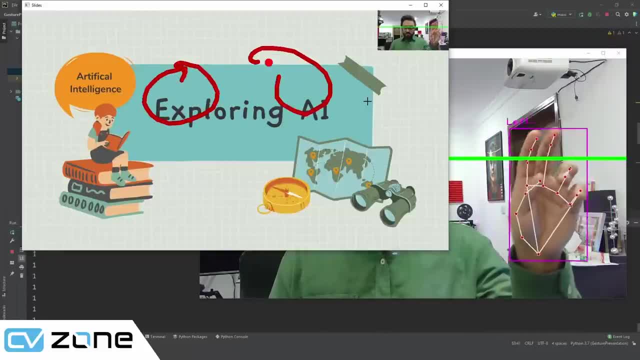 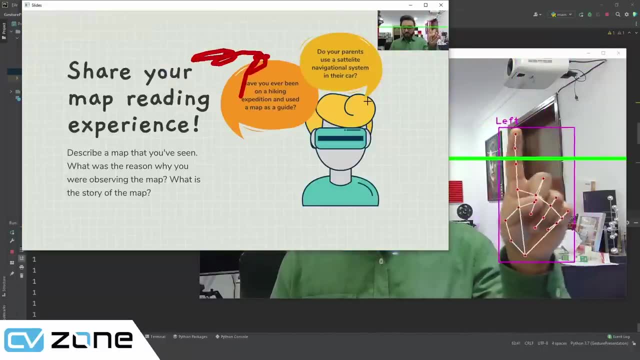 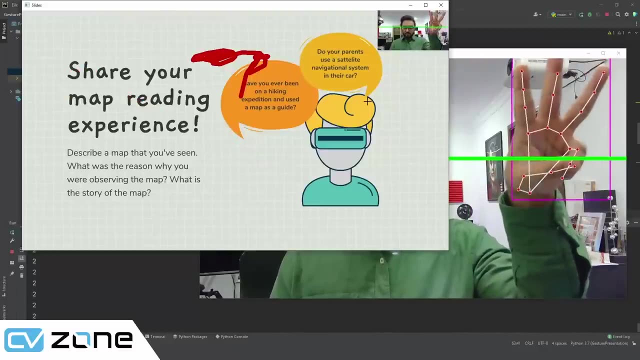 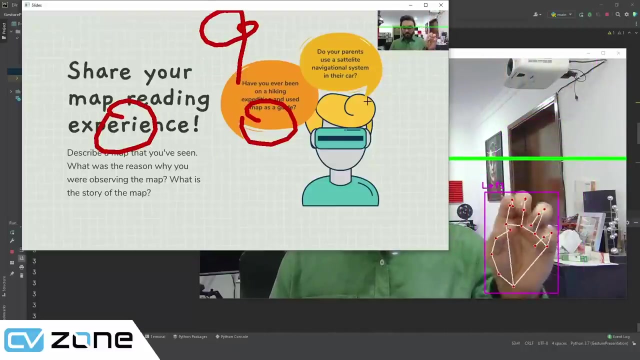 so now I can see the problem is solved, so hopefully this will not create any more problems. so let's see this. there you go. we are able to do them separately: one, two, three and four. we are able to rub off all of them and we are able to create without any lines in between. 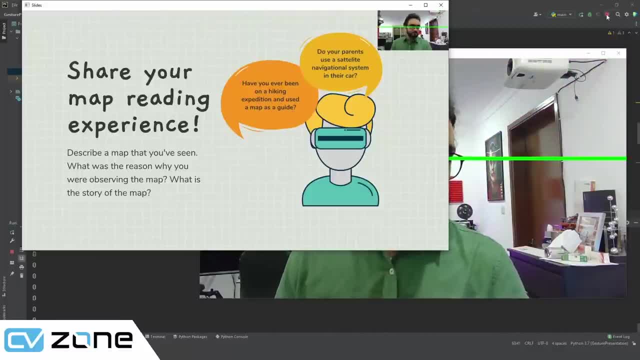 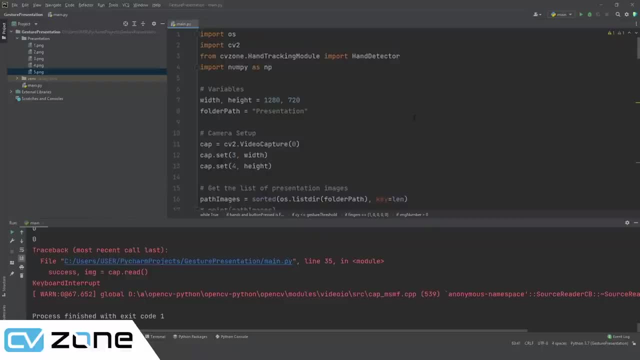 so this was the issue. so this is it for today's video. i hope you have learned something new. this is a very good project if you want to actually present and it can be used in real life. so you can take this and present with your own presentation. all you have to do is change the files over here and, if you wanted to,